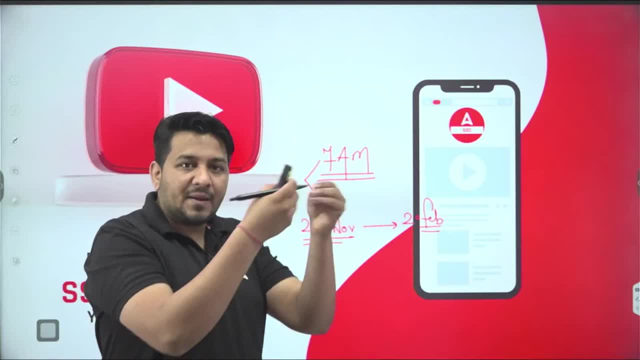 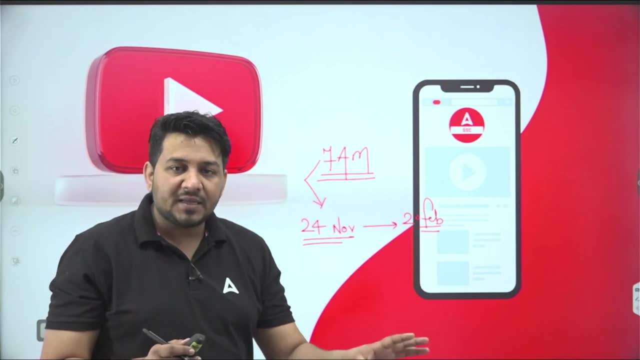 For always you said: it is your wish to study further. It is your wish to study further or not to study further, But at least till the 20th of February you will be so ready That you will have at least one job. 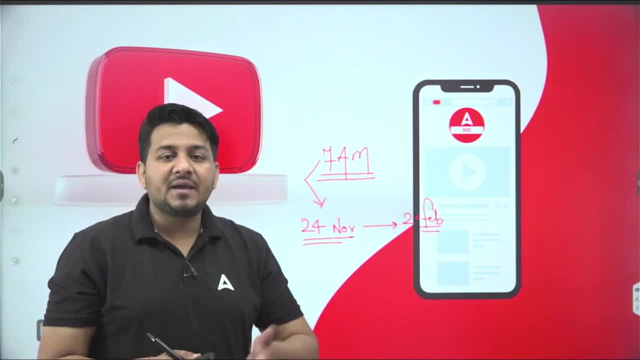 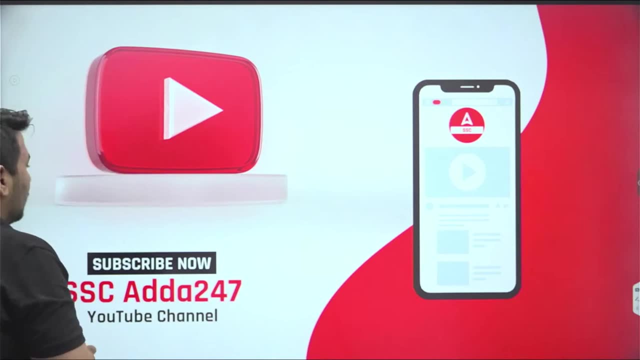 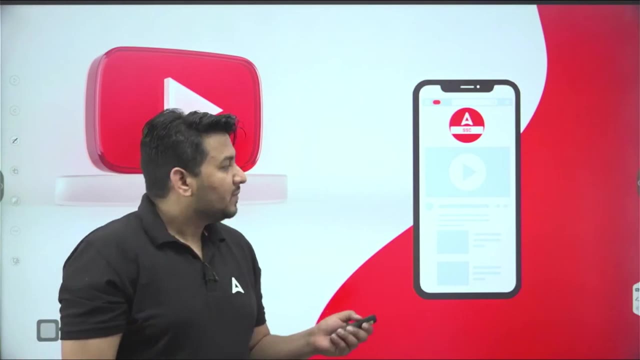 After that, pursuing further will depend on your wish. So all students quickly like and share the session and start the class And all students come with me live at 7 o'clock. Let's move ahead with a small information. See all of you see the link of the app on the blue strip. 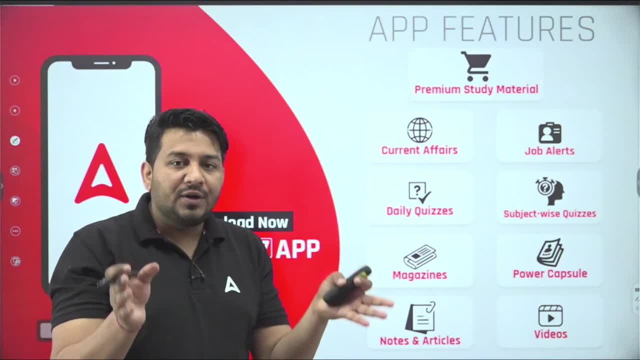 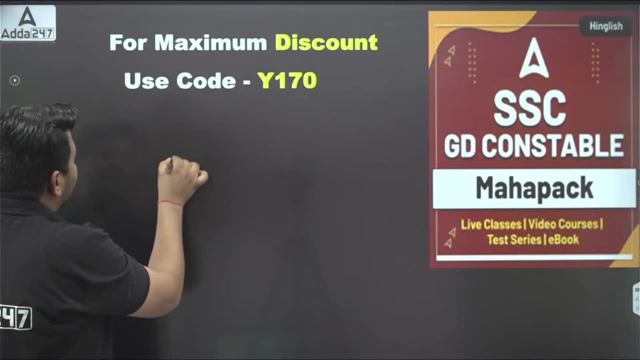 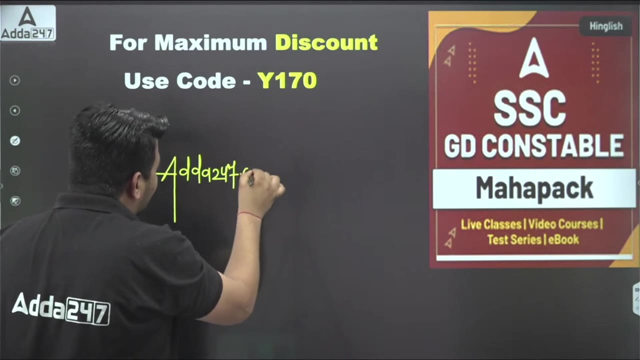 Click on that link and download the app. Then you will get the notifications of the video. Come on, Let's start the class with a small information. This is our GD Mahapack. See, you know, the vacancy has come. GD Mahapack will be your best friend at this time. 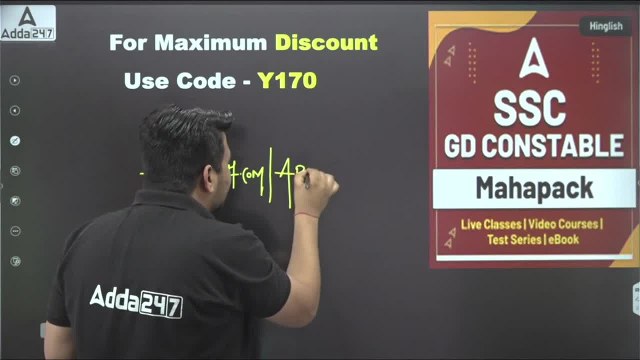 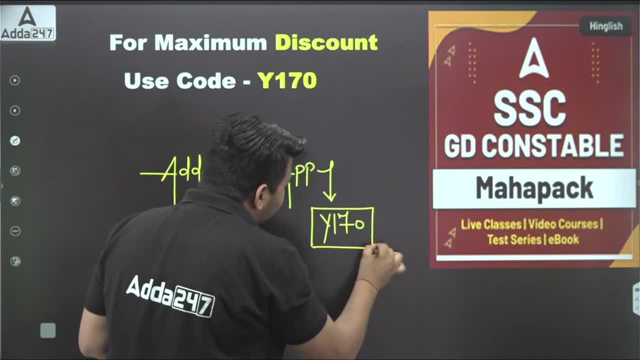 So if you have GD Mahapack, then it is not a good thing. So quickly visit atat247.com or the app, Enroll in it with Y170 code. So put this coupon code, Then you will get the maximum discount. 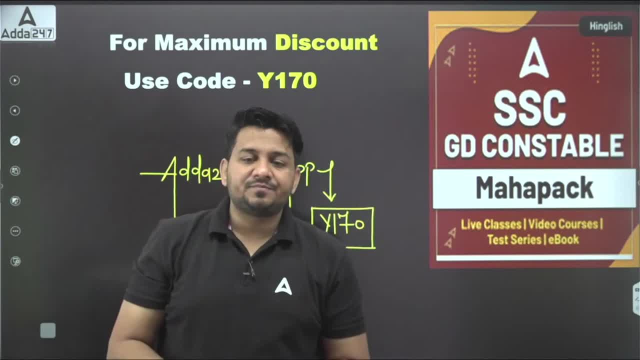 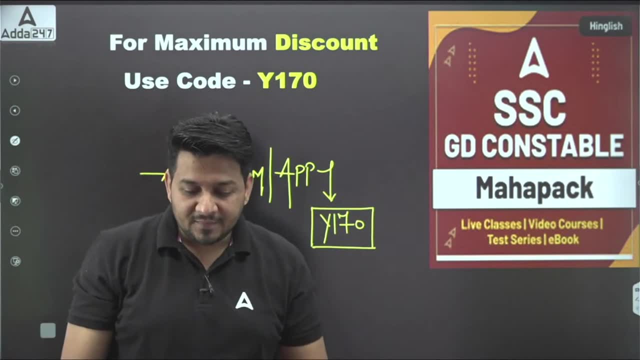 Come on, Let's start. Write in the comment: Yes, sir, ready. Quickly write in the comment: Yes, sir ready, Start, Let's start. Let's start. Bring the first question. Are you all ready? Ram Ram. 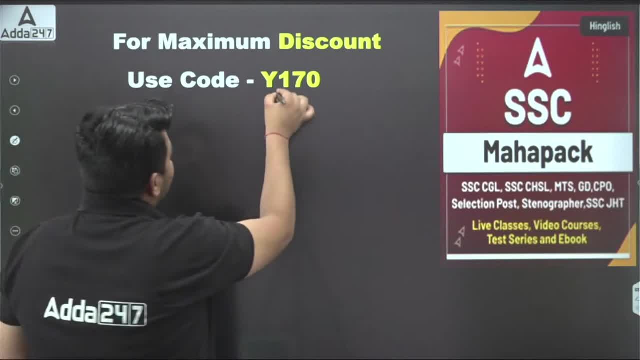 Come on. And if you want to cover all SSC exams together- CGL, CHSL, for all of them- then you can go to SSC Mahapack with our Y170 code. All SSC exams are covered in it. The process of joining is the same. 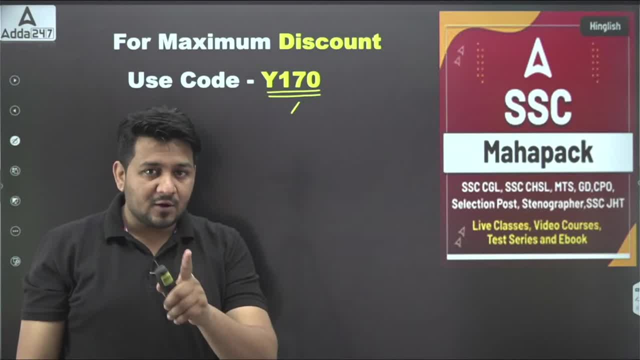 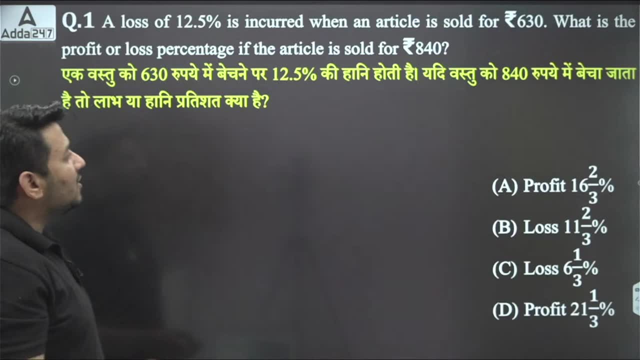 Come on. So, brother, I am bringing the first question in front of you. Make notes, Understand each thing very carefully. Come on, The first question is in front of you. All the questions are of GD, Previous year. The first question is in front of you. 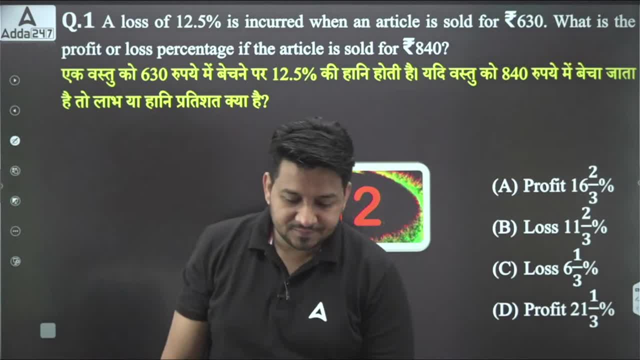 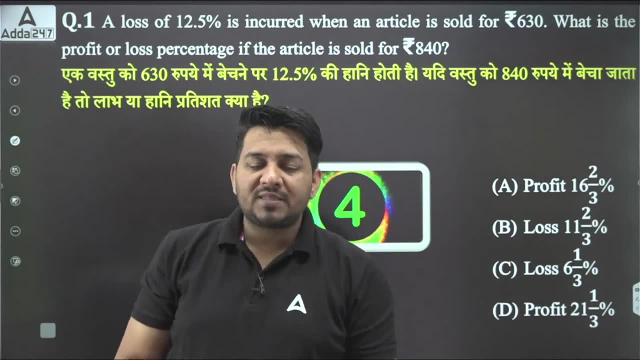 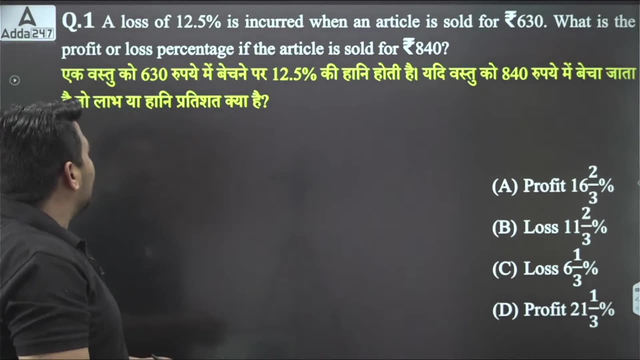 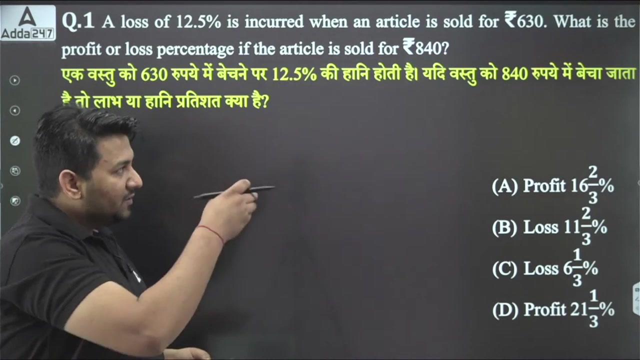 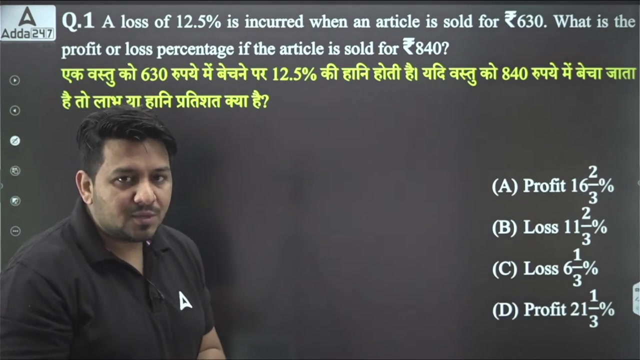 The time limit is your start, Tell me. The first question is in front of you. I will teach both son. Saturday Saturday: Saturday Saturday St. How will we know that if we sell it in 840, there is a profit or loss when we know the cost of the article? if the cost is less than 840, then there will be a profit. if there is a higher cost then there will be a loss. so basically, first we will take out the cost from here. how see? very carefully, you know that selling in 630 rupees is a 12.5% loss. what does 12.5% mean? 12.5% means one share. 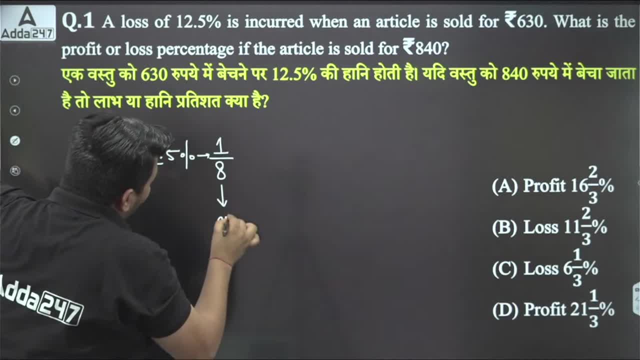 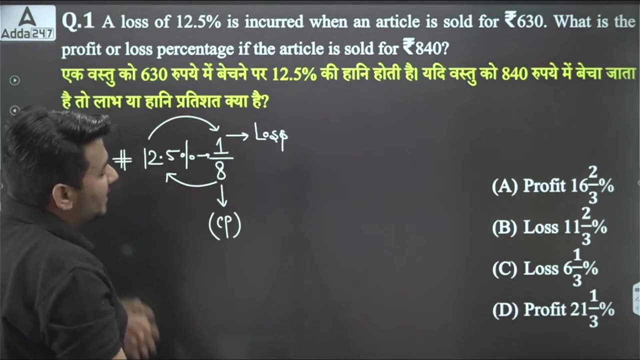 This 8 unit is called cost. 8 unit is cost if I take out 12.5% of 8,. if I take out 12.5% of 8, then there will be a loss of 1 unit. think that 8 rupees is a loss of 1 rupee. see, 8 rupees is the cost and 1 rupee is the loss. 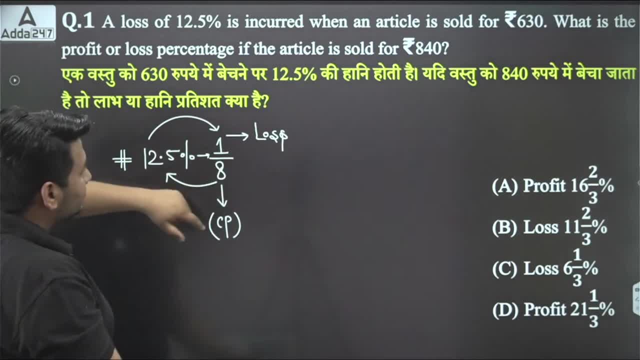 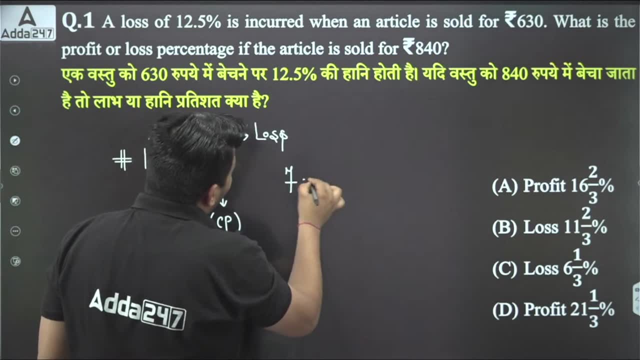 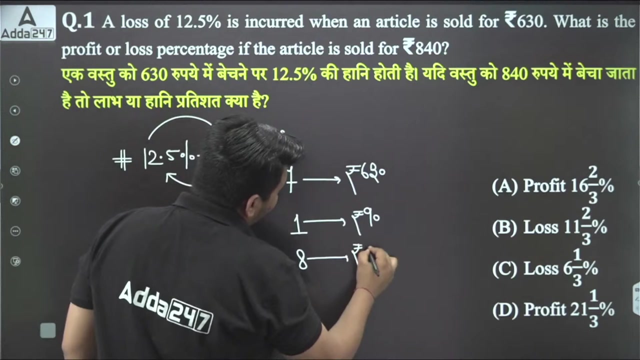 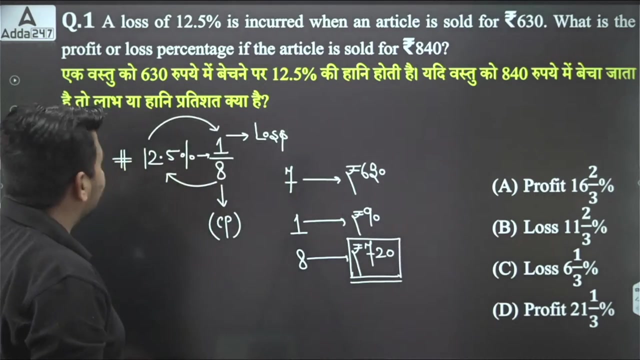 if we sell it in 8 rupees, see 12.5% is a loss of 1 rupee. if we sell it in 7 rupees, see 12.5% is a loss. how much would be the value of 7 units? 630 rupees, so how much would be the value of 1 unit? let's say 793 rupees, so how much would be the cost of 8 units? 8 names: 72, 720 rupees. costs are 720 rupees. that is the cost of price. 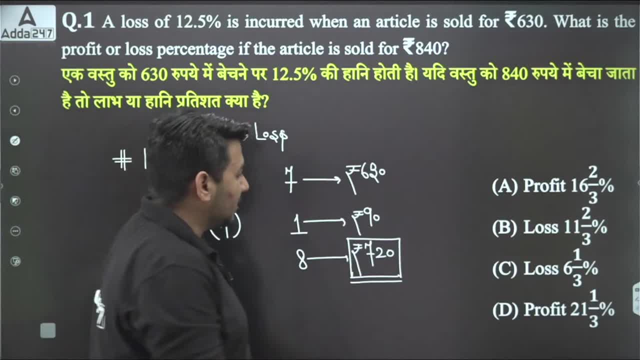 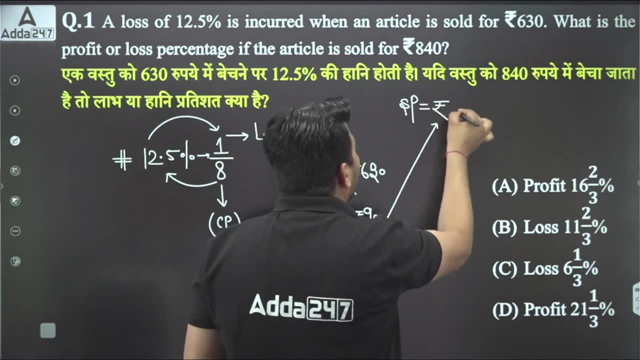 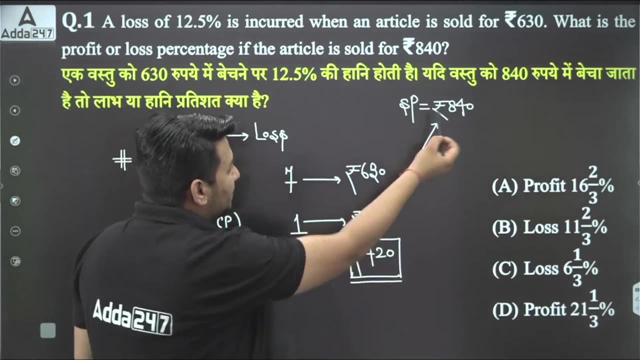 Ok, now if we sell it in 840 rupees, see how will we sell it. How much is the selling price 840 rupees? How much is the profit If you sell something for 720 rupees for 840 rupees? 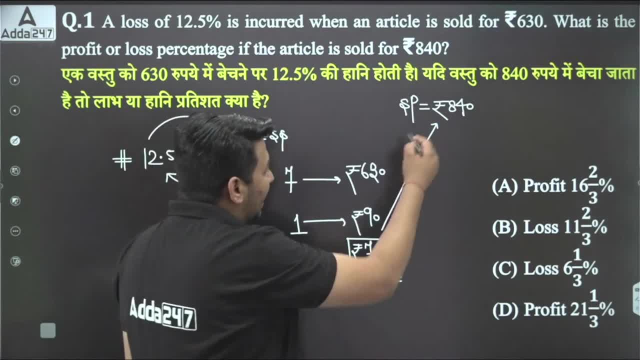 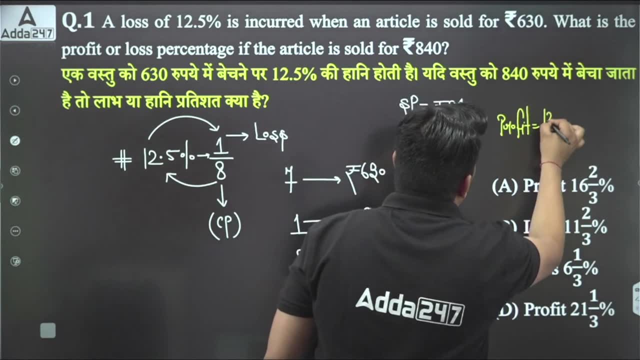 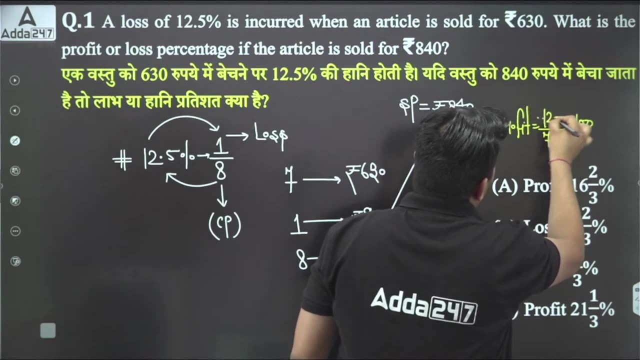 How much is the profit? How much is the profit? You will ask, sir, what is the profit of 120 rupees On 720? So tell me how much will be on 100?? So this one time and this one time, 6 times. 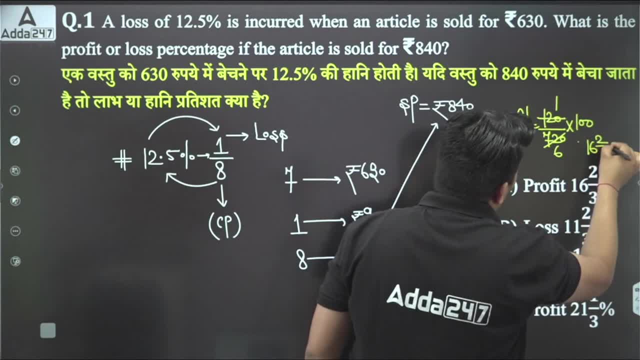 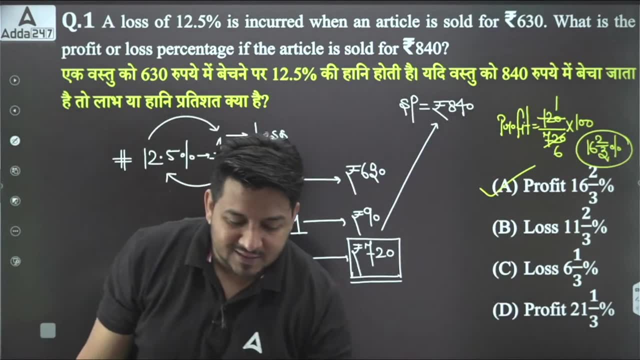 100 divided by 6 means 16 to 2 divided by 3 percent. You are getting profit of 16 to 2 divided by 3 percent. What is option number a? The correct answer is Tell me quickly that. yes, sir, clear. What is option number a? 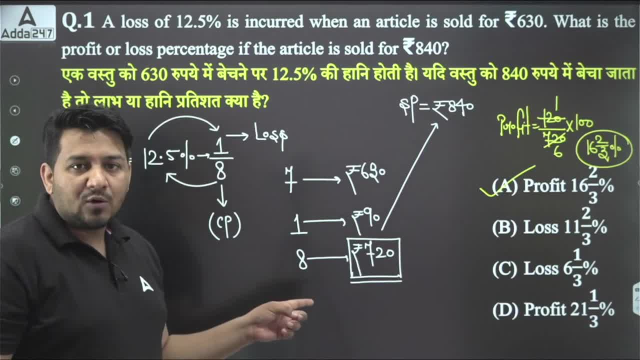 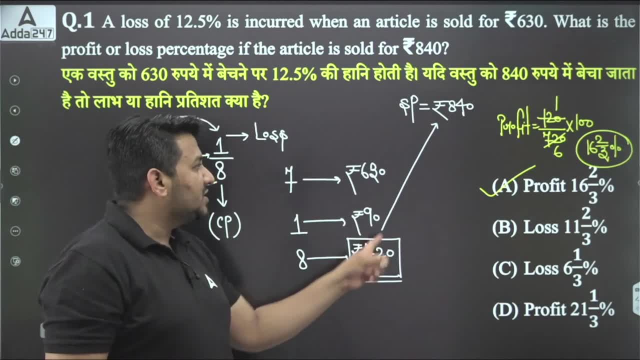 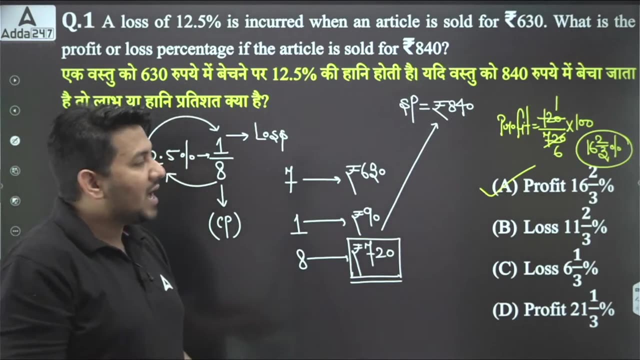 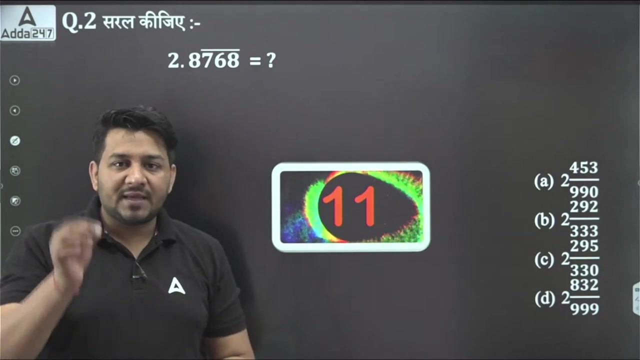 The correct answer is: Tell me clear or not clear On any step. First I took out the cost. when the cost came. then I saw that it is a thing of 720 rupees. it is selling at 840,. I took out the profit of 120 on 720, I took it out at 100, it became clear. let's move on to the next question. what is the next question? and let me tell you, there will be one question left from the decimal in the exam. 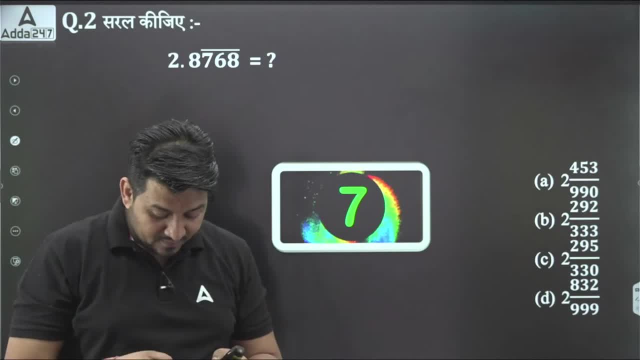 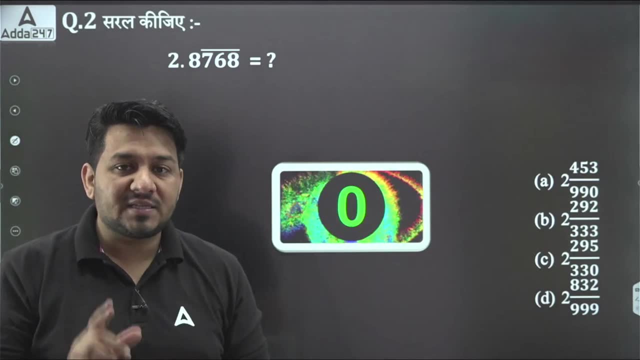 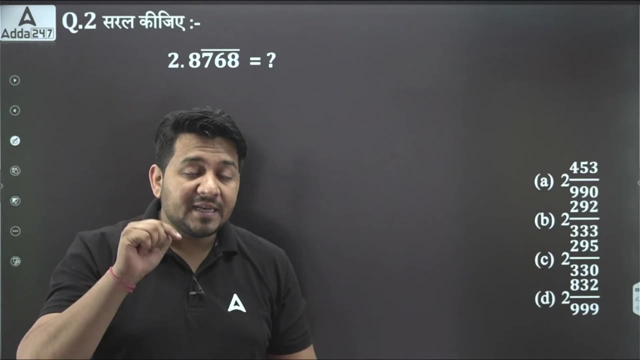 Sir, the vacancy is less. I just want to tell you one thing, son: how many vacancies came last year- 25,000, and at the end, how many vacancies had become 56,000,. how many vacancies had come 25,000, but at the end, how many vacancies had become 55,000, 56,000 vacancies had become. so, brother, the vacancy is not less, the vacancy will increase. you have to keep faith. 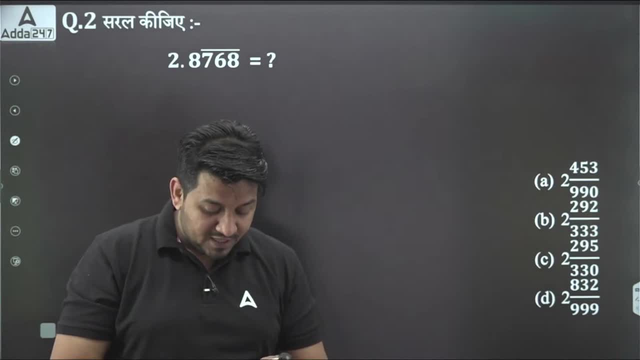 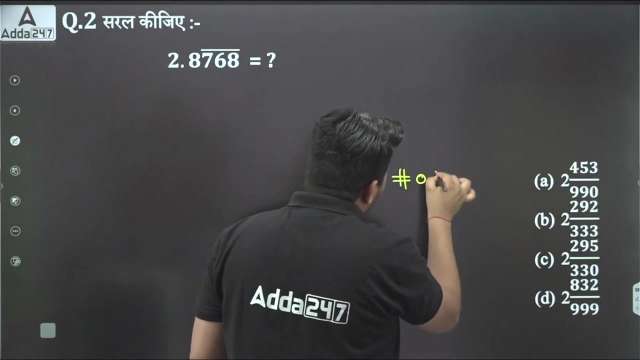 I am still telling you, If you are sitting in this hope that, sir, the vacancy is less, then the vacancy is not less, son, don't worry, the vacancy will come. now, look carefully, I am going to write my three points. write three points of decimal, the question of decimal in life, child. if it is wrong with you, then tell me. the first point is this child. note these three points on the front page of the copy: today 0.P. and if it is above P, then your direct result would be P upon 9,. 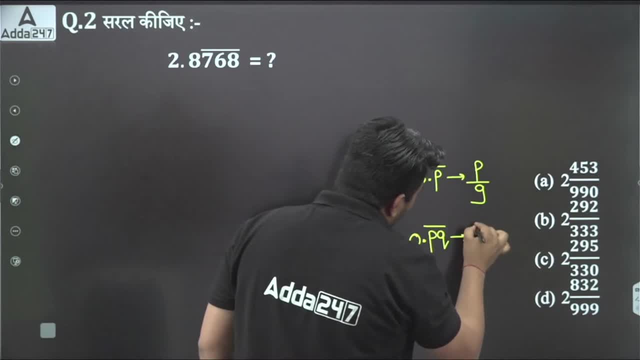 0.P. Q and above P and Q, then your direct result would be PQ upon 99,, that is double nine, 0.P. QR. is it PQR? okay, Q and R have over bar, but not above P. then you do what? take this PQR. 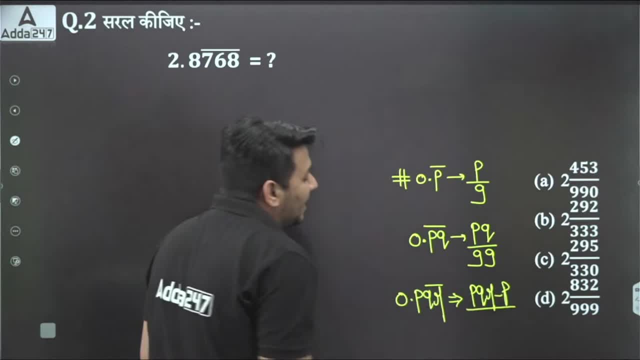 minus it P because it is not above P, and if there is a top bar of two numbers, then 2 times 9 and 1 times 0, this is the method of doing it: 2 times 9 and 1 times 0.. Clear Now see. apply your trick on this. 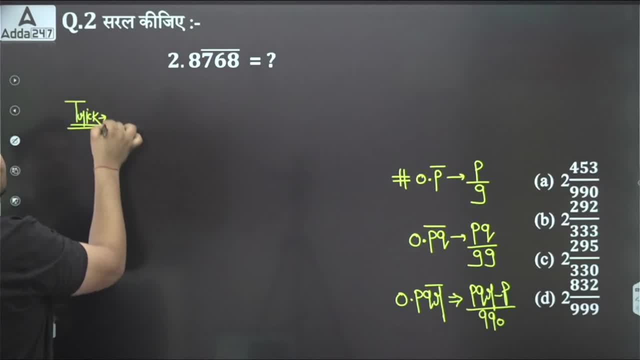 Write the value written before decimal as adjectives. For example, I wrote 2 as adjectives, 8,, 7,, 6, 8. Minus 8 because there is no bar above 8. There is a bar above 3 numbers 3 times 9 and 1 times 0.. 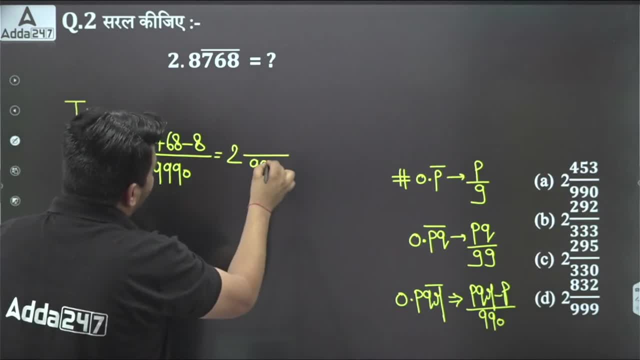 So this will be 2 upon 999 and above 8, 7, 6.. See 8 is 8 and 8 is 0. Cancel this. Cancel more. Yes, cancel 3 by 3.. 3 times 3 is 9.. 3 times 3 is 9.. 3 times 3 is 9.. 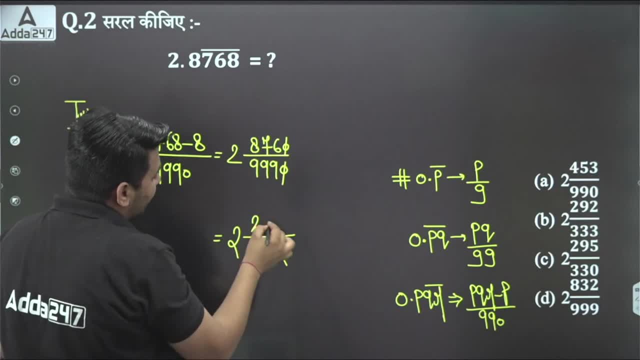 Cancel above. Cancel 3 by 3.. 3 times 3 is 6.. 2 is 27.. 3 times 9 is 27.. 3 times 3 is 6.. Is there any such option? Yes, there is. Which option? B option: 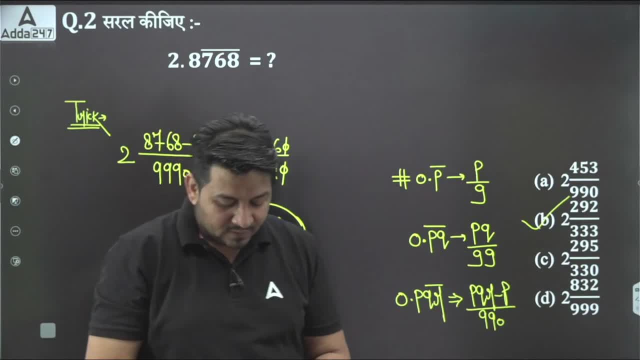 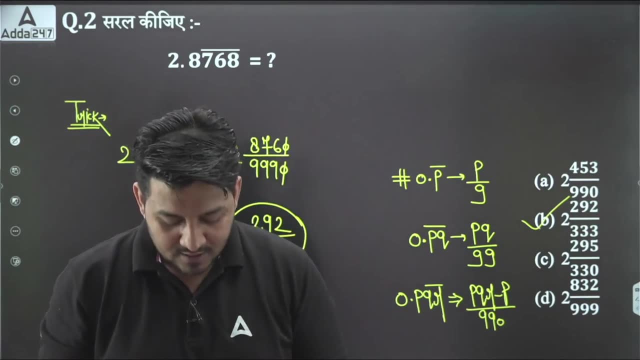 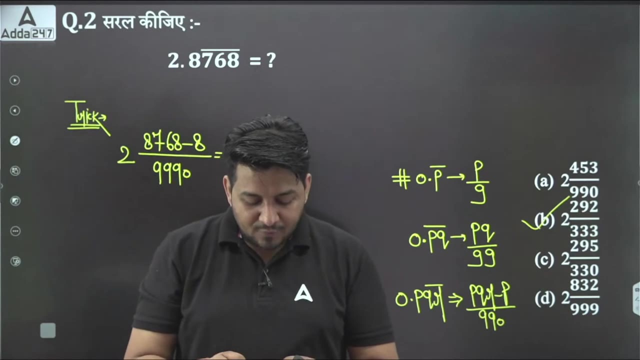 Which option, B option, Say clear or not clear? Tell me quickly: Yes, sir, clear. All students comment and tell me: Yes, sir, clear. Do you have any doubt on any step? If you have any doubt on any step, then you can ask us. 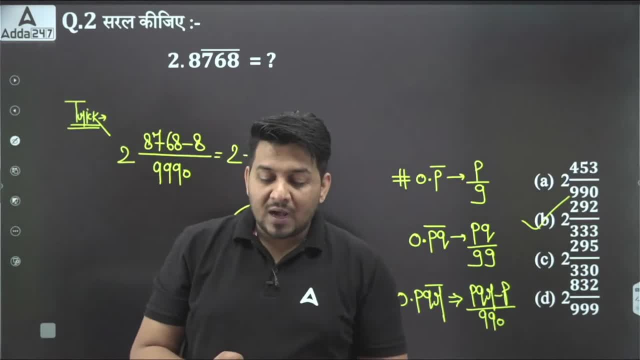 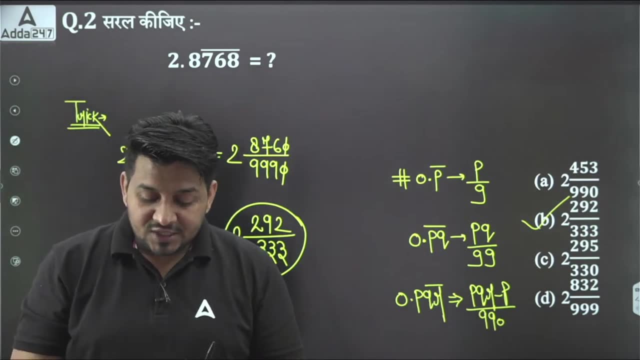 If you have any doubt on any step, then you can ask us And friends. no one has yet liked and shared the session. Like and share it quickly. Share it quickly on any Telegram, Facebook, WhatsApp, wherever you can share it. 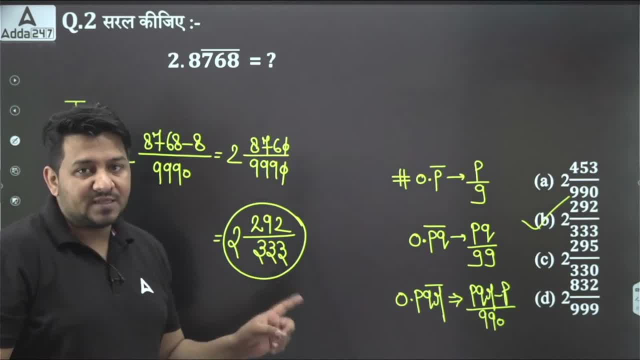 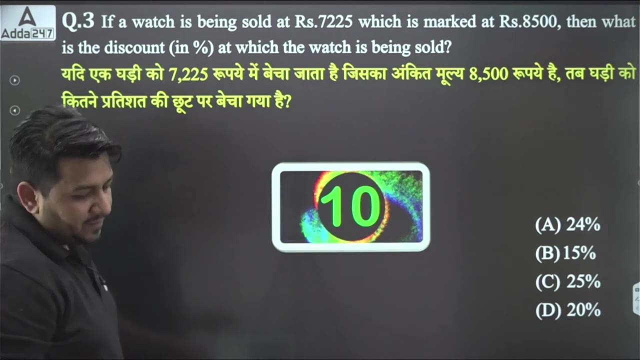 It is your responsibility to send these classes to all students today. There is only one thing that I will tell you today: It is your responsibility to share this class as much as possible today. Next question is in front of you. Tell me. There is a copy-paste question on January 10th. 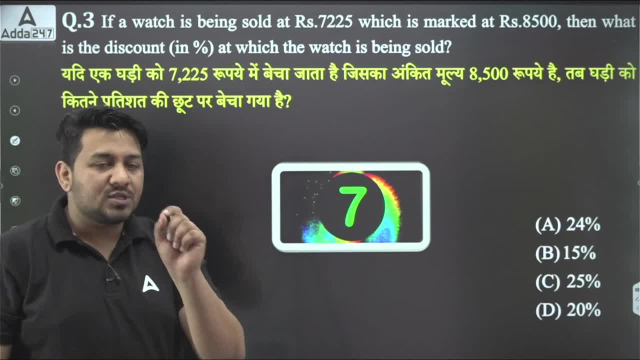 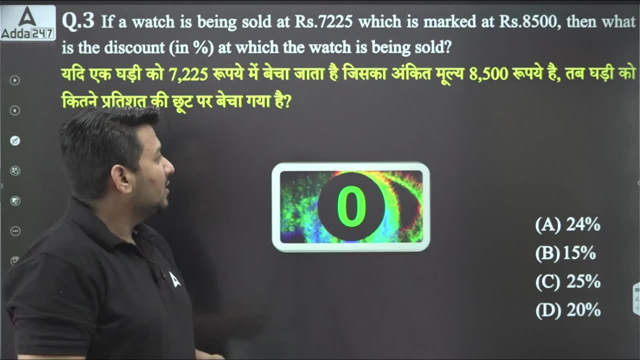 There is a copy-paste question. on January 10th The same data was asked in your GD. The same copy-paste of the paper on January 10th. What is the question saying? A watch is sold for Rs 7,225.. 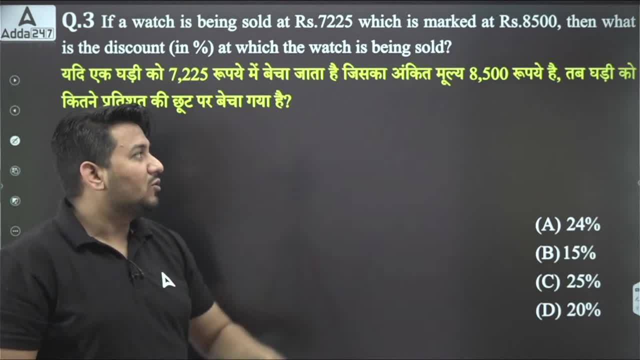 The estimated price of which is Rs 8,500.. So tell me what percentage of the watch is being given a discount. What percentage of the watch is being given a discount? How will you do it? Do you know what is the mark price? 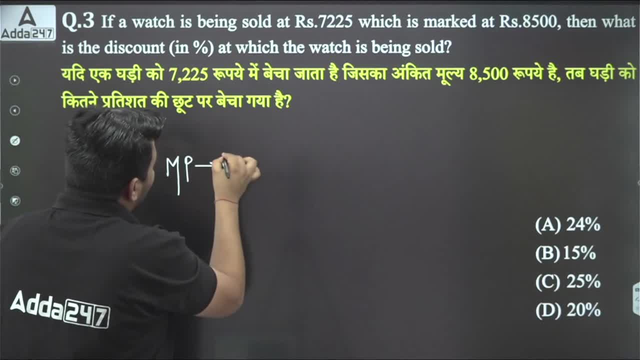 First tell me what is the mark price. Mark price is Rs 8,500.. What is the selling price? The selling price is Rs 7,225.. Now look carefully: Rs 8,500 is being sold for Rs 7,225.. 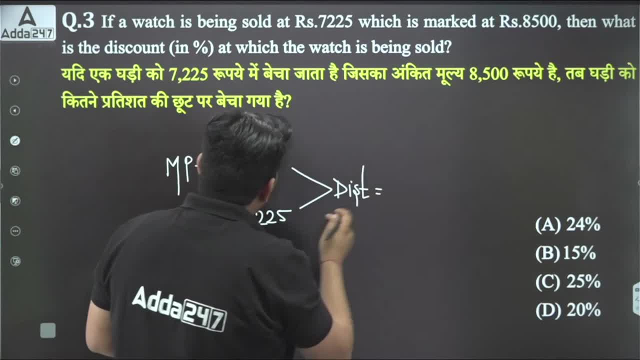 How much discount are you giving? How much discount? Look, 5 out of 10 is 5.. 2 out of 9 is 7.. How much is here? 2 out of 4 is 2.. The discount is Rs 1,275.. 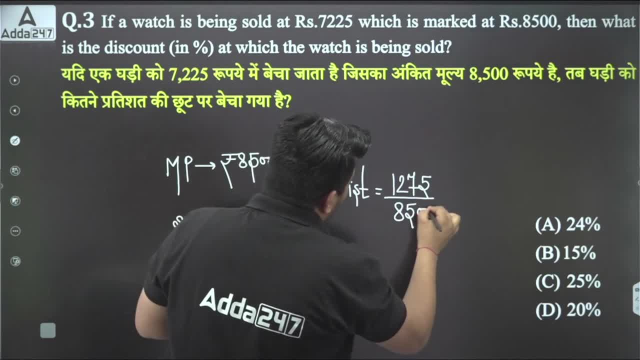 On how much? On Rs 8,500.. So tell me how much will it be on Rs 100?? Will you be able to calculate? Will you be able to calculate? Cancel these two zeros with this. Cancel it with 5, 17 times. 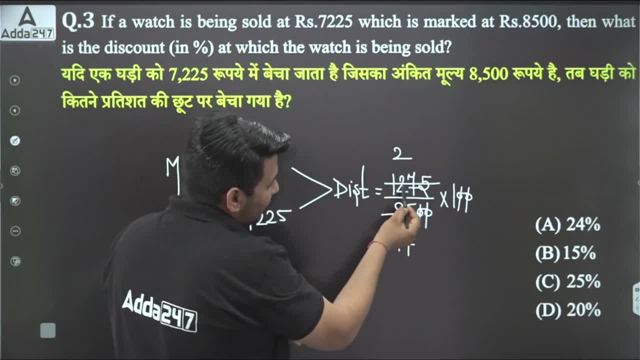 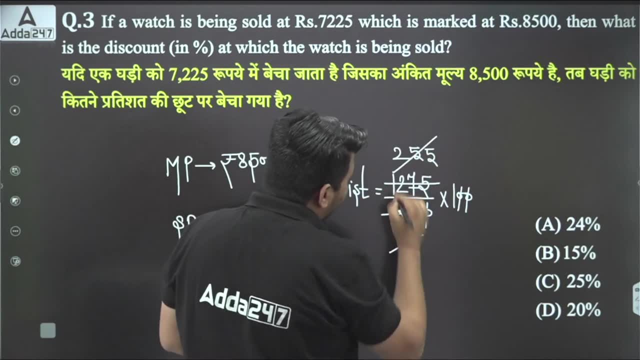 Cancel it with 5,, not 5, 10 times. 2 is left, 2 is 25.. 5 is 25.. 2 is left, 5 is 25.. Cancel it with 17.. How many times? 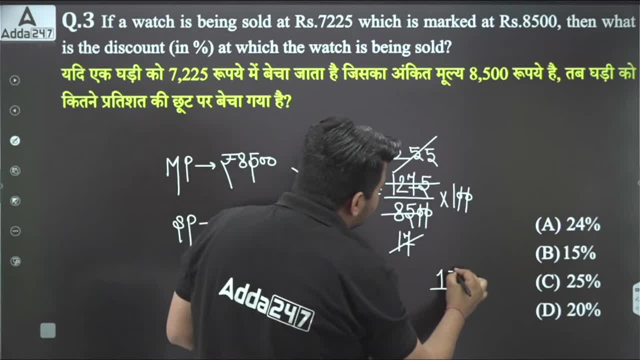 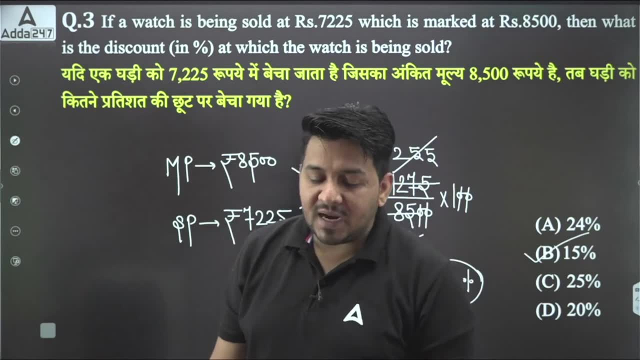 17 times 17.. 8 is left. 85 is left. 17 times 5 is 85.. That means 15% discount is being given to you. How much is the discount? 15% discount, Look carefully. 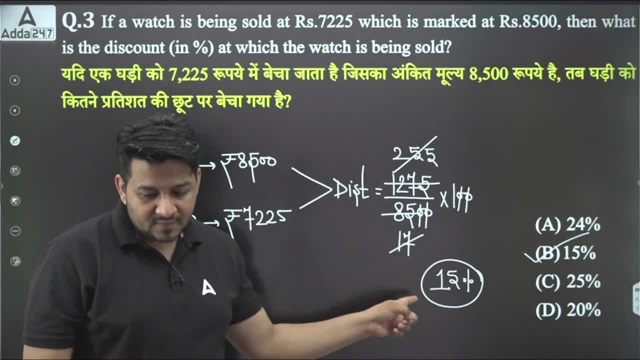 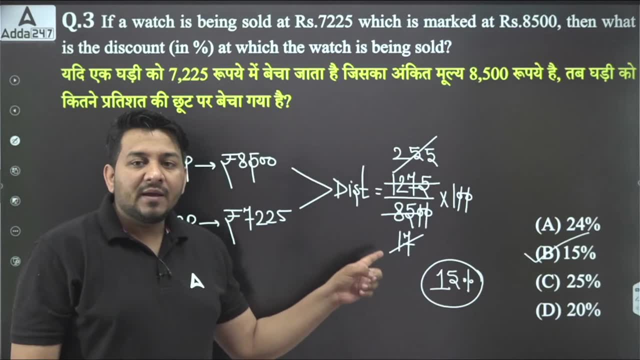 How much is the discount? 15% discount. Is it clear? All the children tell me. is the answer clear? Do you have any doubt? Do you have any doubt on any step, Yes or no? Did you enjoy it? It's good to drink coffee. 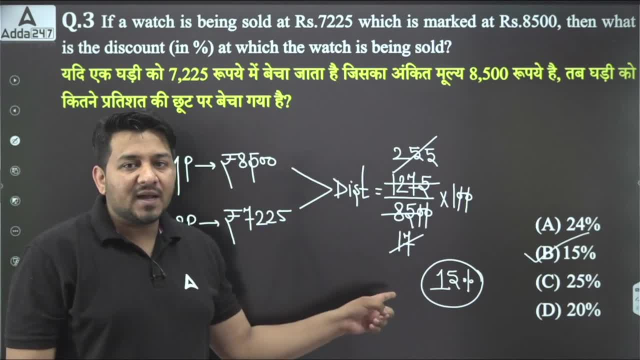 It's good to drink coffee, But let's make notes. It's okay to drink tea and coffee in the morning. It's okay, But let's make notes. Next question, Next question: children. Let me tell you This question came in the same format in GD. 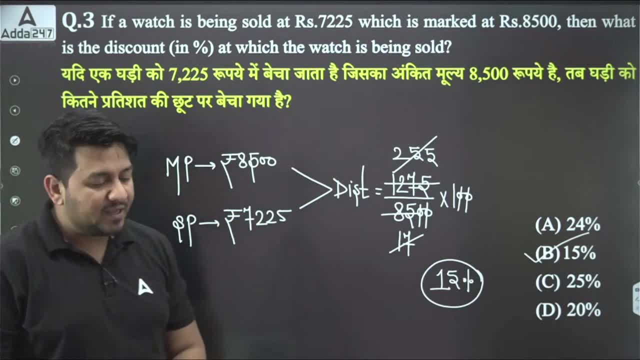 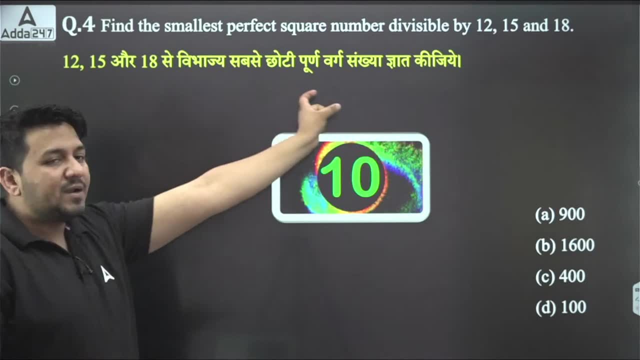 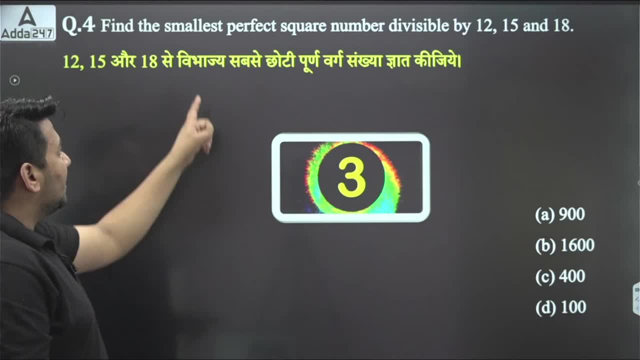 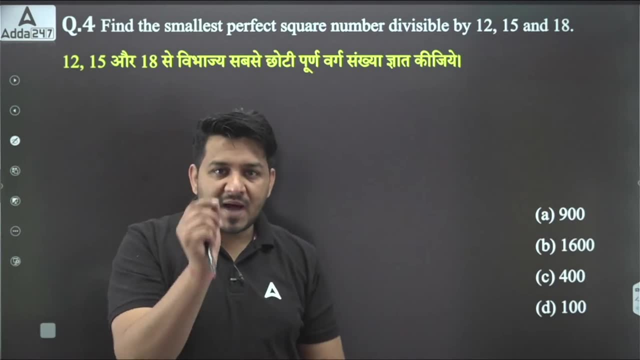 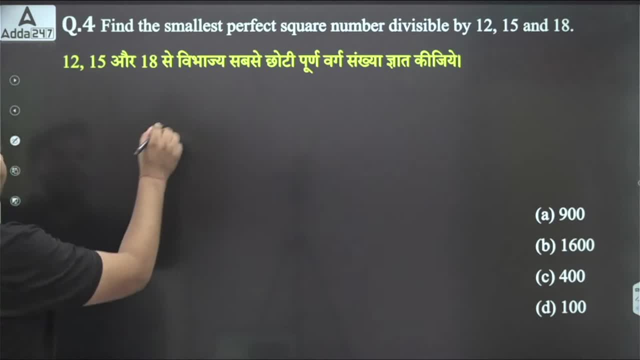 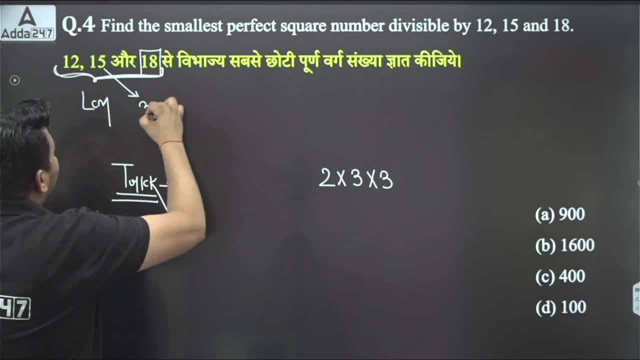 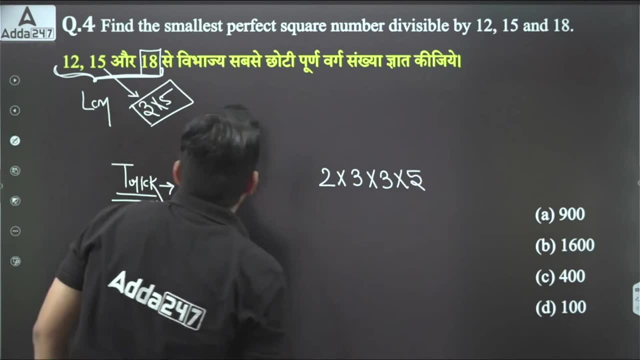 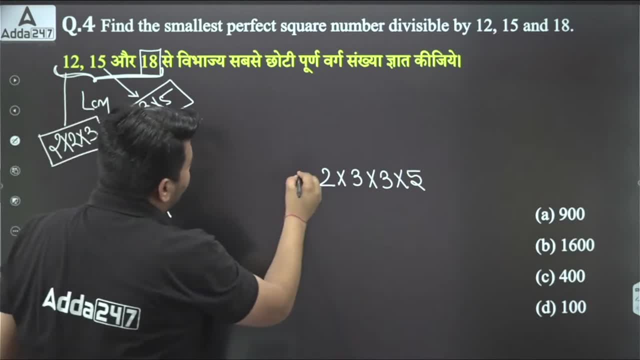 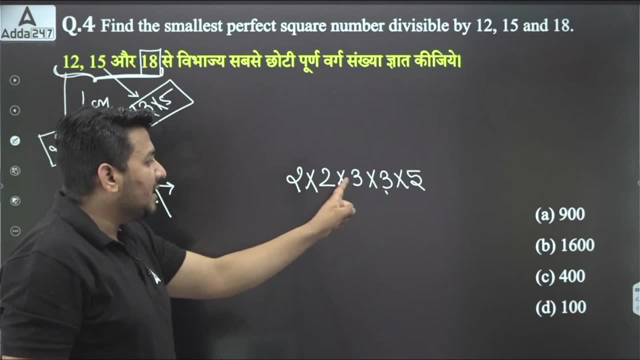 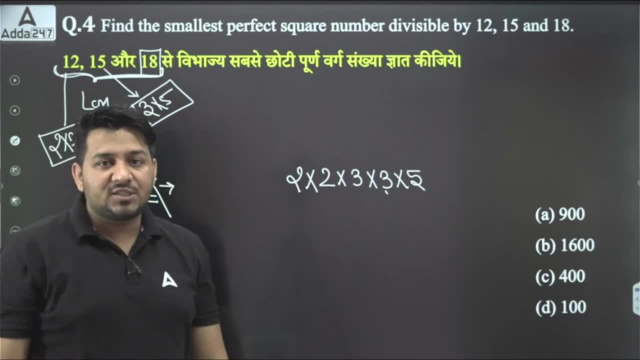 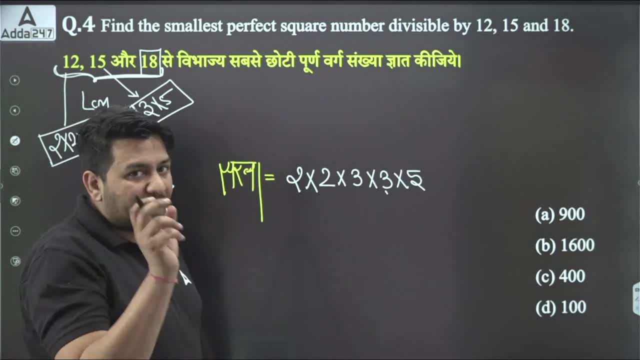 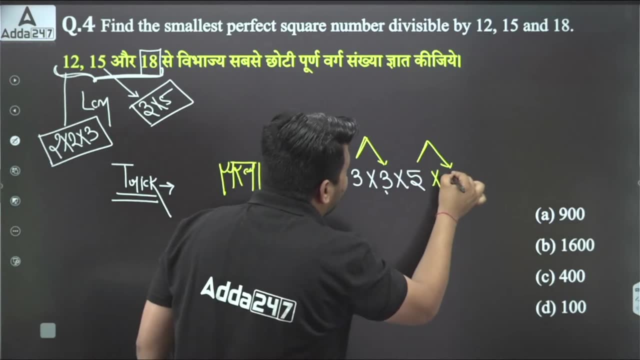 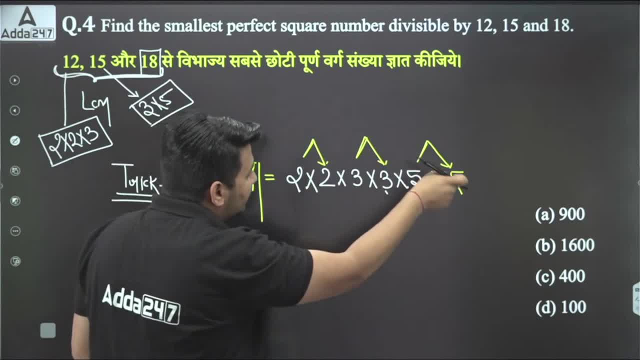 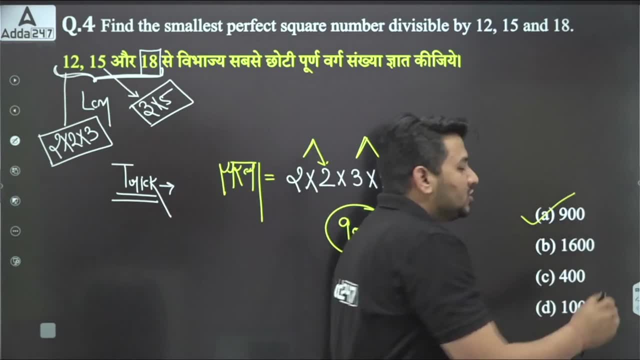 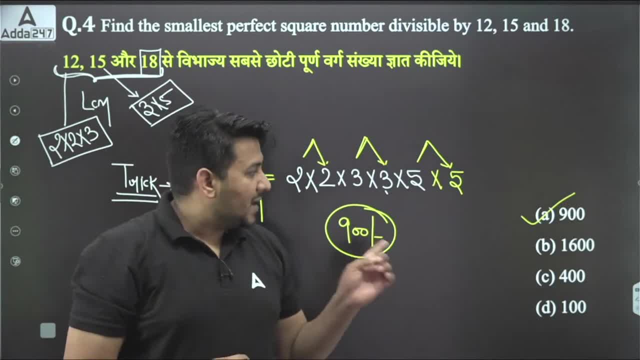 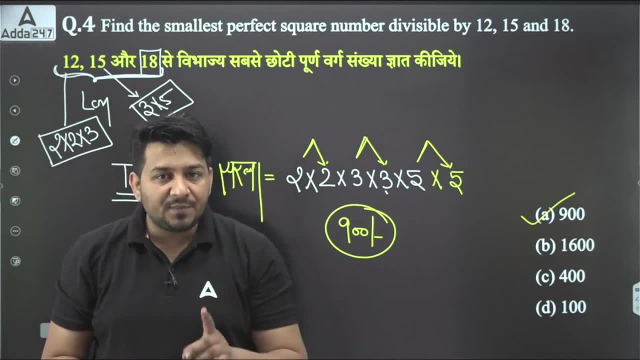 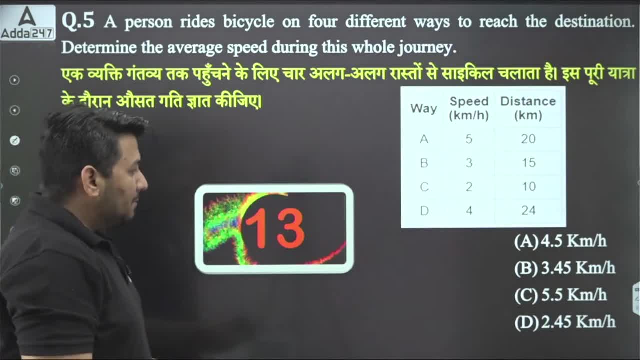 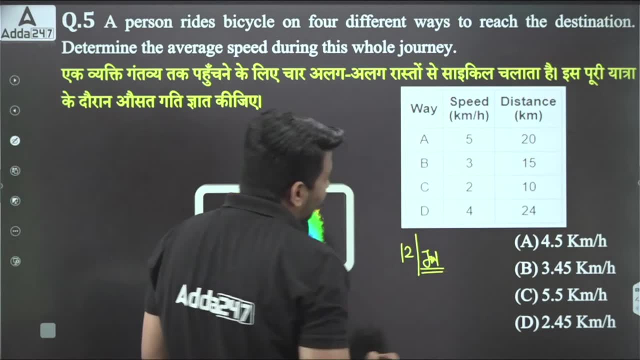 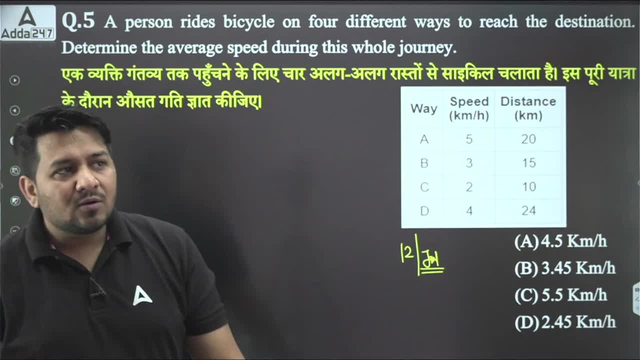 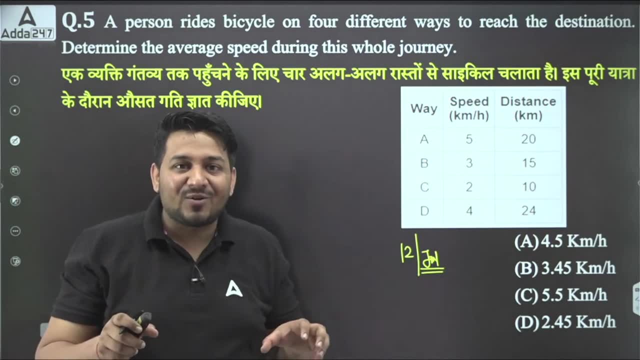 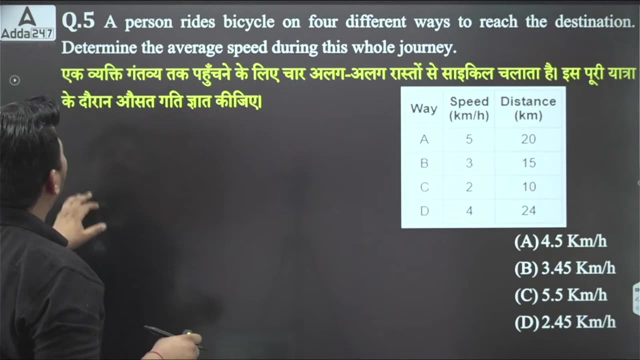 12., 12., 12., 12. 12.. He tries to scare his father. GD's paper tries to scare him. many times it doesn't happen. it's a very simple question. What is he saying to us? One person rides a cycle from four different ways to Gantab to reach Gantab. 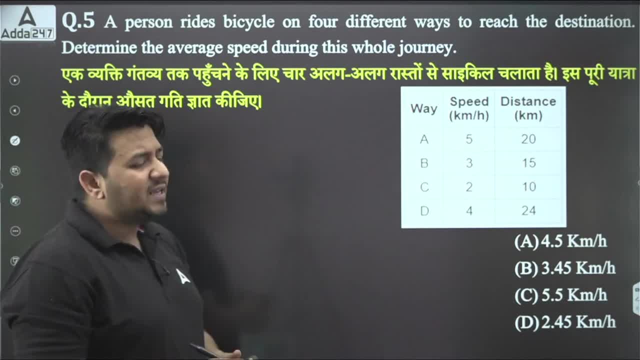 During the entire journey. learn the correct speed. It is the same question. don't be afraid of it. there is nothing in this question. Look: what is the average speed? What is the average speed? The average speed is equal to total distance upon total time. there is nothing in this question. 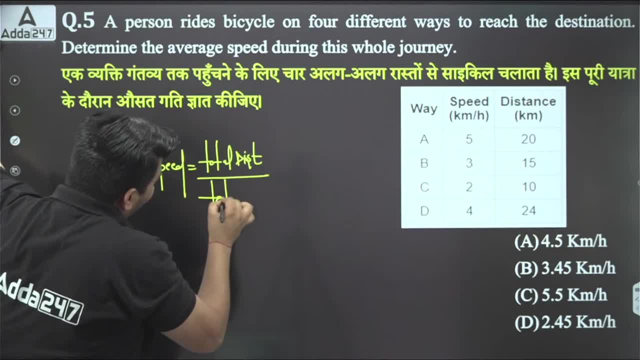 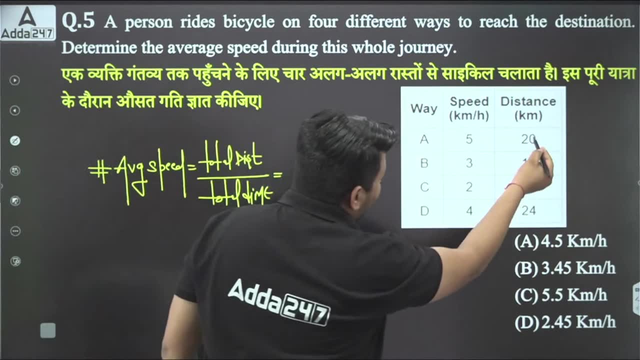 Total distance upon total time. I have taught you this Total time. What is the total distance? Add it: How much is 5 and 4? 9.. What is the total distance? 0, 5 and 4 is 9.. 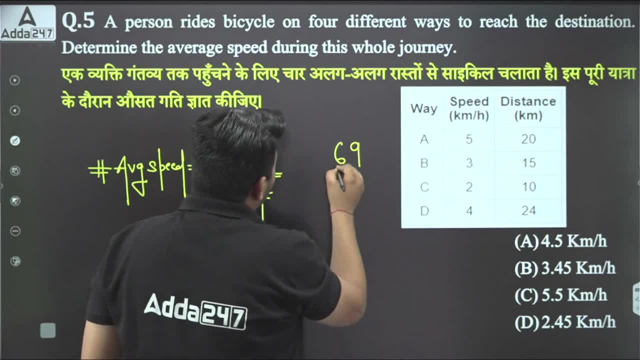 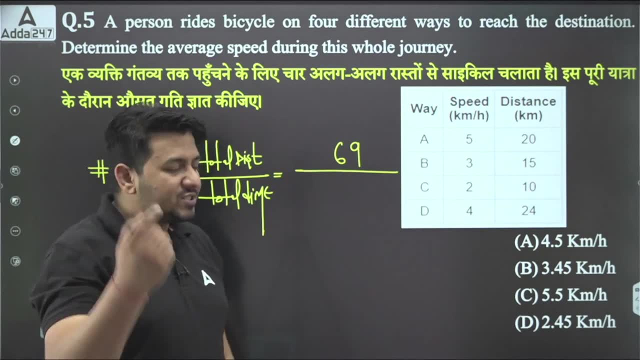 2 and 1 is 3,, 1 is 4 and 2 is 6.. In total, you have covered the distance of 69 kilometers. Now see how much time it takes. Look very carefully. There is a small thing here. 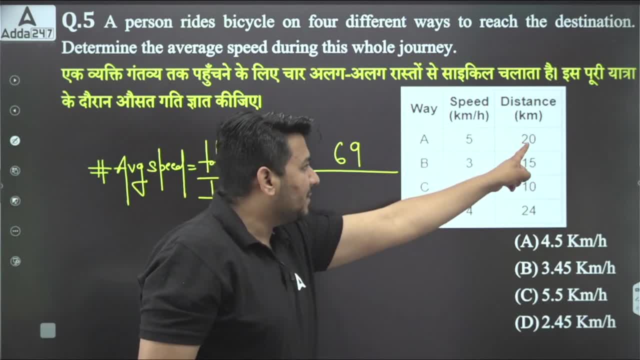 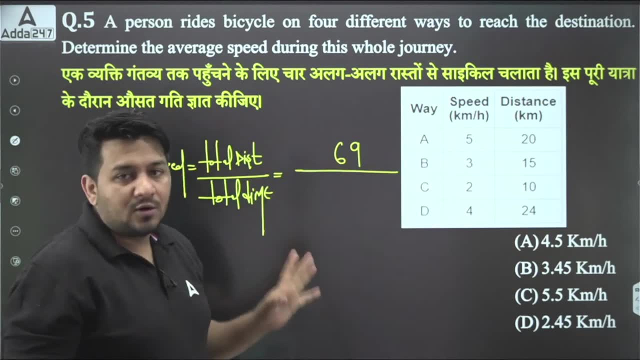 See: in total 20 plus see here 20 kilometers went. here 15 kilometers, here 20 kilometers, here 24 kilometers. In total 69 kilometers have been done. Now see, these 20 kilometers have gone. 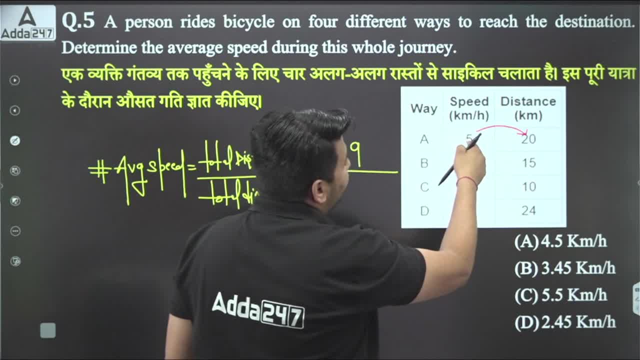 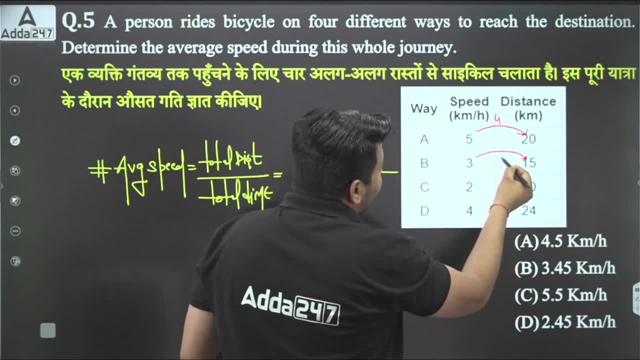 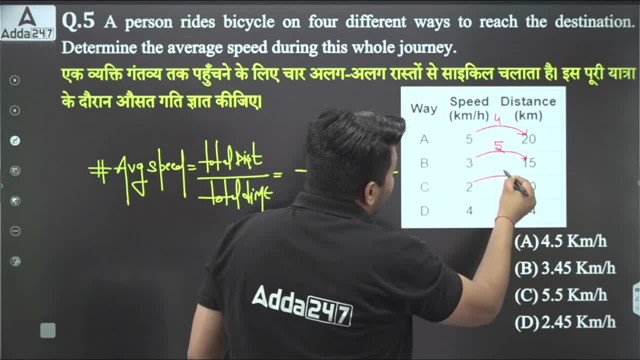 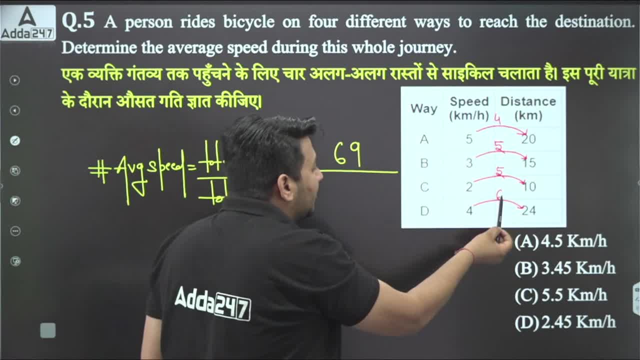 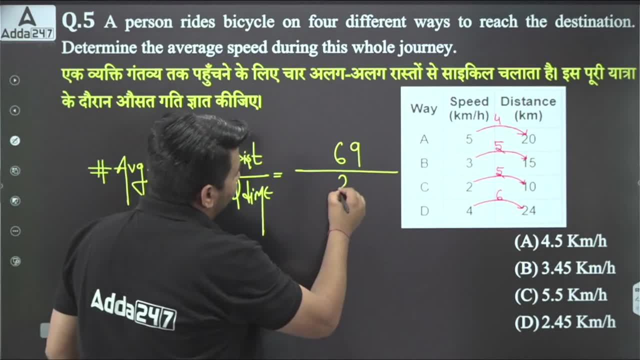 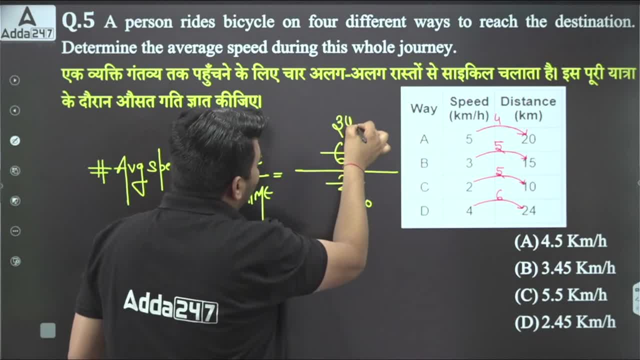 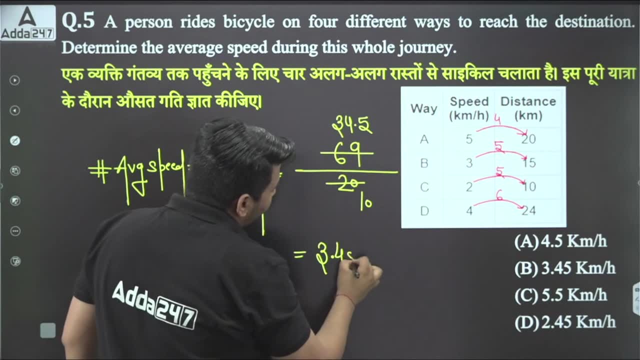 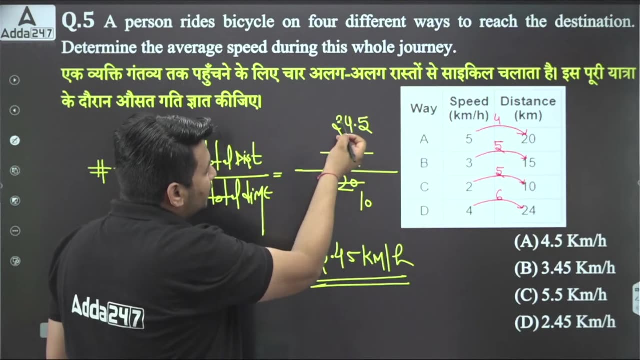 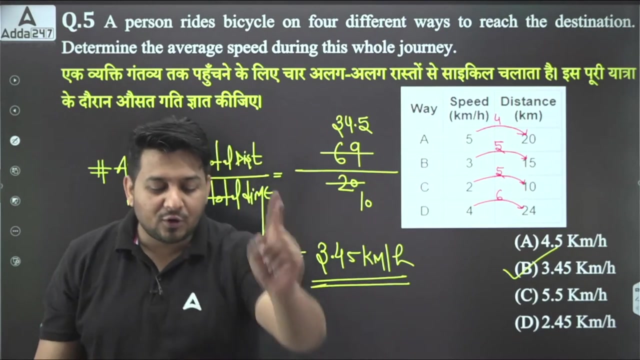 5, 20 drove 25, 25, 25, 28, 26, 27, 26, 27, 28, 29, 30, 34, 35, 36, 35, 36, 34, 34, 35, 45, 45, 46. Answer is clear or not clear? 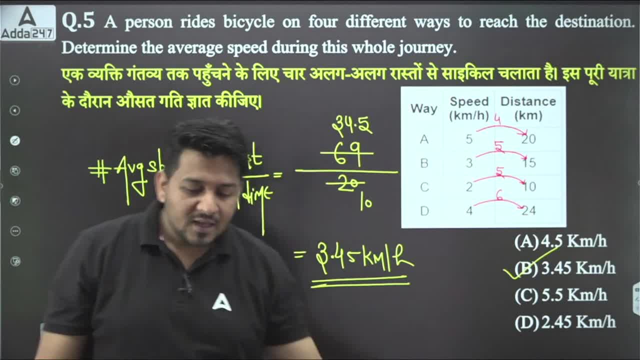 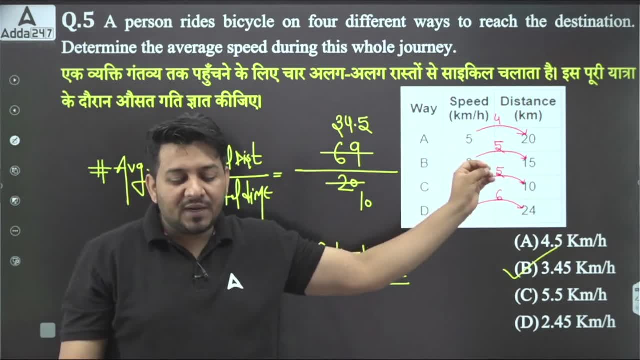 All children say yes, sir, clear, Same copy paste. question of 12th January paper From there. I have made you do it. The paper which was done on 12th January, I have made you do the question of that. Next question. 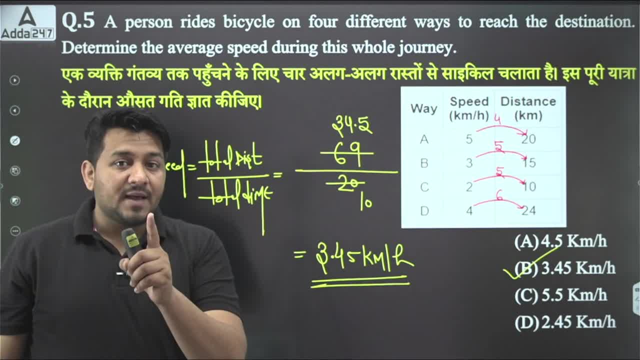 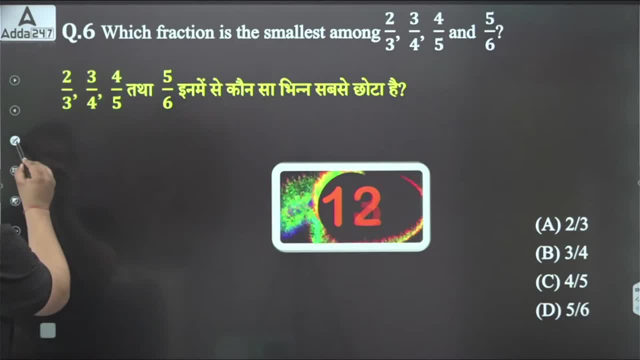 Let's move ahead. If you are understanding well, Then like and share this session. Next question. Next question: children, tell me, in front of you, Same question has been asked in your exam. Which is the smallest difference? Which is the smallest difference? 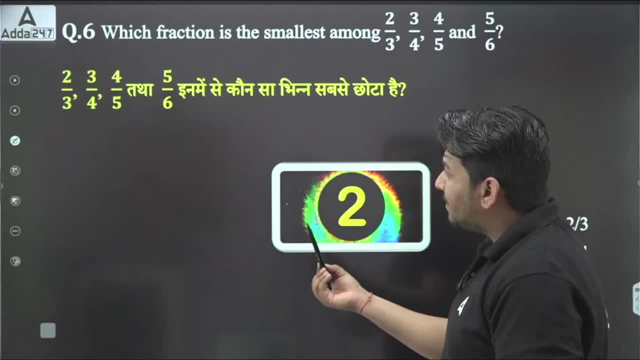 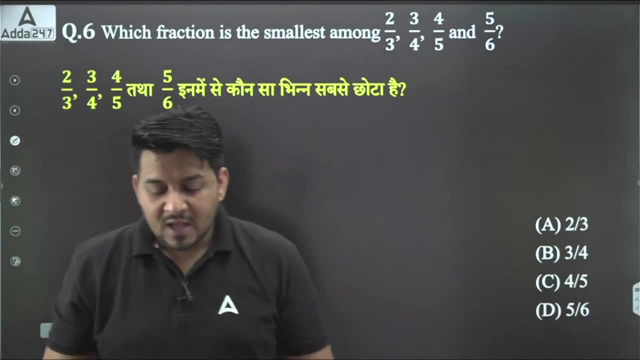 2 divided by 3.. 3 divided by 4., 4 divided by 5. And 5 divided by 6.. This has been given to you. The smallest difference has been asked from you Today. I will teach you a very easy way. 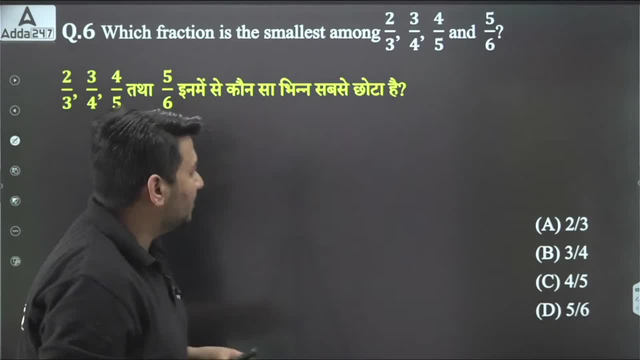 You will not be worried in life, Never. What is the first fraction value? You will say that the first fraction value is 2 divided by 3.. The second fraction value is 3 divided by 3.. The third fraction value is 4 divided by 5.. 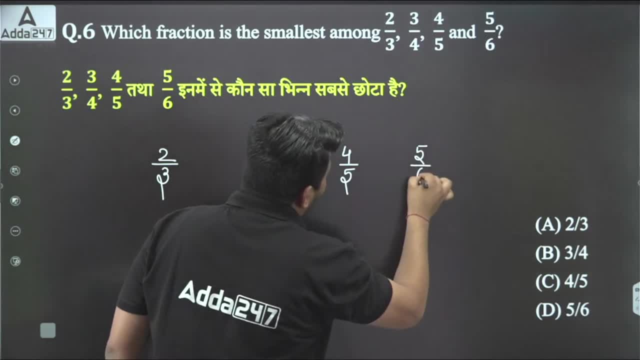 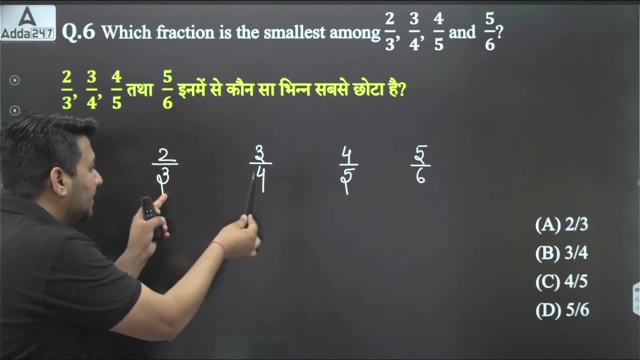 And the fourth fraction value is 5 divided by 6.. Now see, First of all, Tell me one thing: If I remove 3,, 4,, 5, and 6 from the denominator, 3,, 4,, 5, and 6.. 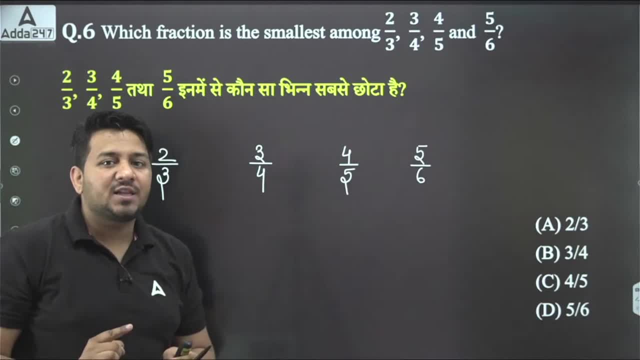 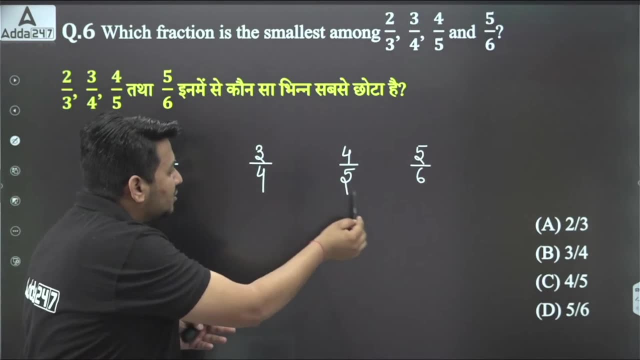 So can I say that the remaining number is divided by the full number. Yes or no? You will say yes, sir. So what to do now? You have to 3,, 4,, 5, and 6.. How many LCM will there be? 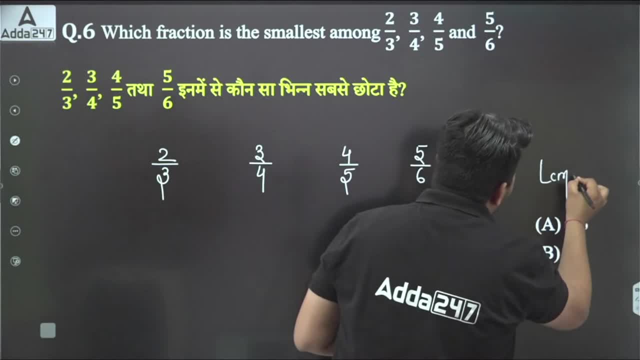 3,, 4,, 5, and 6.. How many LCM will there be 60.. How many LCM will there be 60. Tell me, will there be or not? You will say yes, sir, In all places. multiply 60.. 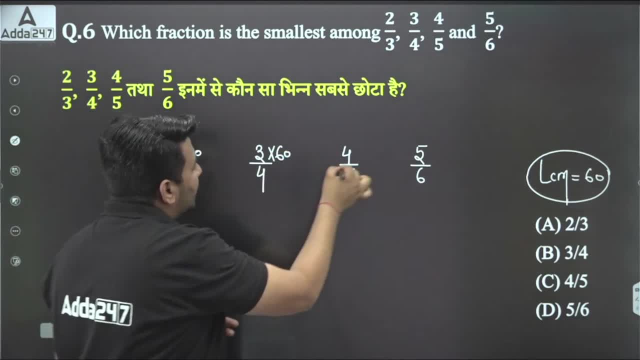 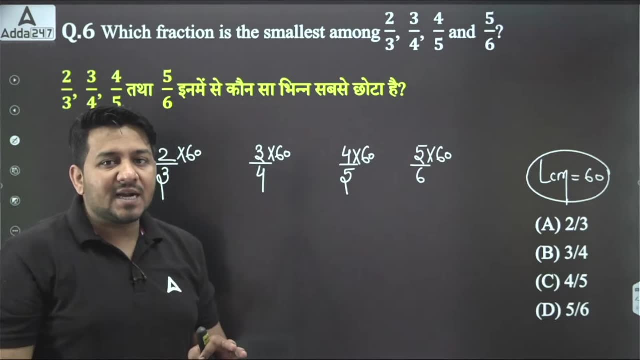 Here also multiply 60.. Here also multiply 60.. Here also multiply 60. And here also multiply 60. In all places you multiplied 60. See Cancel from 3. 20.. 20 times 20, multiplied by 2, is 40.. 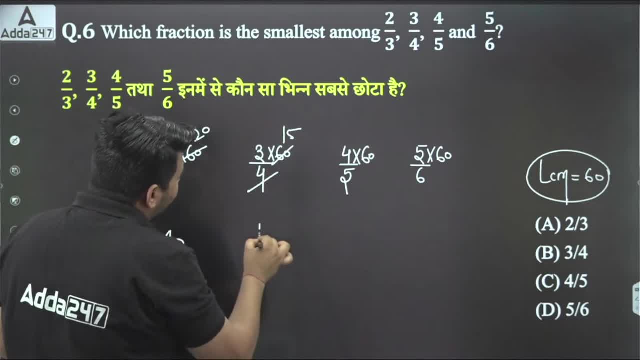 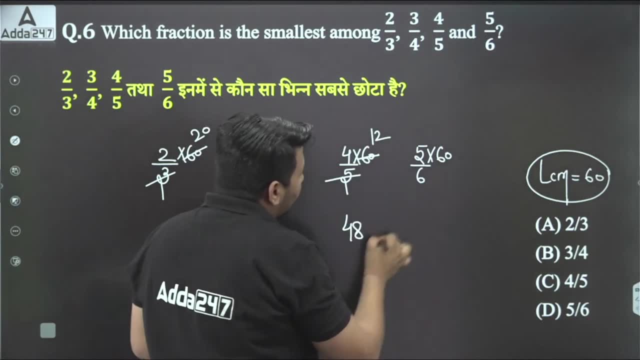 Cancel from 4. 15 times 15, multiplied by 3, is 45.. Cancel from 5. 12 times 12, multiplied by 4, is 48.. Cancel: 10 times 10, multiplied by 5, is 50.. 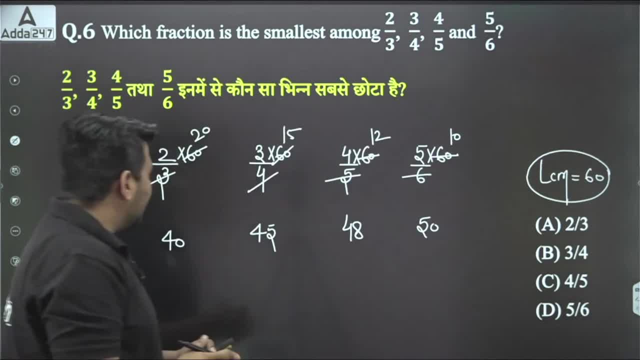 Now tell me 40,, 45,, 48, and 50. What is the smallest number? You will say 40. This is the smallest number. This is the smallest number, And this is the smallest number. And this is the smallest number. 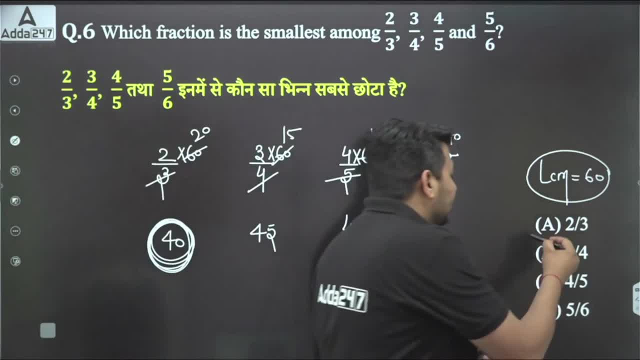 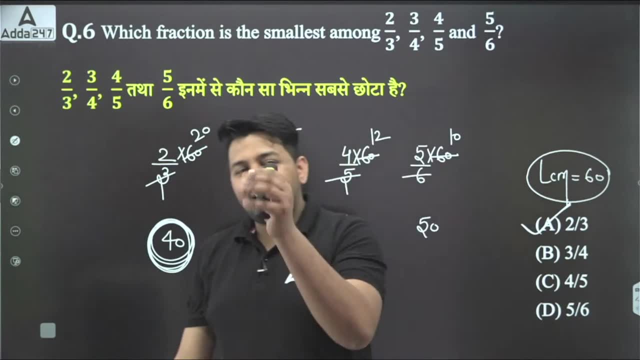 And here what is seen is: This means the smallest number is 2 divided by 3.. 2 divided by 3 is the smallest number. Is it clear? One more trick, If you want to do without pen and paper. So what do we do now? 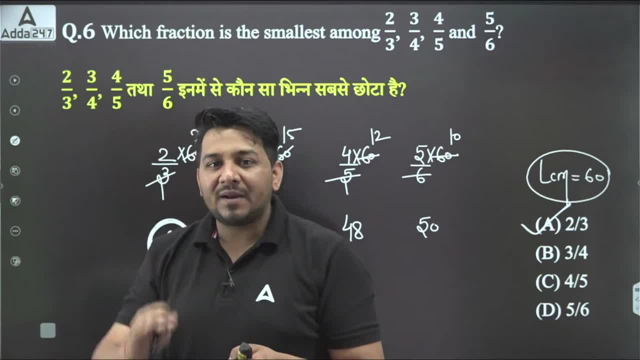 If you want to answer the question without pen paper, I want that. Sir, I will not do this. also, Now tell me what you will do. So I have taught you one more trick. Ask me: what is it? I said, the difference here is 1.. 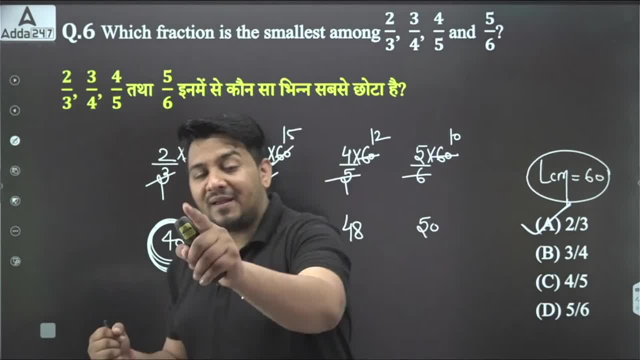 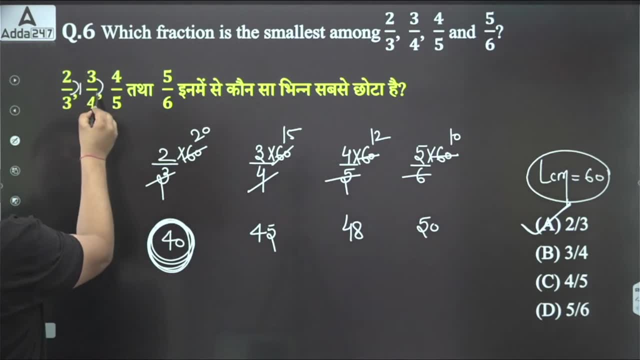 The difference here is 1.. And I will show you how to do it. See there is no change in the paper. Now how to do it. See what is this difference One: Here the difference is 1,, here the difference is 1, and here the difference will be 1.. 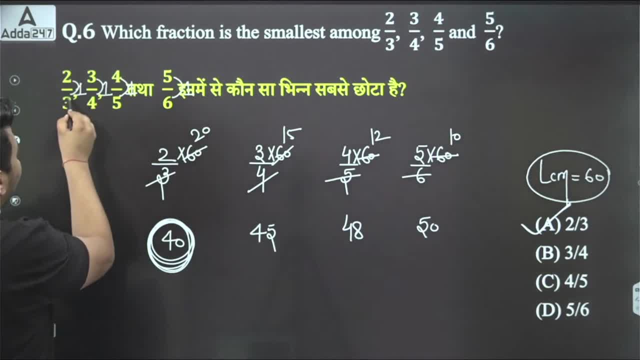 If the difference is equal in all places, then the one whose part is small will be the smallest bin and the one whose part is big will be the largest bin Brother. the one whose part is small is the smallest bin. the one whose part is big is the largest bin. 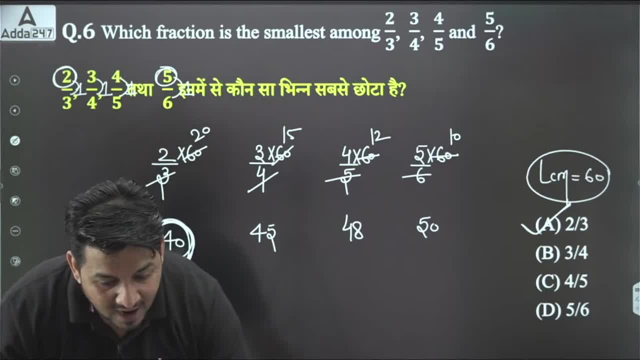 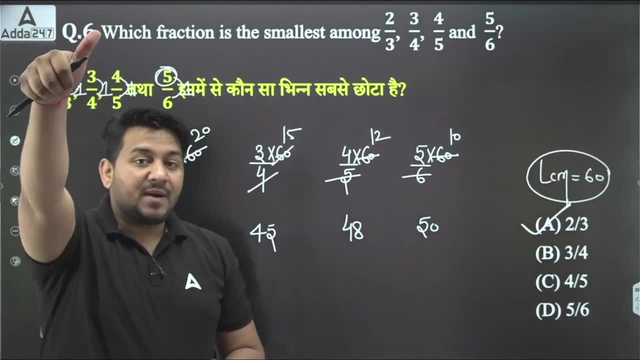 Done Clear. You could have answered with difference. my children Clear. Next, let's move ahead Quickly. all the children like and share once. then I will move ahead Quickly, share once. Next question: children in front of you. 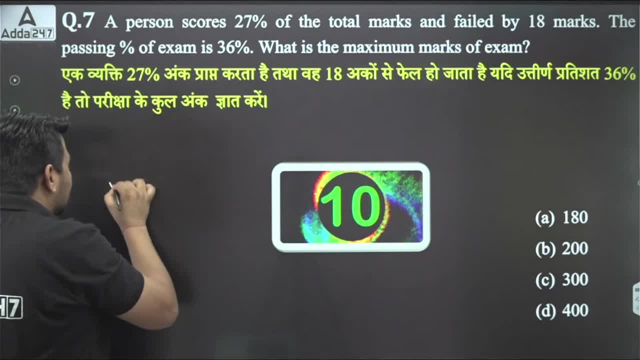 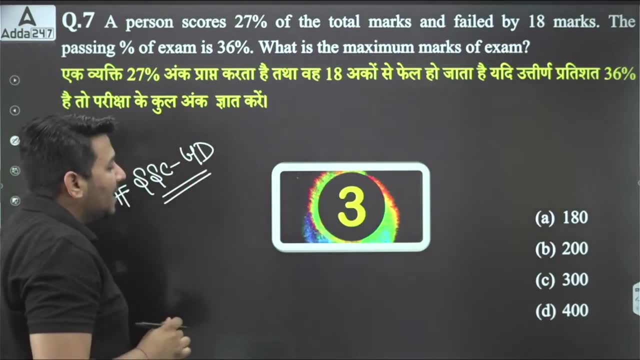 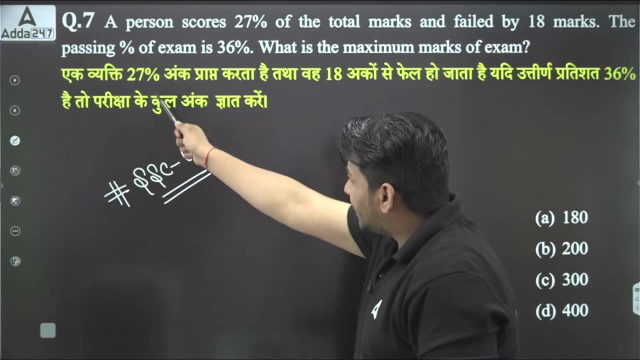 Now let me tell you, like some of your favorite things, SCGD's favorite question. he asks every time. every time he asks, every time he will ask you this question. What is the question? One person gets 27% of the number. 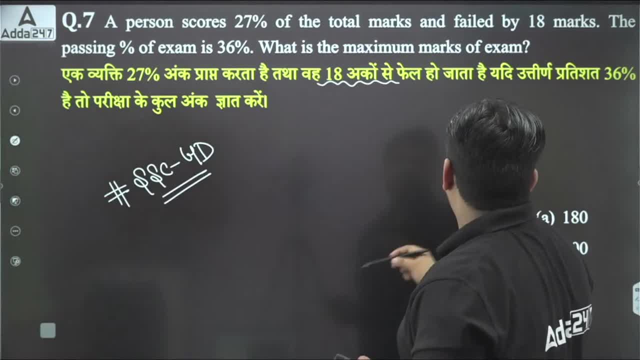 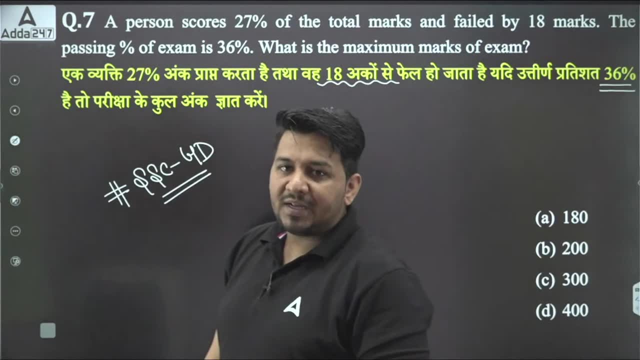 And 18 numbers fail. How much is the percentage of getting 36%? So how many are the total numbers of the test? How many are the total numbers of the test? How will you get it? I will teach you a very easy trick. 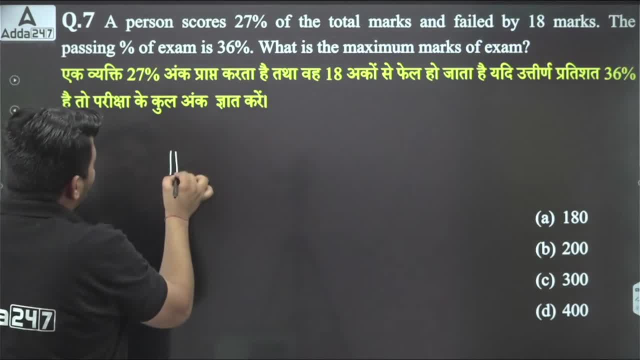 Look My brother. tell me one thing: How many are needed to pass 36%? If you bring 36% number, then let's assume you pass. What did I say If you bring 36% number, If you bring 36% number? 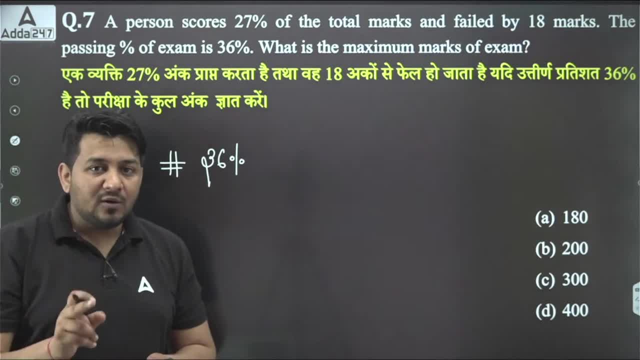 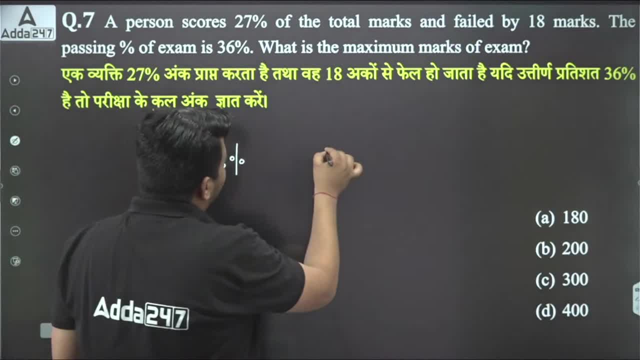 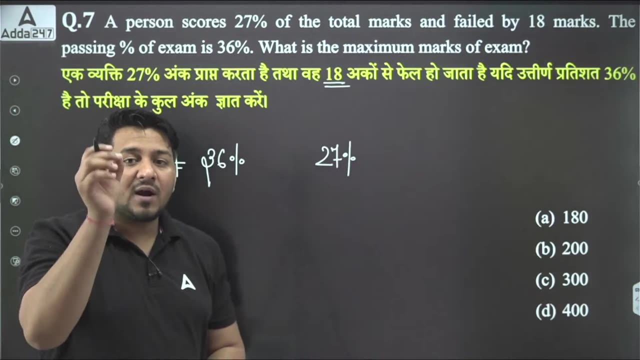 But how many did you bring? 27%? You brought 27% number. And how many numbers are failing? 18 numbers, Brother. you brought 27% number and you are failing with 18 numbers. If I give you 18 more numbers. 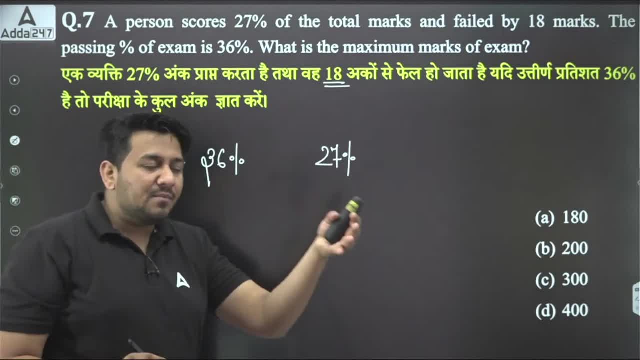 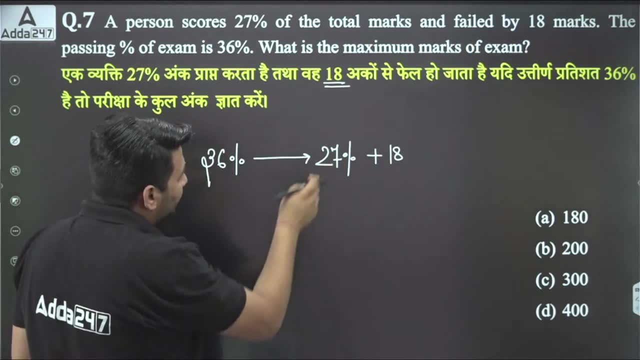 Brother, if you are failing with 18 and I give you 18 more numbers, If I give you the pass, then will you pass? Absolutely will be Guruji. If you pass, then equal to 36%, Bring it here. Take this 27 and bring it here. 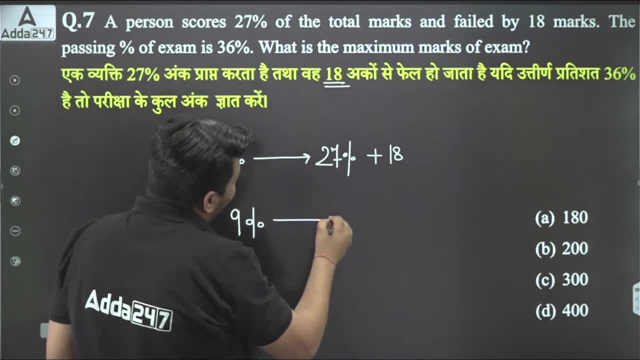 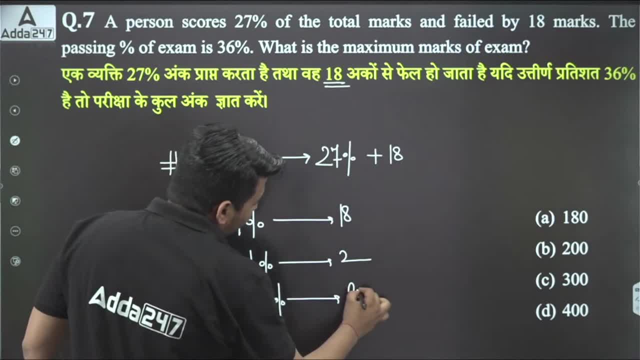 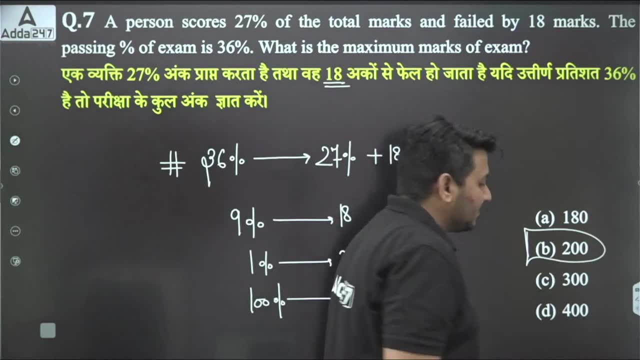 100% is 200.. How much is the value of 100%- 200? These are the total numbers of the test. These are the total numbers of the test. Which option is number B? Say clear or not clear. All the children comment once. yes, sir, clear. 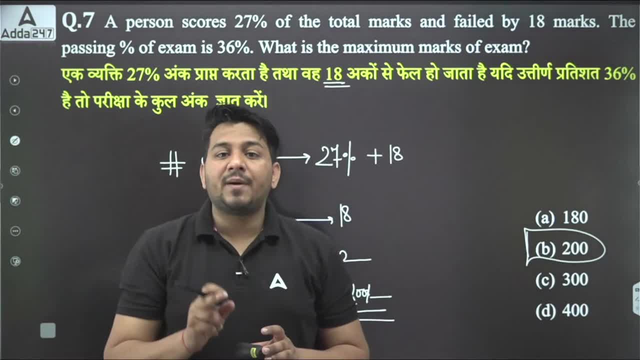 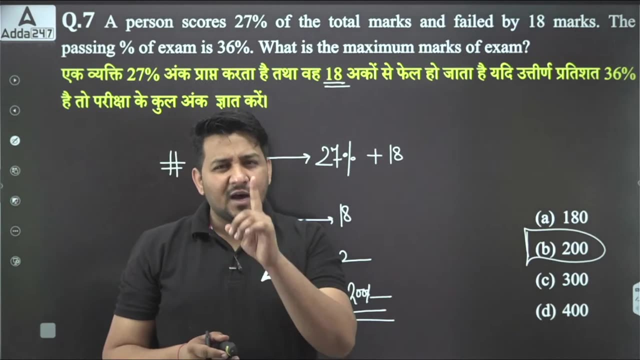 If you are studying math for an hour in the morning, I am telling you again, You are doing the biggest work of the day today. Today, if you study math for an hour daily in the morning- Because if the children are on the subject of your selection, Then it is math- 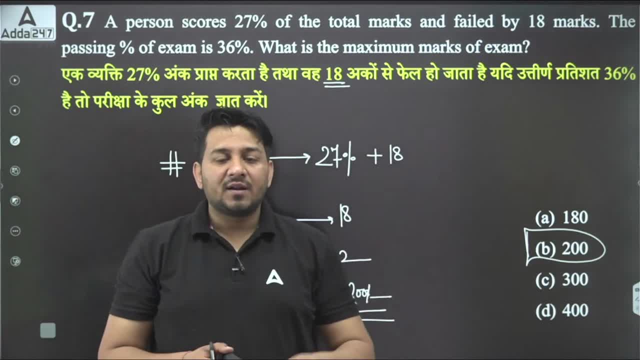 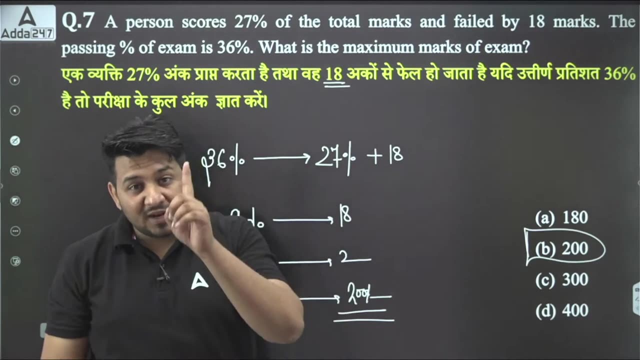 All the children will do reasoning. Even if you give less time in reasoning, you will do it. In GS it is very uncertain What will be right, what is wrong, But if you do math you will do it 100% correct. So the most important subject this time is math. 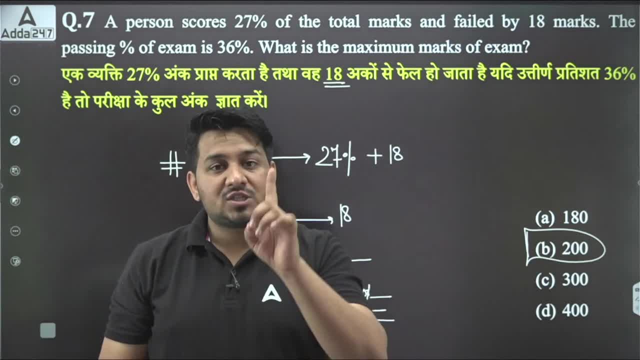 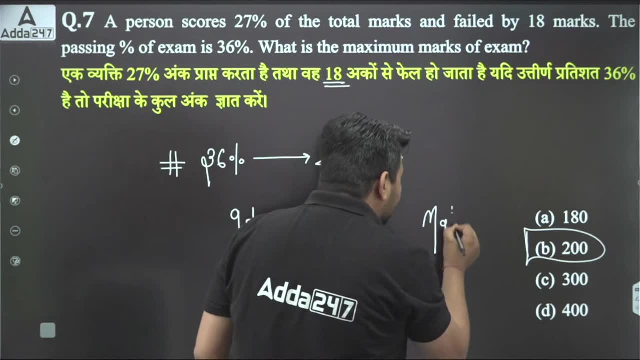 Which will give your selection? Now, if you do math, Believe it or not, It depends on you. Now the selection will be of only the child Whose hold on this subject will be the most On math, If your hold is the most on this subject. That's why I am not saying that I teach. 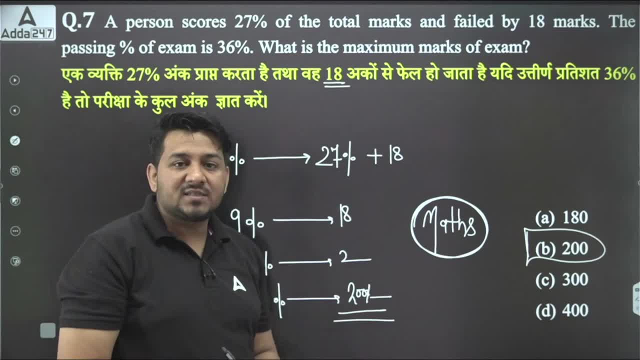 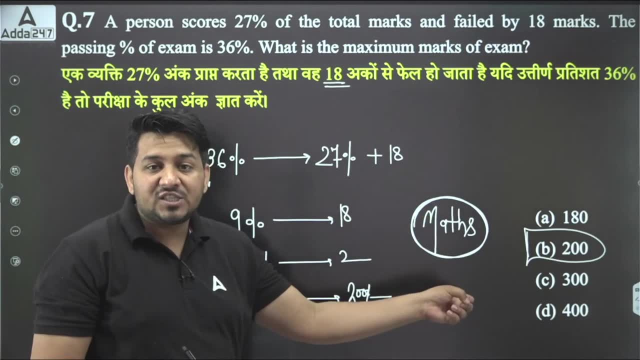 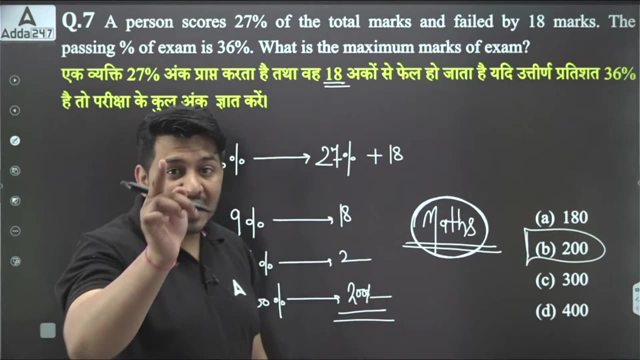 That's why I am not saying that I teach math. That's why I am saying: Because you do analysis yourself The previous year, of the children who read analysis on the channel, Go and see that the whole selection somewhere, Only one subject depends on math: the most. Next question: 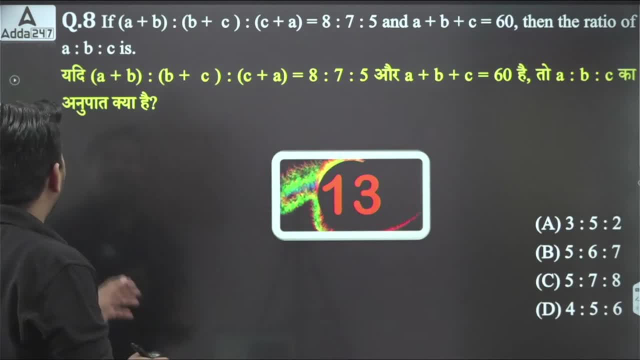 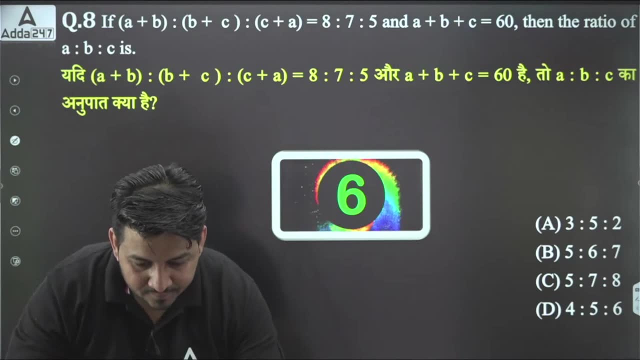 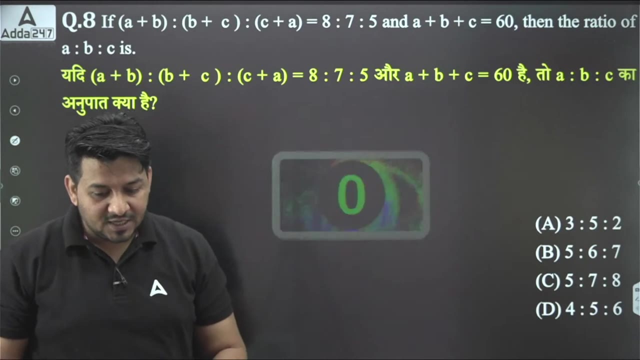 Next question: children. Very, very, very important. And we will teach a new trick for this question. And you know One of the favorite questions of SSCGD- Ok, One of the favorite questions of SSCGD. One of the favorite questions of SSCGD. I also put the mensuration today. 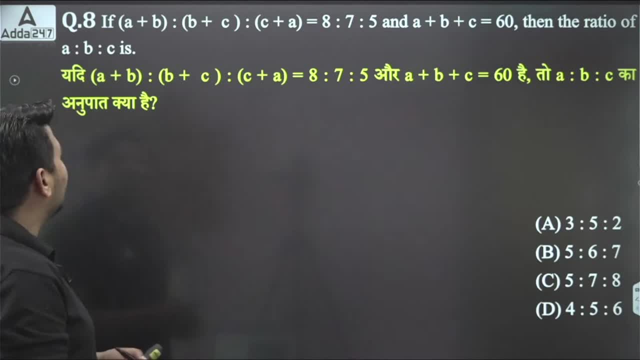 Ok, Don't worry, See what the question is saying. A plus B, Ratio B plus C, Ratio C plus A, Which is equal to Eight answers Seven answers Equal to five. If A, B, C is equal to how much Sixty. So tell me How much is A Ratio B, Ratio C? 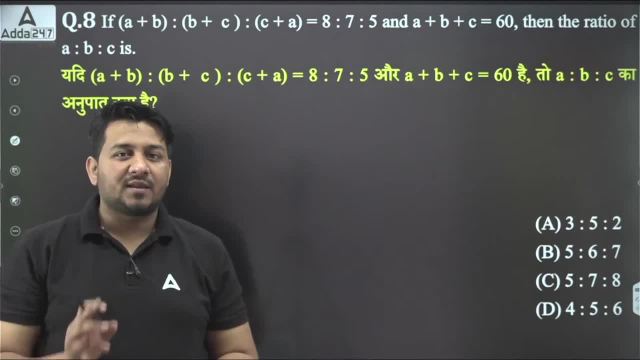 I will teach a wonderful trick. See very carefully If I add these three children. See A plus B. I did not do anything. Tell me A plus B. How much is here? B plus C? How much is here A plus B? How much is here? A plus B? How much is here? 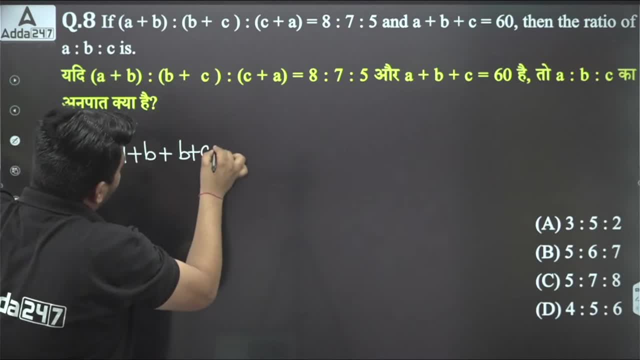 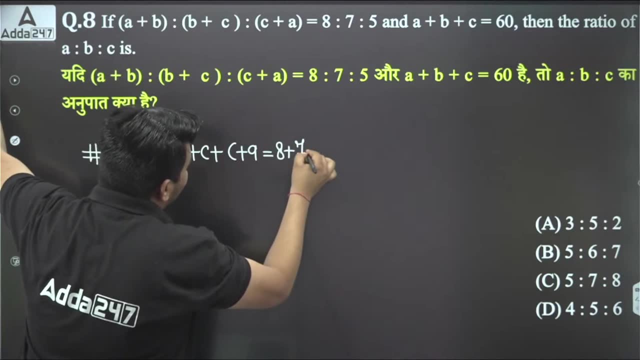 B plus C. How much is here C plus A? Which one is equal to A plus B, A plus B, A plus B, 8 plus 7 plus 5, Even, How much is this? How much is this? How much is this? A plus A, 2A? 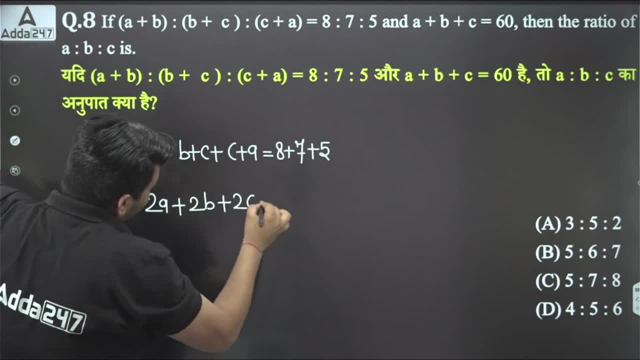 B plus B, 2B, C plus C, 2C, 8, 7, 15, 5, 20, 2C, 8, 7, 15, 5, 20. If you cancel two of them, How much will be the value of ABC? How much will be the value of ABC? 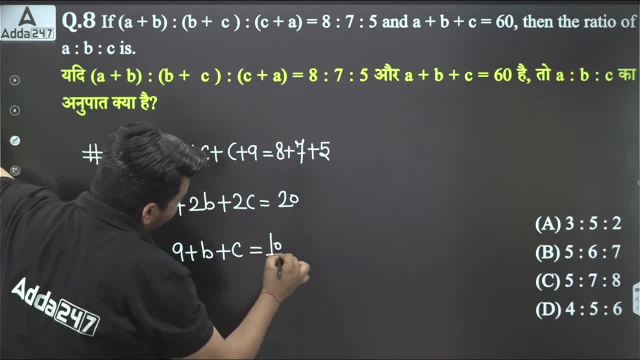 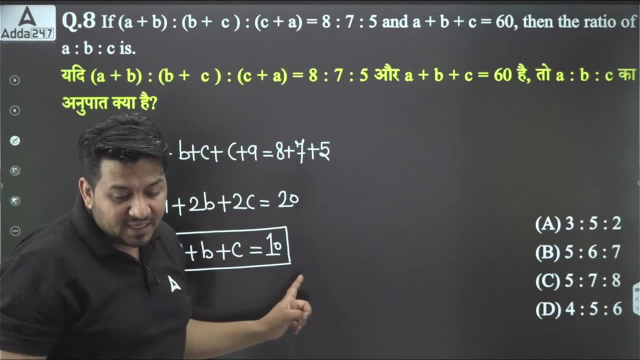 times 2, How much will it be? I have taken the value of a b c. Tell me one thing: what did you take out of the value of a b c? You will say 10.. And what is the actual value of a plus b plus c? 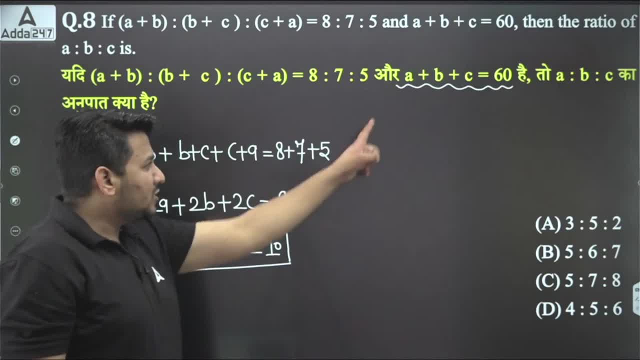 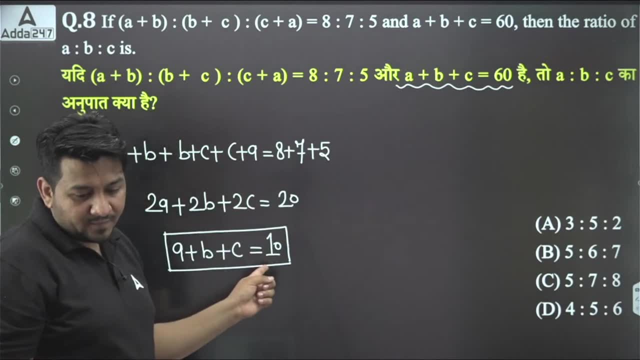 It is 60.. See the actual value of a, b, c is 60.. What is this? It is 10.. That means this value is 6 times less than the real value. See carefully: The real value is 60 and this is 10.. 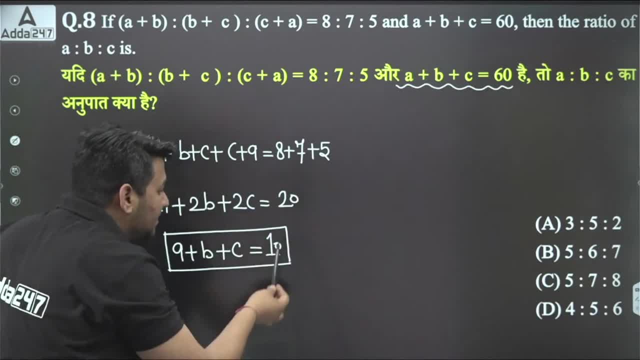 That means this 10 is 60 times less than the real value. So don't sit here to balance. I will tell you when to balance. First, you take out the value of a from here. How will you take out the value of a? 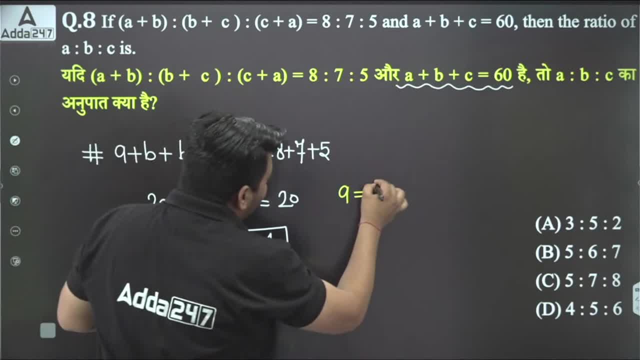 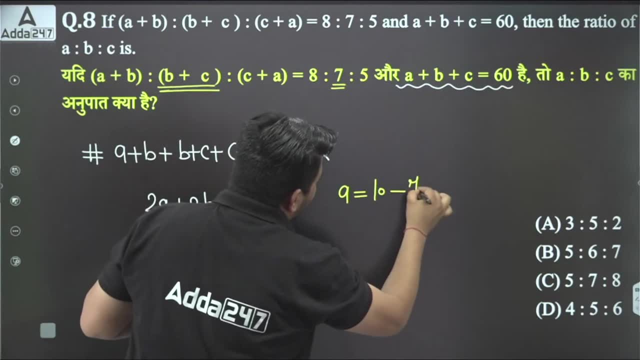 You know that the sum of all three is 10.. If you want to take out the value of a, then b plus c. What is the value of b plus c? 5. Reduce it. What is the value of 7 out of 10? 3.. 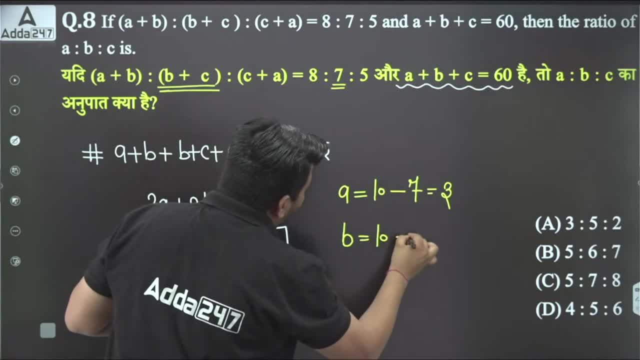 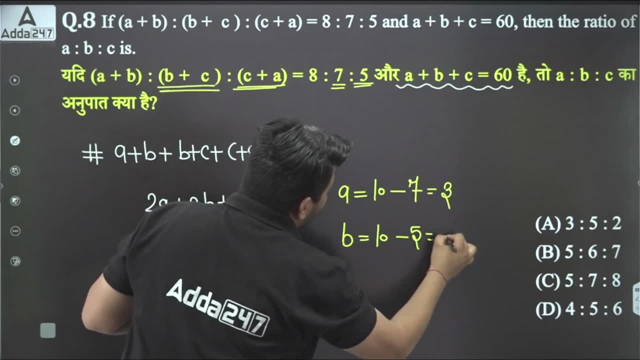 In the same way, what will you do when you take out the value of b, b plus c? To take out the value of b, what is the value of c plus a? 5. Reduce it. How much will it be? 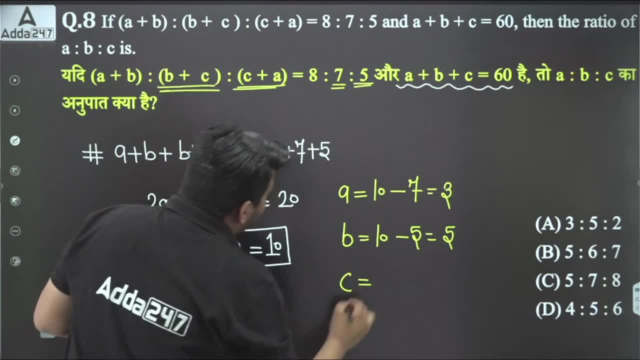 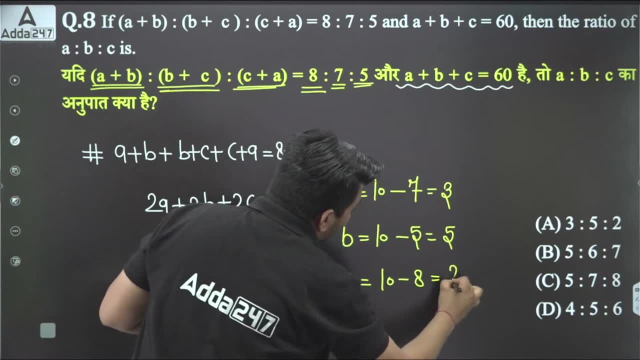 5. Okay, What will you do to take out the value of c? To take out the value of c, what is the value of a plus b? 8. Reduce it. How much is 8 out of 10?? 2.. 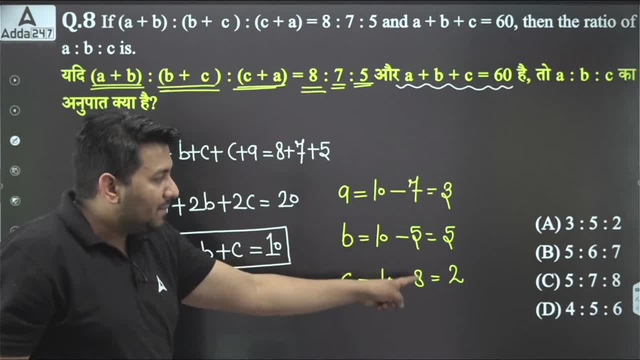 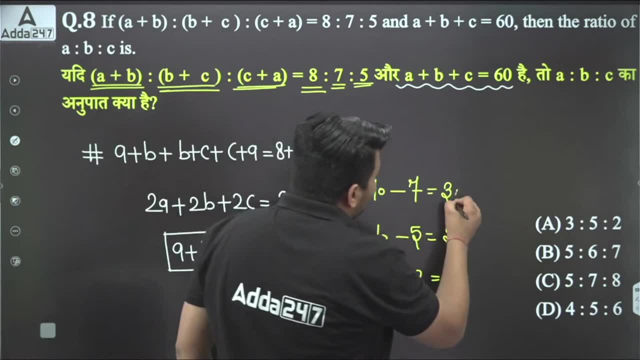 And now the value of a, b, c has come out. Now, children, the value of a, b, c has come out. This value is 6 times less than the actual value. So what to do? Multiply this by 6.. 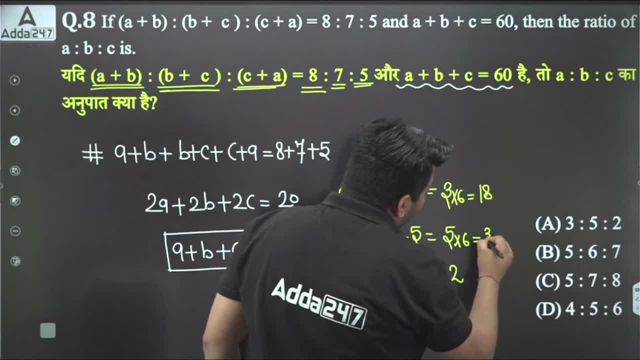 How much will it be 18.. Multiply this by 6.. How much will it be 30.. Multiply this by 6. 12. Now you add 18,, 12,, 30, and 30,, 60.. 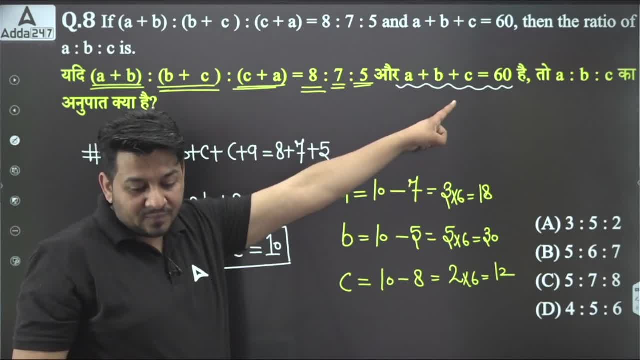 What is the value of a, b, c, 60. Is it clear or not clear? Look, the value of a, b, c is 18,, 22,, 18, and 12.. How much will it be? 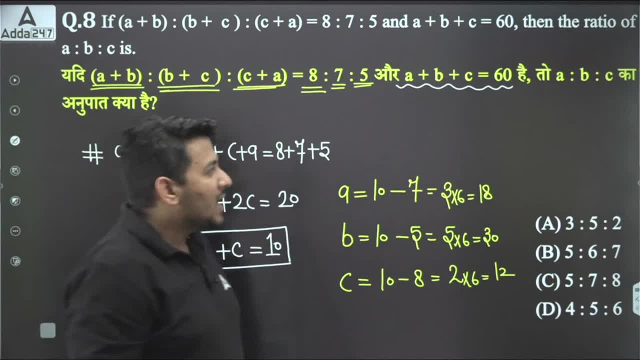 30 and 30, 60. The value of a, b, c is 60. Now we have been asked the ratio. What will be the ratio of a, b and c? Tell me How much will it be? 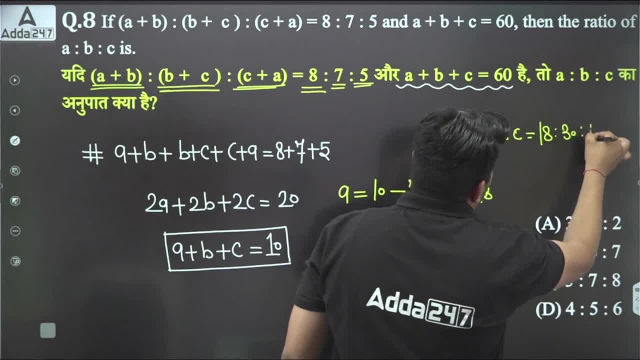 18,, 30, and 12.. Cancel the value by 6.. 6 times 18.. 6 times 5 is 30.. 6 times 12 is 6.. Alright, 3 times 5 times 2.. 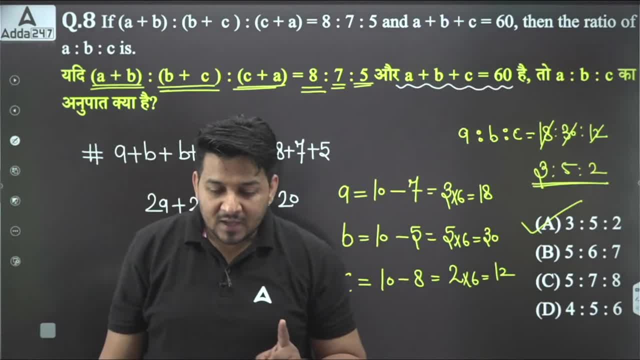 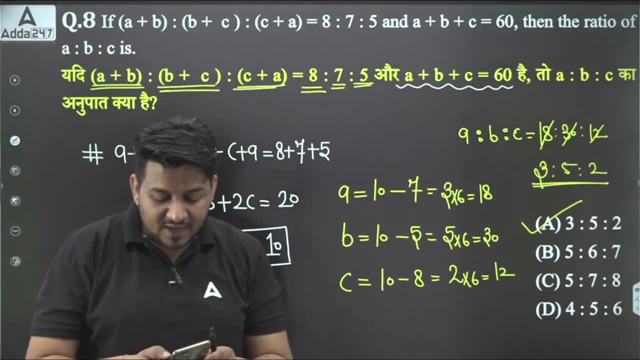 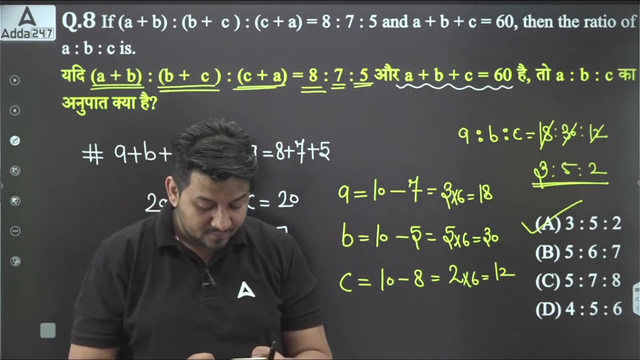 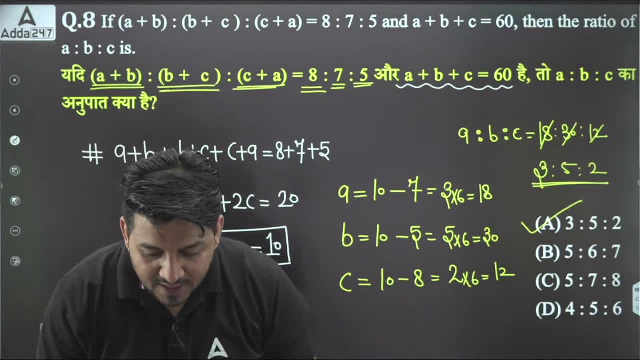 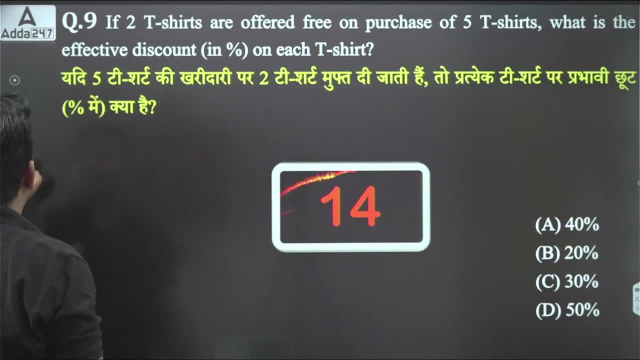 Mere bhai Jaldi se ek baar comment karo. yes, sir, clear. Kya aapko itna samajh me aagya Agla question? bachon aapke saamne Same question. aapke exam ka hai Bataye? 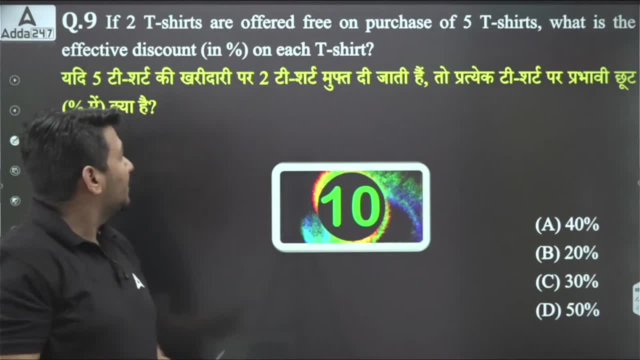 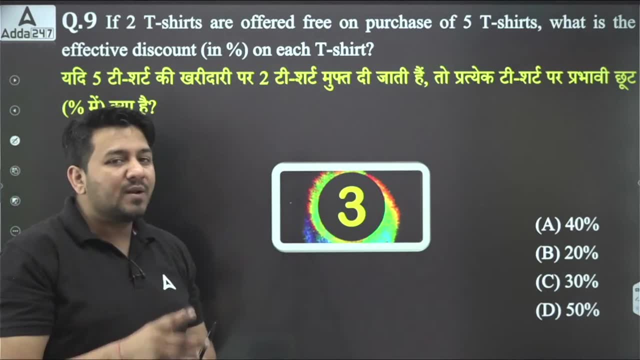 Yadi paanch t-shirt kharidne par. Yadi paanch t-shirt ki kharid par Do t-shirt-e muft di jaati hai To prateek. t-shirt par prabhavi chhoot kitni hai Paanch t-shirt kharidne par do t-shirt free hai. 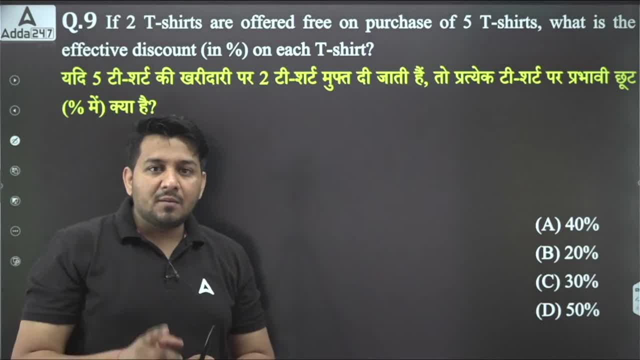 To kitne percent ki chhoot hai, Agar paanch t-shirt kharidne par, Do t-shirt-e aapko free mil nahi hai. Kitne pratishat ki chhoot hai, Kaise nikalogay Dekho, bachay, Is question karne ki trick. kya hai? 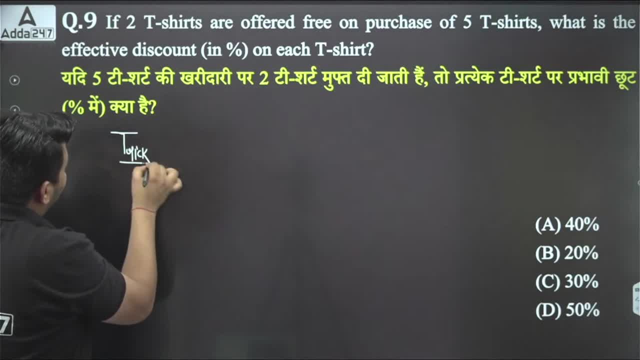 Is question ko karne ki trick kya hai? Bachay bahut dhyan se. dekho, Paanch t-shirt kharidne par Do t-shirt-e free. hai Iska matlab shopkeeper ke paas Paanch aur do saat t-shirt-e hongi. 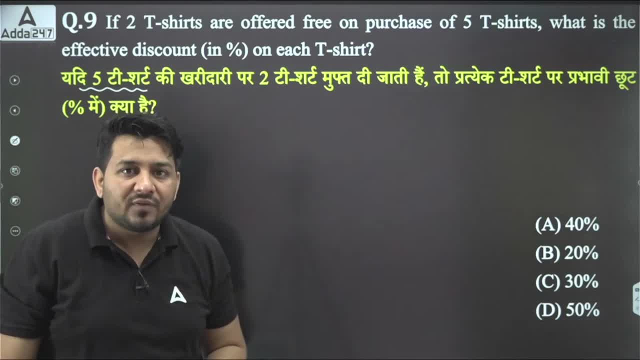 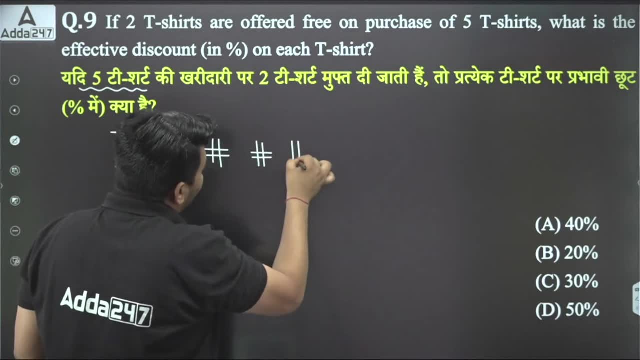 Bhai saat t-shirt-e Tabhi to paanch kharidne par do free dega Bolo. Bhai, paanch kharidne par do free dega Iska matlab. saat t-shirt-e hai 1,, 2,, 3,, 4,, 5, 6, 7. 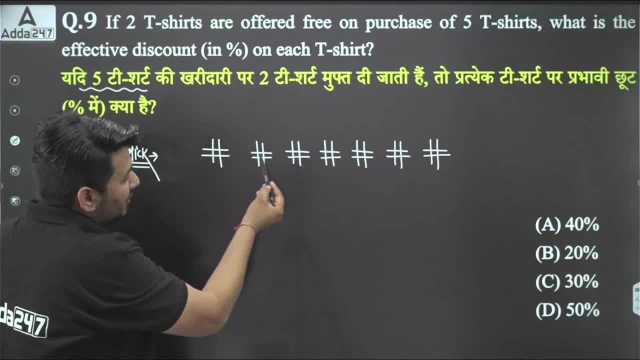 Kitni t-shirt-e Saat t-shirt-e hai 1,, 2,, 3, 4,, 5, 6, 7. Kitni t-shirt-e hai Saat t-shirt-e hai Maanlo bete Ek t-shirt ki keemat ek rupay hai. 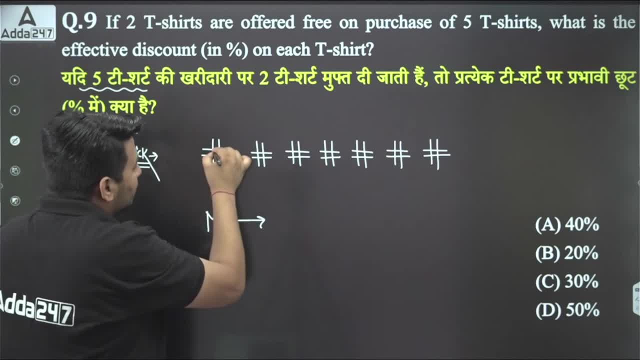 Ek t-shirt ki keemat Bete. Ek t-shirt ki keemat Ek rupay hai. To saat t-shirt-e ho gayi bete. To saat t-shirt-e ka mark price. Kitna hoga Ayi batao Saat t-shirt-e ka mark price. 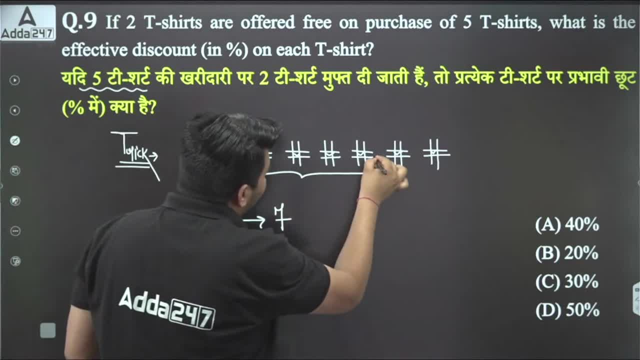 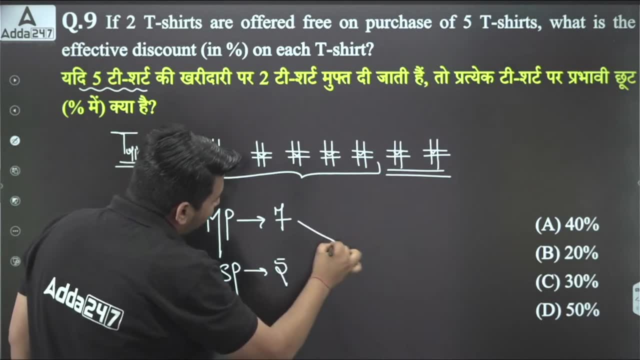 Saat rupay hoga. Usne aap se kaha, ki Saat paanch t-shirt-e ke liye pay kar, do Do t-shirt-e free dega, Yani selling price. bete Kitna hai Paanch rupay, Yani saat rupay ki cheech. 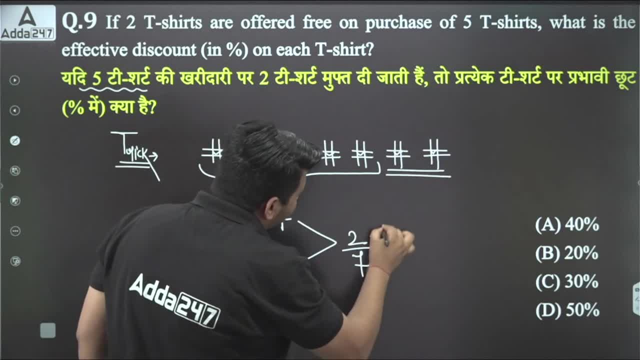 Paanch rupay me bech raho Do ka discount de raho Saat pe To batao saat par kitna hoga Do saat bate saat, Do saat bate saat. Yani saat duni chauda Thik hai, Thik hai. 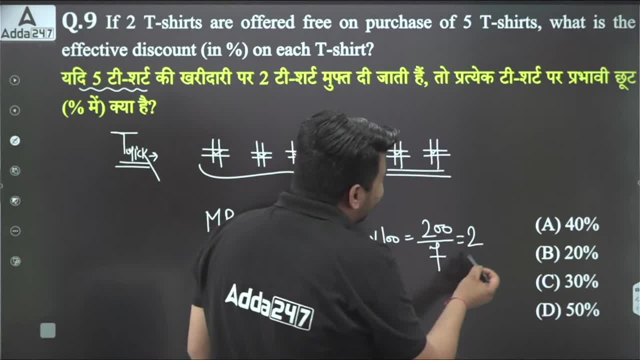 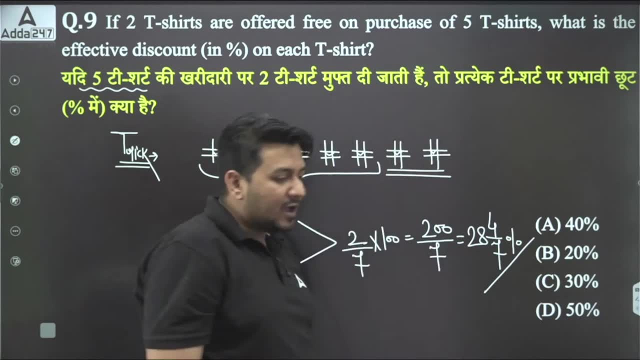 Thik hai. Saat duni chauda Che bacha saat ho gayi Saat ate Chapan Chaar saat Thik hai, Ye kitna hoga: Twenty eight four by seven percent Option. ye aayega Option error hai bete. 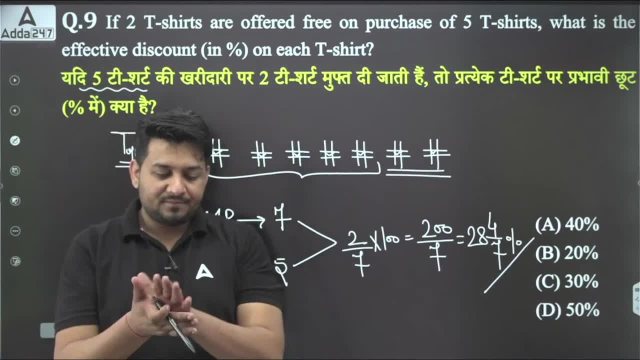 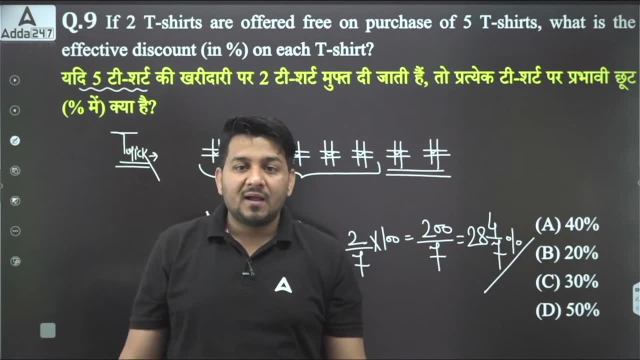 Option error hai. yaha par, Wah, Kya baat hai, Matlab galat option me bhi option nikal dete ho. tum log, Bhaiya Galat me bhi option aajate hain. aap logon ke Socho, saare option galat hai. 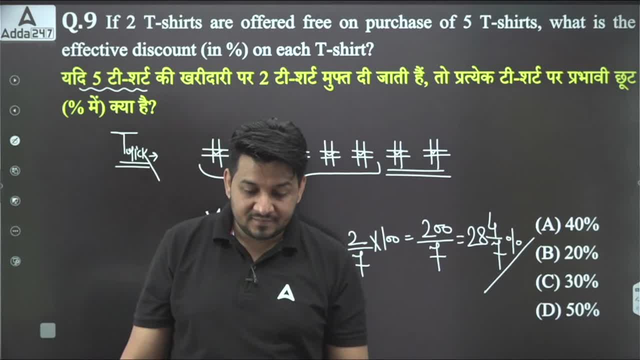 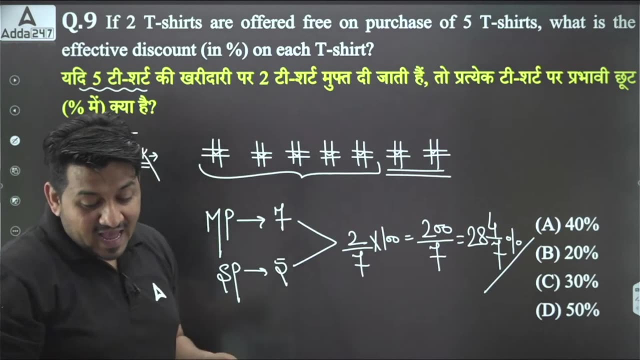 Uske baad bhi tum ne answer nikal liya. Socho: saare option galat hai, Prabhu, Prabhu, tum kahaasre aa ho, Prabhu, Kya matlab kar ke maanoge, Kyakar ke maanoge. 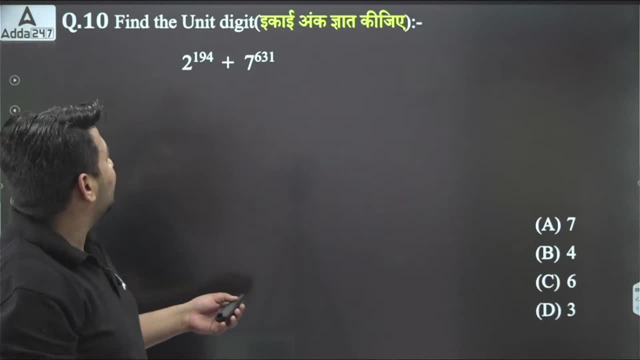 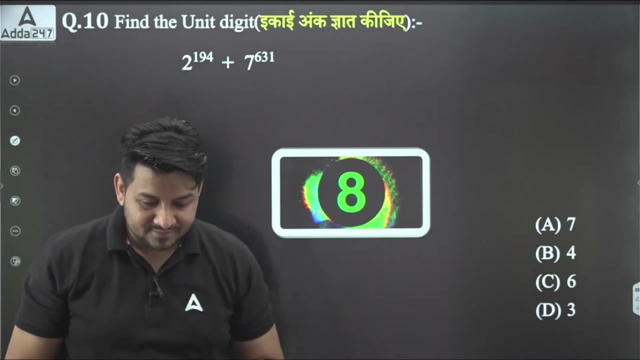 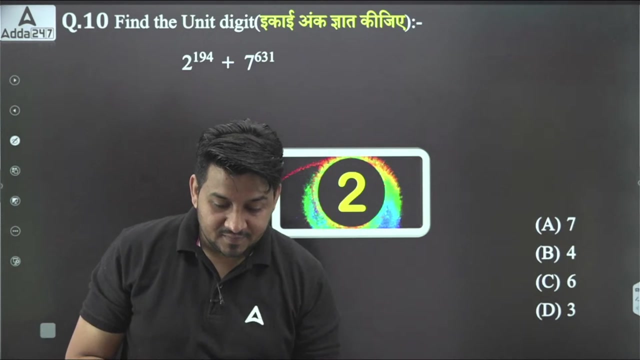 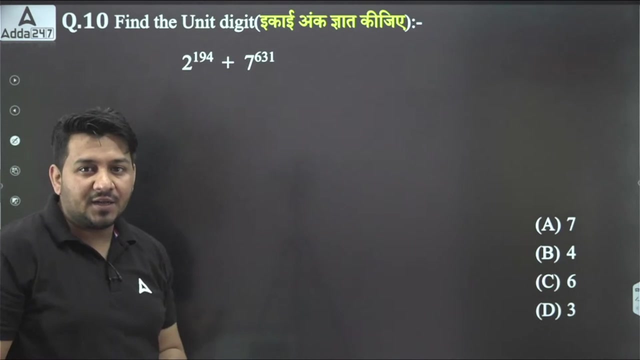 Chalo. next question: bachao aap k samane bataye Unit digit par bete mitt badi hai. If there is one question in your exam, all the students will share it once. share it quickly. What is the question saying 2's power is 194 and 7's power is 631.. 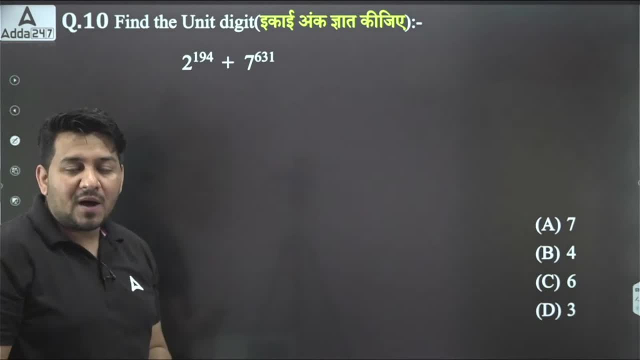 2's power is 194 and 7's power is 631.. And you were asked to tell me the number of 1's. How will you find out, For example, how much is 2 on the unit digit? How will you find out? 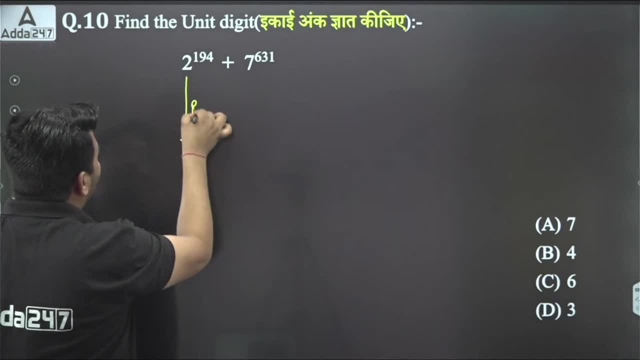 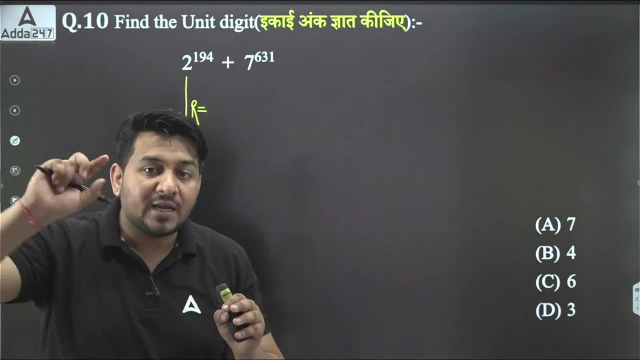 Whatever the power is, divide it by 4.. Divide 194 by 4, how much will it be? See, the divisibility rule of 4 is: either divide the whole number by 4 or divide the last 2 digits by 4.. 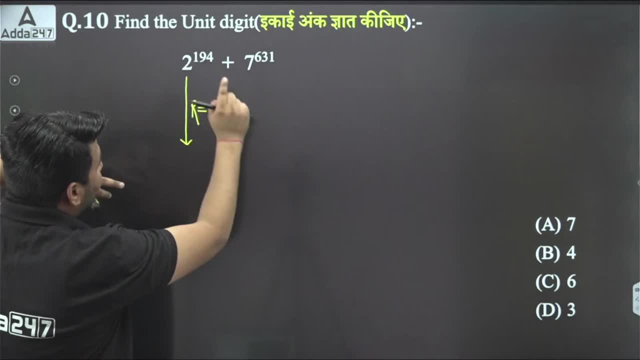 So how much is the last 2 digits 94. Divide it by 4.. Not 4, 8.. 1 is left, 14 is left, 4 is 12.. Divide 194, how much will it be? 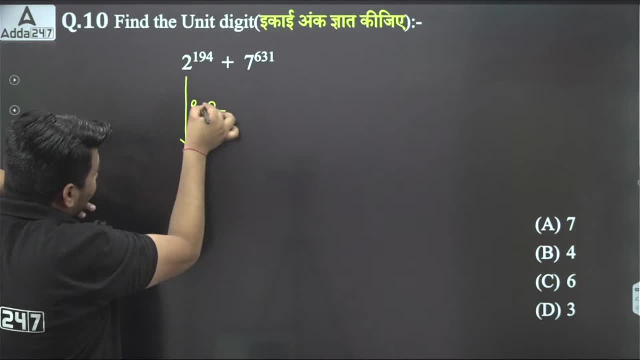 It will be 2 sespal. So whatever 2 sespal is, divide it by 2.. If you put it on the unit digit, then the power of 2 is 2.. That is how much will it be? 4 unit digits will come. 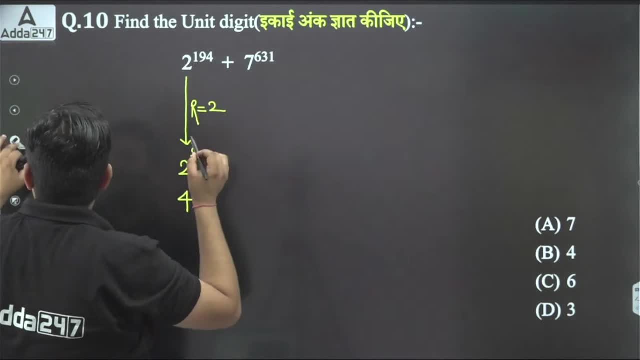 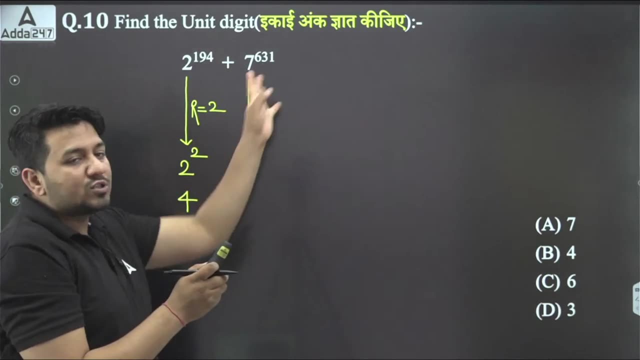 Just like this. Now see, I am talking here children. What will you do? here I am talking about 7. 631.. Like 631, divide it by 4.. Divide 31 by 4.. 4,, 7,, 8,, 29,, 30,, 31.. 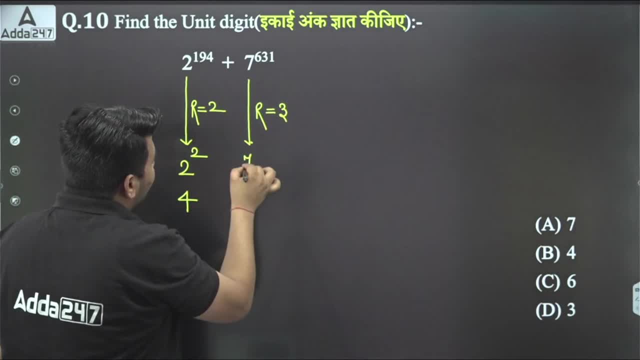 That is, how much will sespal come? 3 will come. Do the power of 7, 3.. How much will it come? What is the power of 7, 3, son, Tell me this. Power of 7 is 3.. 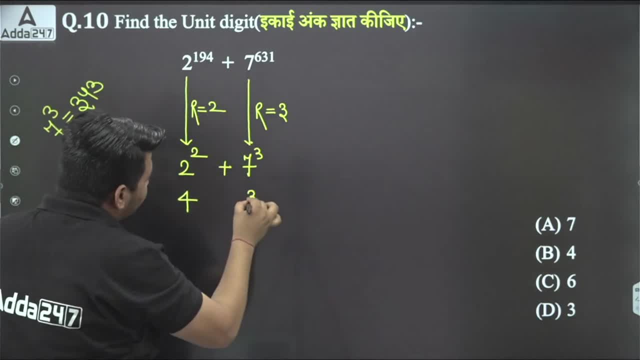 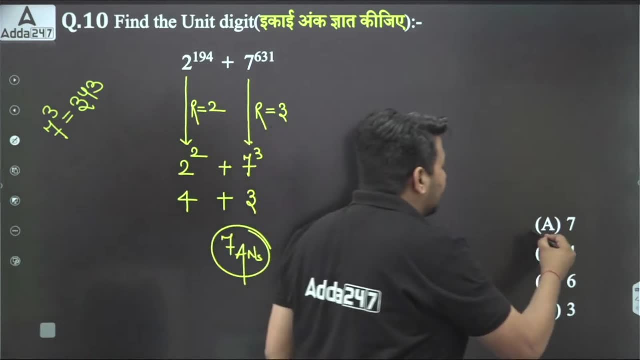 343.. Tell me, does it happen or not? That is, how much will the unit digit come? 3 will come, And how much is 4 and 3?? 7, son, your unit digit came out. 7, son, your unit digit came out. 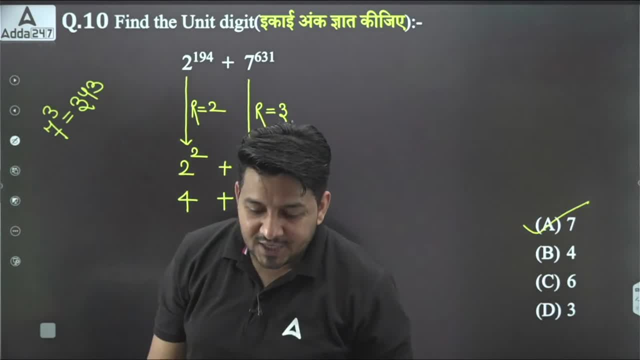 Tell me, is it clear or not clear? 7, son, your unit digit is there. Tell me, is it clear or not clear? 7, son, your unit digit is there. Tell me, is it clear or not clear? 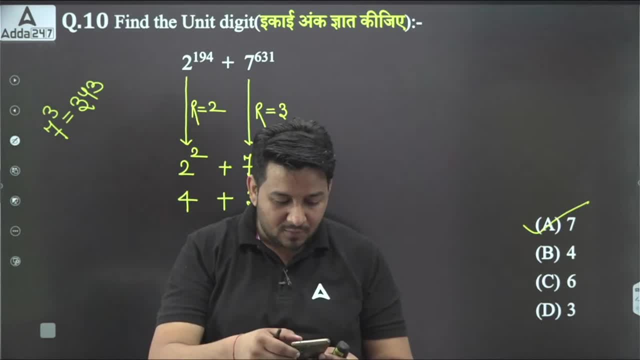 Today I feel that there is some problem in between. Okay, I think, children, some problem came in between slightly, But it is okay now It is properly okay. children, This is not a problem. All children will walk, sharing, like and sharing. 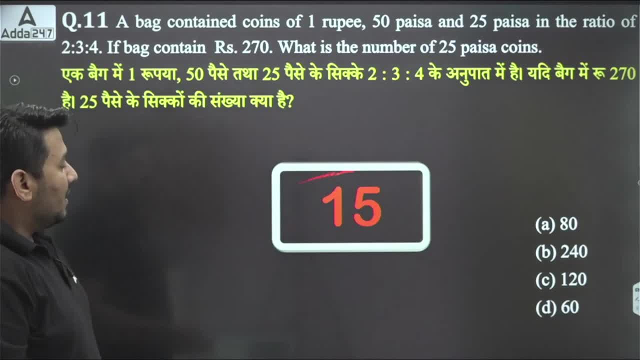 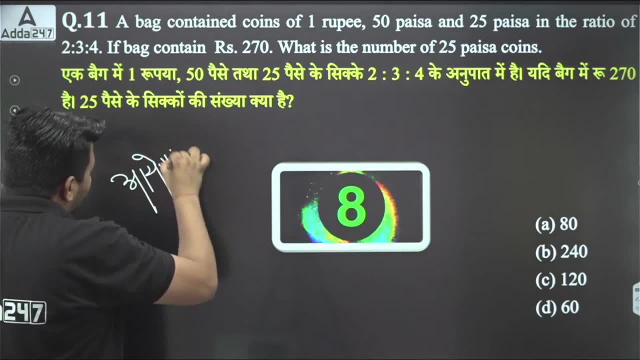 Next question: children, in front of you I write down this question and give it that it will come. Go pick up your paper. see It is repeated at least 20 to 30 times And it will come in your exam 100%. 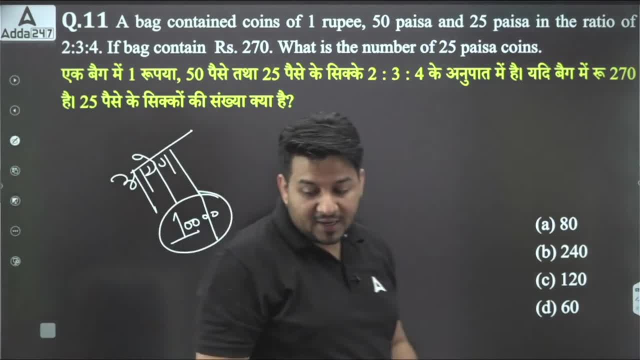 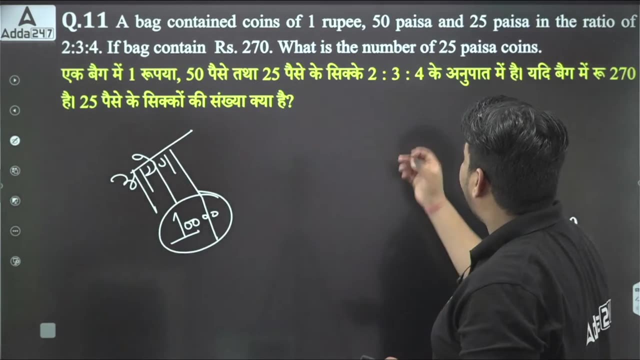 I am writing down this question and giving it son. It will come in your exam. Son, take it, Don't worry, there will be no buffering In one bag. 1 rupee 50 paise zata, 25 paise ki sikke, 2, 3 aur 4 ke anupat mein hai. 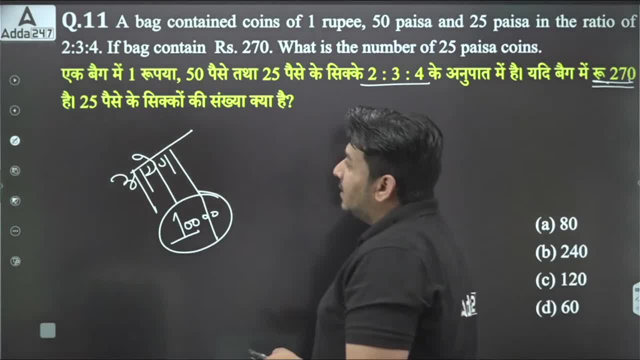 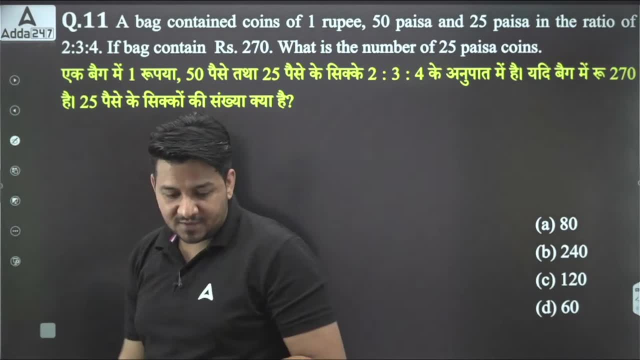 Yadi bag mein kul milaakar 270 rupee hai, toh 25 paise ke sikko ki sankhya gyat kiye. Kaise karenge bache aap iss question ko bohot dhyaan se dekho. 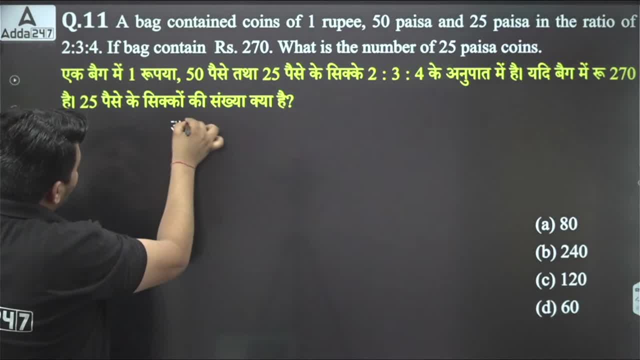 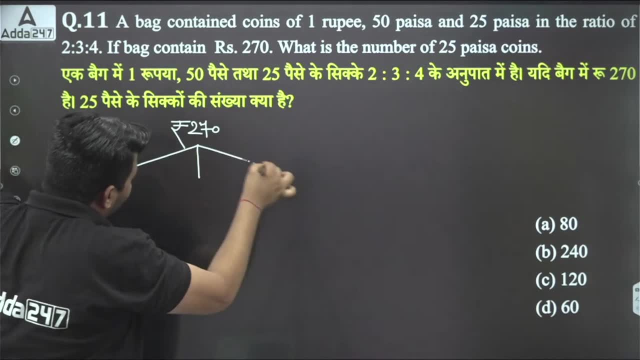 Hamare paas kitne rupee hai? Gurujee, hamare paas 270 rupee hai. Ab, ye 270 rupee bete 3 parts mein divide ho rahe hain. Dekho, iss mein se kuch 1 rupee wale hai, kuch 50 paise wale hai, kuch 25 paise wale hai. 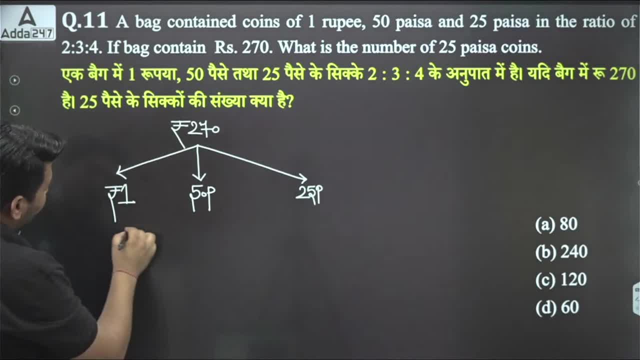 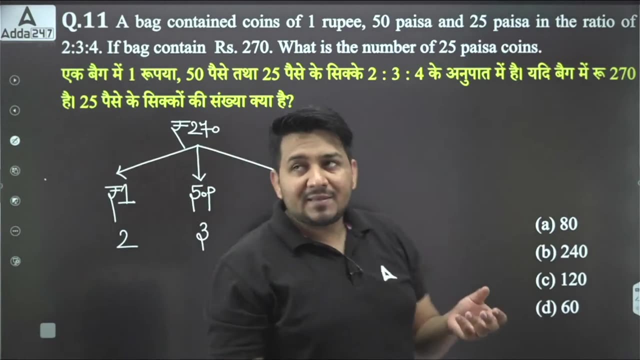 Bolo hai ki na Bag mein inka ratio kitna hai. Bag mein inka ratio 2, ratio 3, ratio 4 hai. Ab dekho, as a student humse puncha kya gaya hai ki sir, yeh batao ki 25 paise, kitne sikke hai. 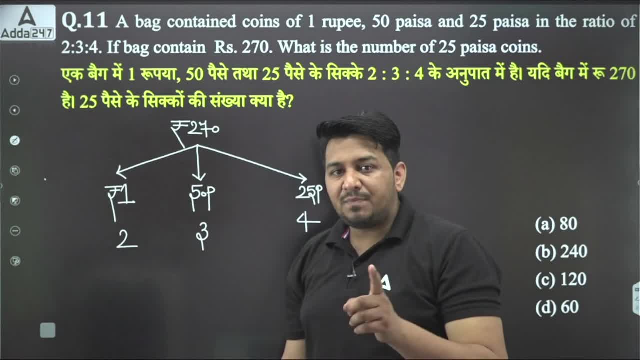 Aap kaise nikaaloge 25 paise ke? kitne sikke hai bache. ki kaise nikaaloge Isko nikalne ke liye? aap kya karenge? aap sabse pehle yeh dekho. 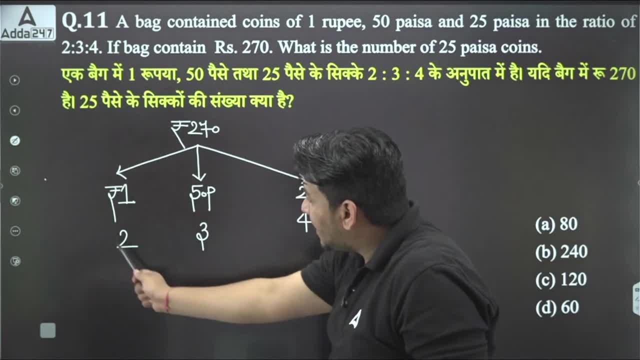 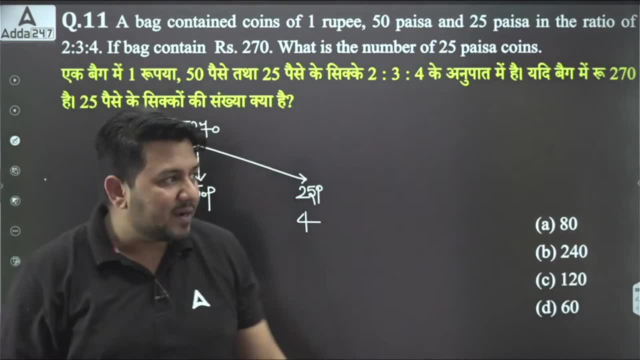 Aapka student mere dimaag mein kya aega ki agar main in sab ko add kardu, Agar bache main in sab ko add kardu to kitne rupee banne chahiye, Agar main in sab ko add kardu to 270 rupee banne chahiye. 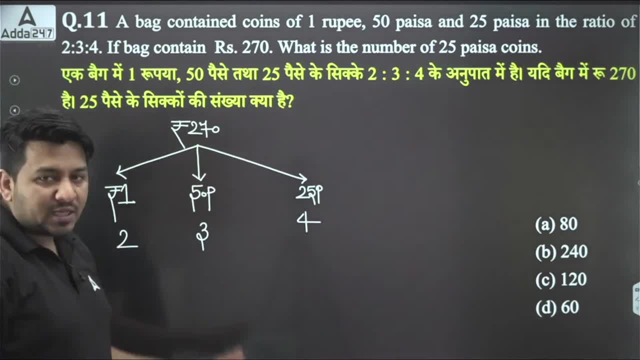 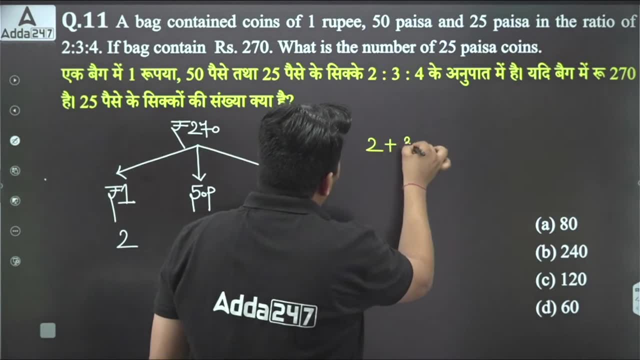 Bolo, agar main in sab ko add karunga, 270 rupee banne chahiye Bolo yes or no. koge sir bilkul add kardu To jaise hai. aap add karoge 2 plus 3 plus 4 value kiske barabar, 270 ke barabar. 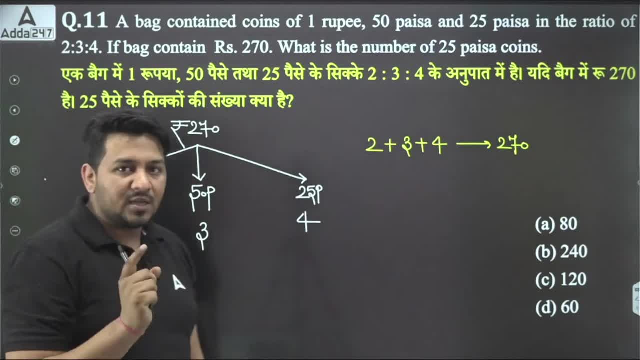 Hai ki nahi 270 ke barabar correct. hai, koge sir bilkul correct, Lekin choti se error hai. yeh rupee mein, yeh rupee mein, yeh dono paise mein. Agar yeh dono paise mein to inko rupee mein convert karo kaise? 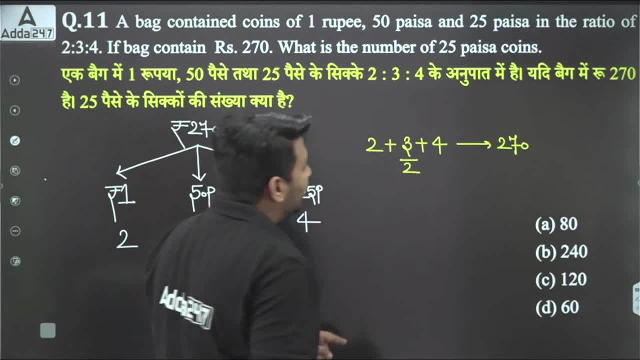 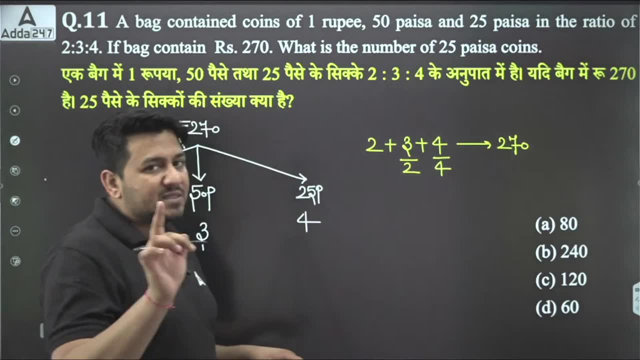 50 paise ko rupee mein convert karne ke liye. 2 ka divide karte kuki 1 rupee mein 50 paise ke 2 sikke hoten. 25 paise ko convert karne ke liye 4 ka divide karte kuki 1 rupee mein 25 paise ke 4 sikke hoten. 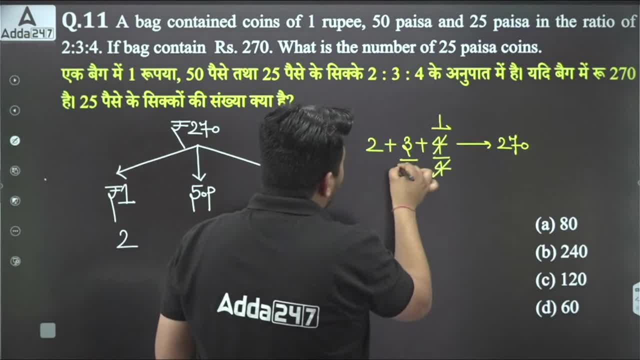 Cancel kardo kitni baar gaya, ek baar Yaha par cancel kardo kitni baar gaya 1.5 times. To yeh kitna hoge 2 aur ek 3 aur ek 4 sabko add kardo 4.5 unit ki value kitni hai. 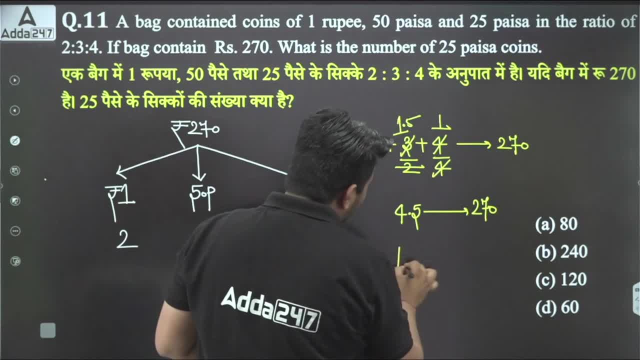 270 To yaha se ek unit ki value kitni aegi 270 divided by 4.5 To yaha se point hata do upar 0 badha do 9 se cancel kardo 9.45. 9 se cancel kardo 9.27 300. 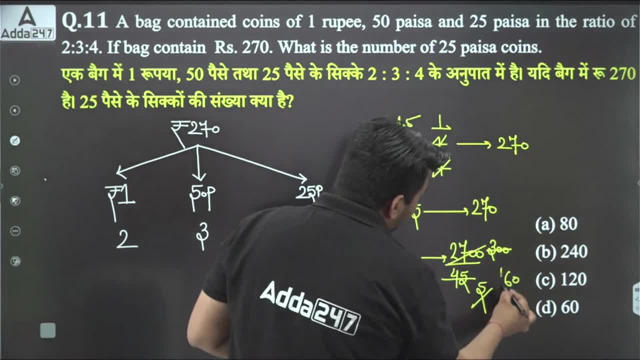 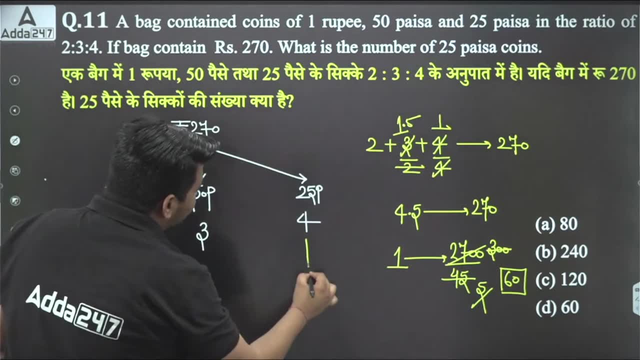 5 se cancel kardo kitna aga 5, 6, 30 hai nahi 60 Ek unit ki value kitni aegi bete 60. Agar ek unit ki value 60 hai, To kehra 25 paise kitne sikke into 60 kardo. 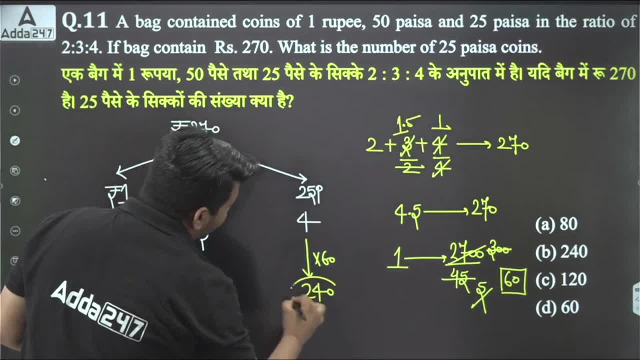 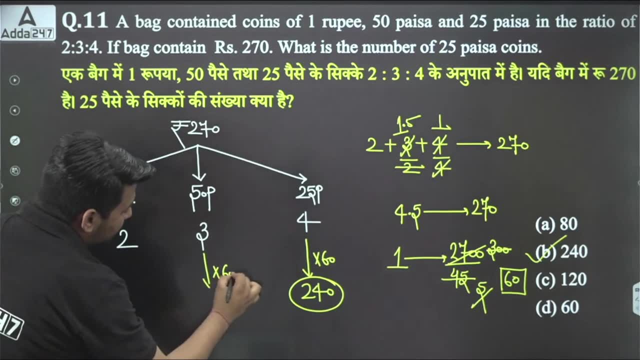 Yani 6, 4, 24, yani 240 sikke hongi. Aur yehi bache aapka answer hai: Agar aap se puch deta, 50 paise kitne sikke into 60 kardo, 638, 180 sikke hongi. 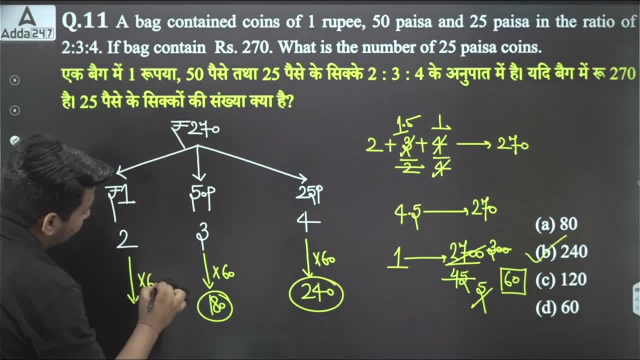 1 rupee ke kitne sikke into 60 kardo, Yani kitna hoge 6, 2ni 12, 120 sikke hongi Sabhi prakar ke sikke bete aapne nikal liye. 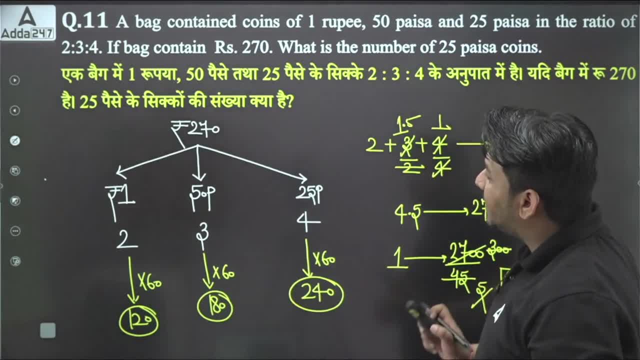 Sabhi prakar ke sikke bete aapne nikal liye. Sabhi prakar ke bache sikke aapne nikal liye. Bolo clear, kini clear. Sabhi prakar ke bache sikke aapne nikal liye. 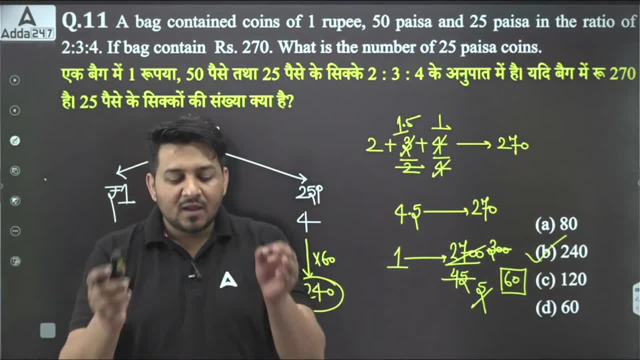 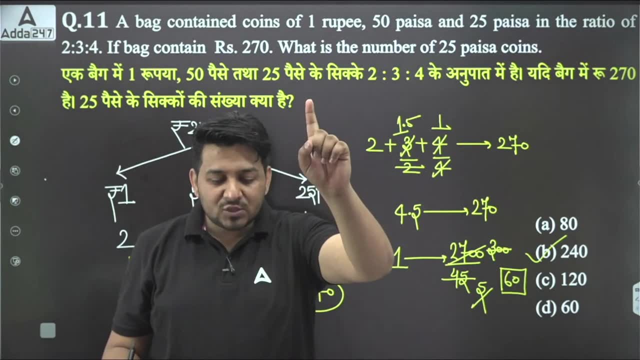 Appar clear hai. Sabhi bache bat te aper clear. Sabhi bache muje bat te aper clear. Sabhi bache bek karaike Bara saw plasta desh rahen Barha saw log ek sika like aur share karen. 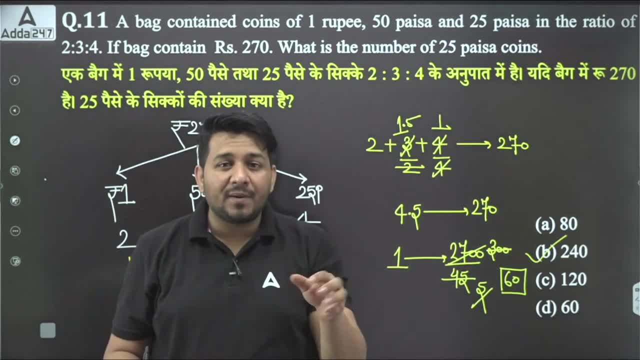 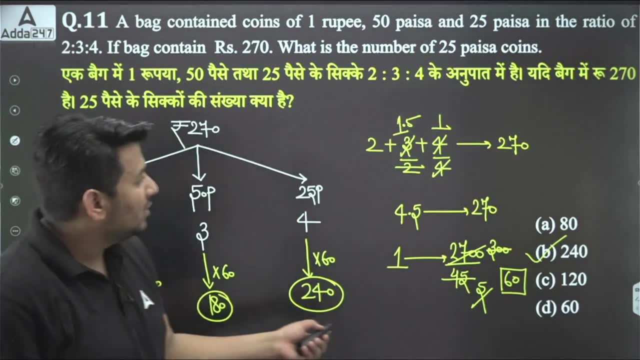 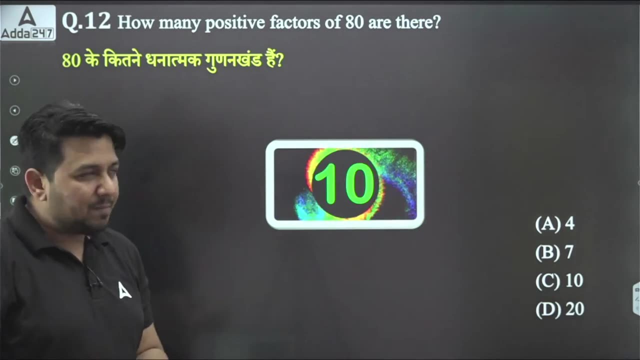 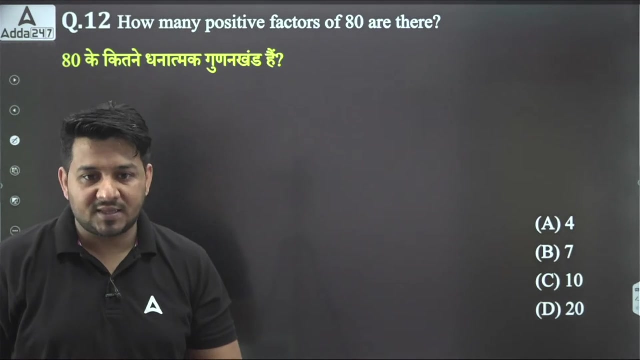 Akshay math guru telegram: apne telegram: Apar bache status ke formye share kar dete. Ek bar jaldi se share kardo. Ek bar jaldi se share kardo Apar jaldi se share kardo. Next question is in front of you. the same question was in your GD. I am talking about the paper of 10th January, which was last year- that how much is the wealth gap of 80,? how much is the wealth gap of 80,? that means the total number of positive factors. how will you find out? 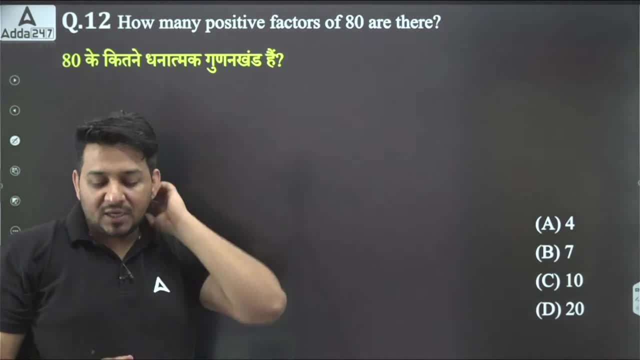 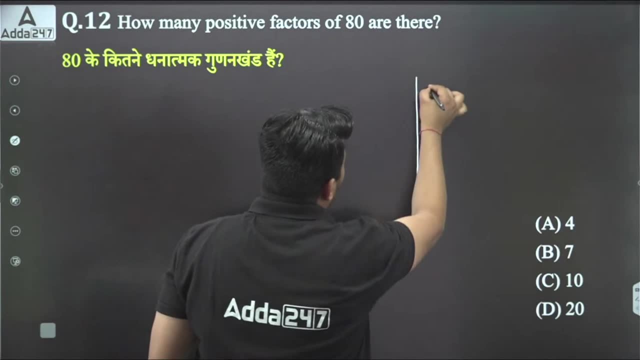 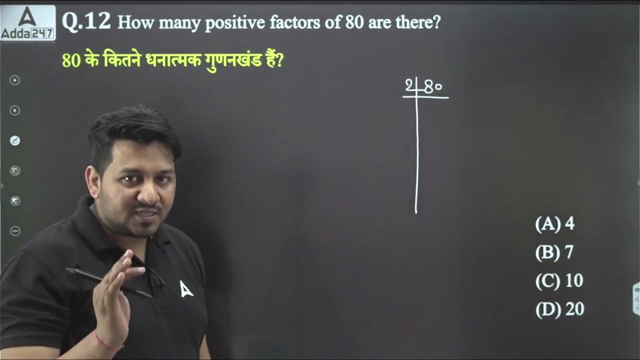 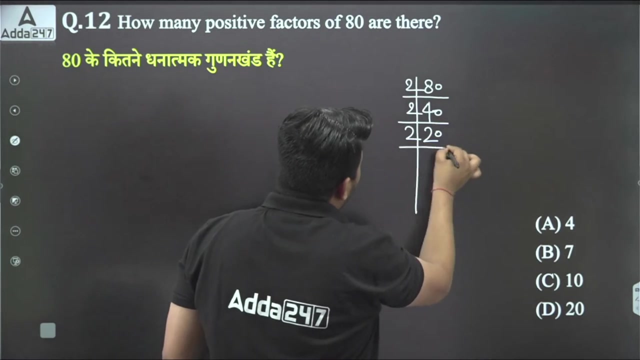 How will you find out children? First of all, tell me one thing: what can you write to 80, children? What can you write to 80, children? Either do 16,, 5,, 80 in your mind, or be careful, be careful, and be careful to avoid this thing. be careful. 40,. cancel from 2, 20,. cancel from 2, 10, cancel from 2, 5, and cancel from 5,. how much will it be? 1.. 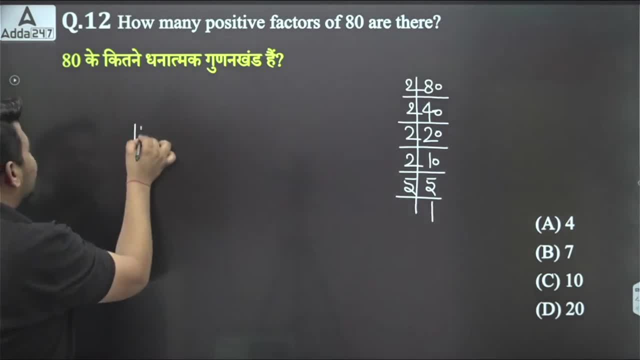 This is the next question. That means children. I can tell you what will you write to 80, children. What will you write to 80, children? What will you write to 80, children? What is the power of 2? 4.. 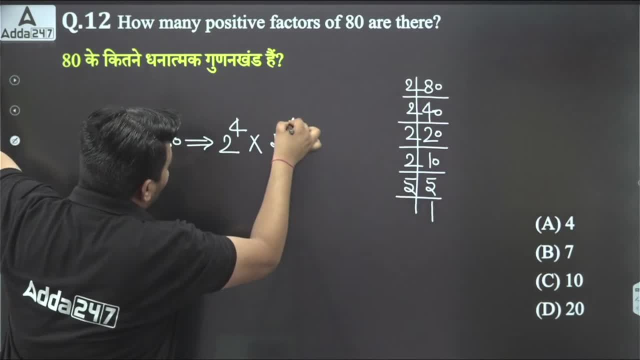 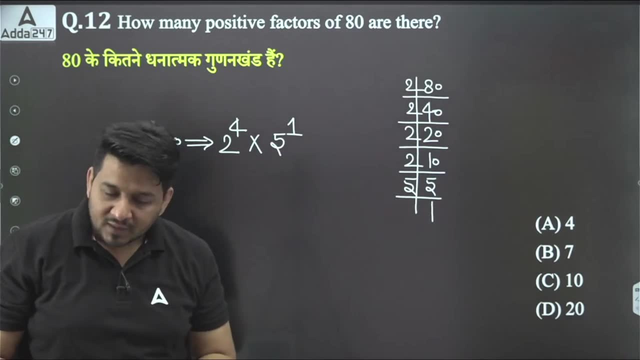 How much is the power of 5?? 1. This is done, Brother. will you write to 80? here? 80 means children. the power of 2 is 4 and the power of 5 is 1.. Clear. 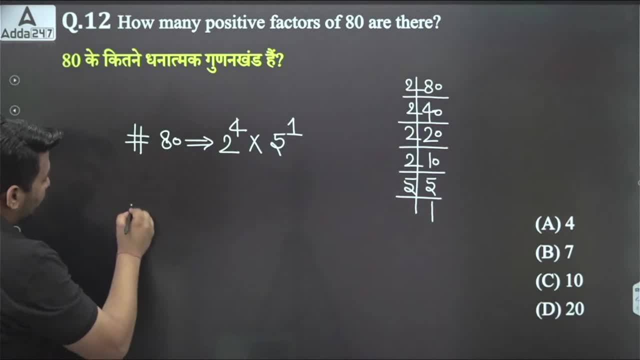 Now, what was the question? The question is: what is the total number of factors? What is the total number of factors? How will you solve it? Whenever I talk about the total number of factors, for example, how much is the power of 2, 4?? 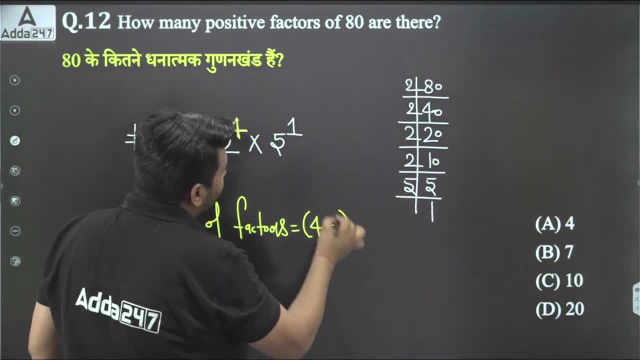 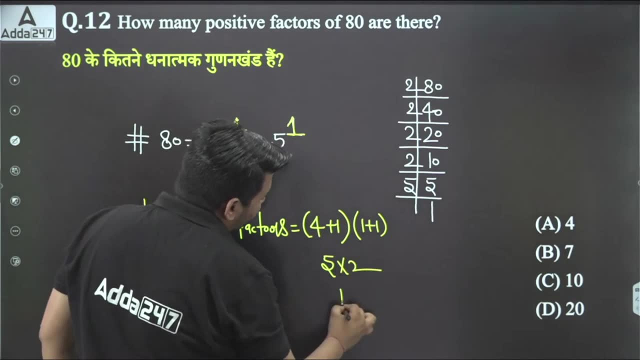 How much is the power of 2?? I write it as 4, plus 1.. How much is the power of 5? 1. So, children, we will write it as 1, plus 1.. That means 5 times 2,, which is 10.. 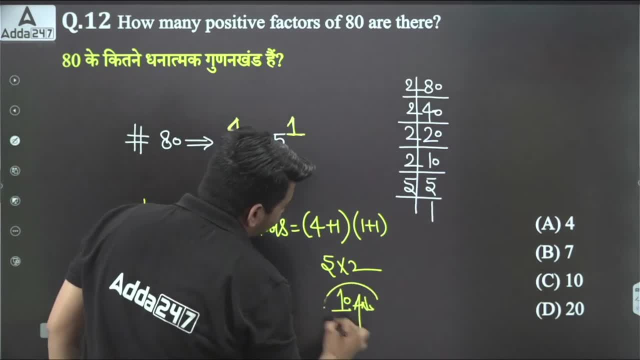 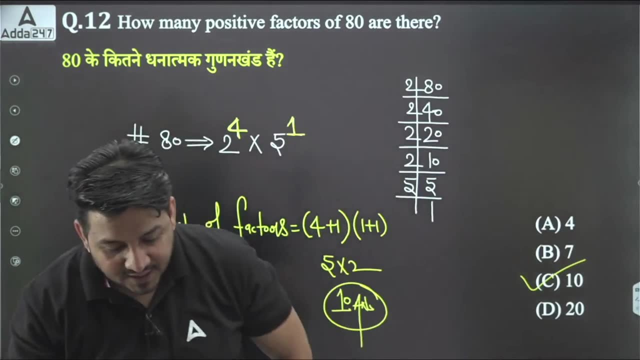 What are the 10 children? There are the number of factors. What are the 10 children? There are the number of factors. Option no C. What are the 10 children? There are the number of factors. Option no C. 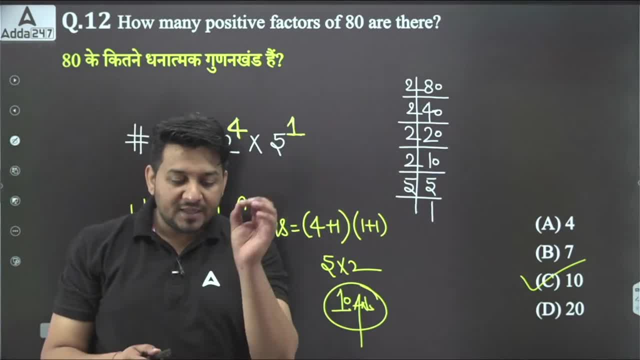 The video is getting stuck, sir. I have seen it. son, You guys manage for a little while. Right now. I am calling my technical team immediately. Don't worry, This does not happen in my class. Yes, Be careful. the accident has happened. This is the thing, absolutely. 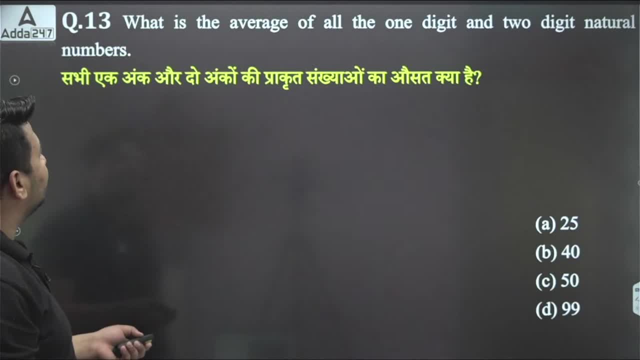 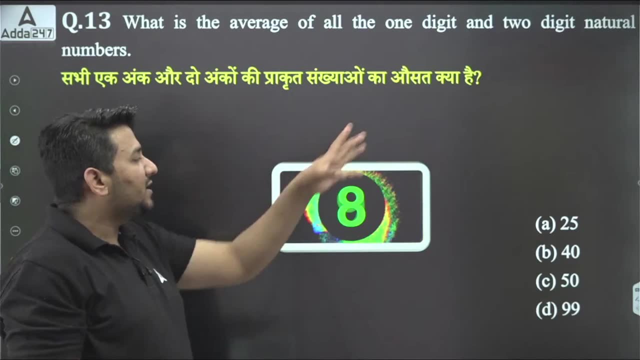 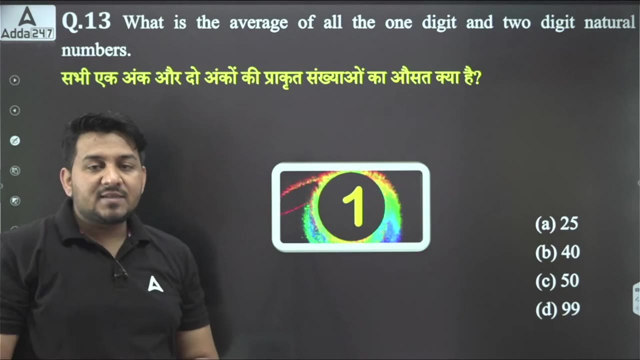 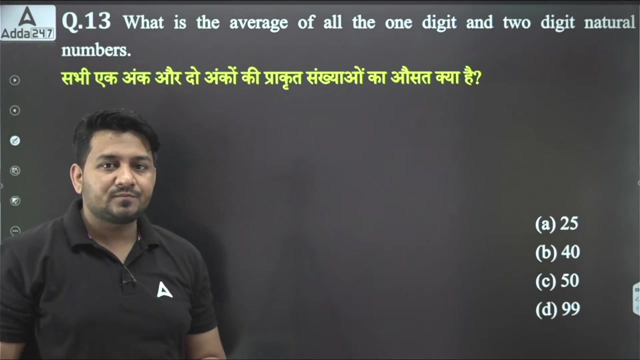 Once all of you share it. The next question, kids, is in front of you, Very important kids. The question says: what is the average of all one-digit, two-digit natural numbers, Son, how will you do it, Son, how will you do it? 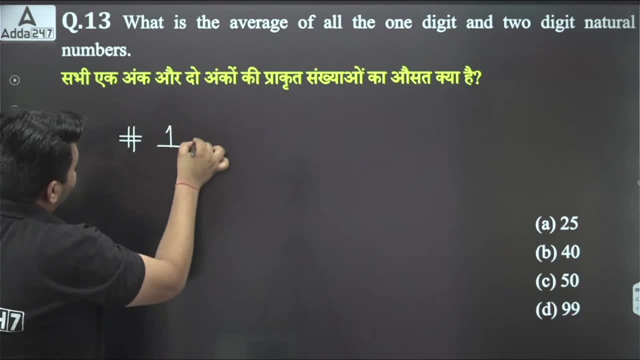 Look first of all one, Then how much is two, Then how much is three, If we go in this way, kids, then how much is three, How much is three, Ninety-nine? To what extent did he go? 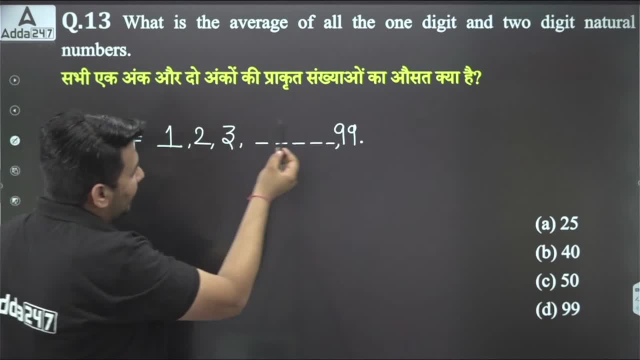 He went to ninety-nine. If I am writing numbers from one to ninety-nine, watch carefully. If, kids, I am writing numbers from one to ninety-nine, then it means that all one-digit and two-digit numbers are included in this. Say yes or no. 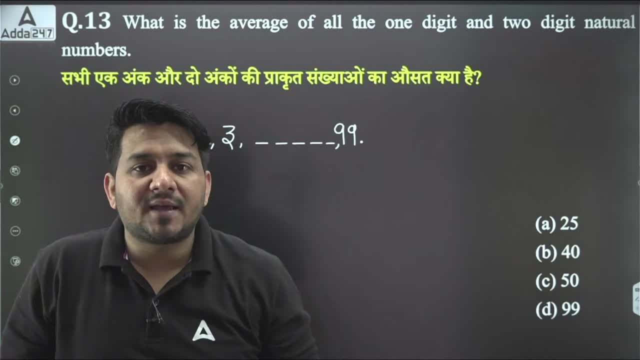 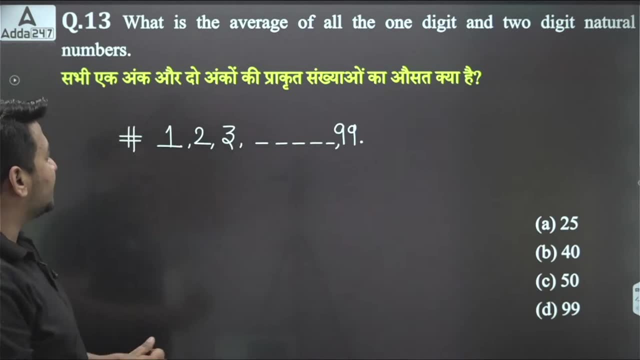 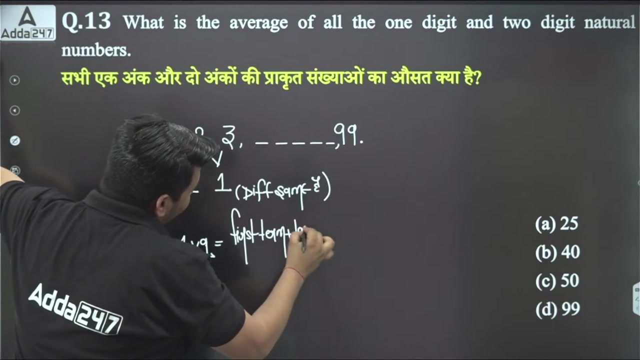 Kids. I have written numbers from one to ninety-nine. So this means that there are all one-digit numbers in it and all two-digit numbers, Isn't it? There is also a number of two digits. tell me if there is or not. tell me if there is or not. how much is the difference? here? it is one. here, the difference is one. tell me, how is the difference? how is the difference? what is the difference? it is the same. how much is the difference? it is the same. when I teach GD, my feelings are connected to it. how will we get the average? the way to get the average is first term plus last term, divided by GD. 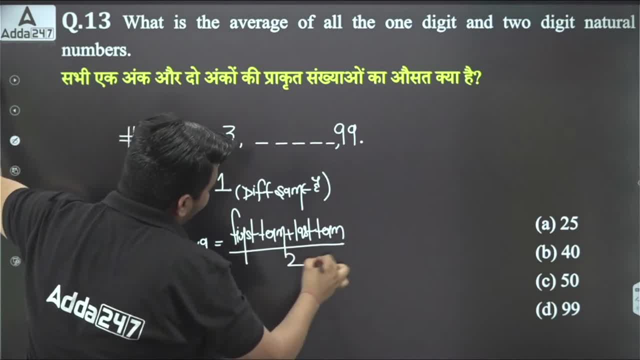 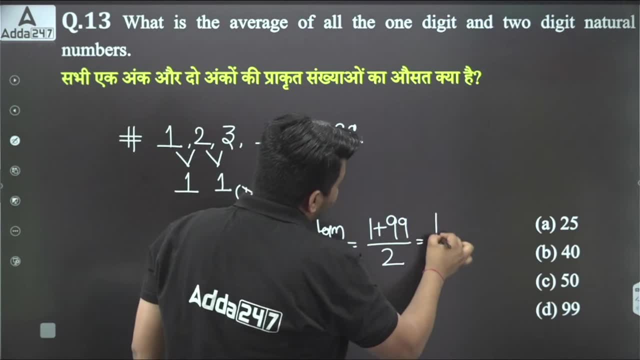 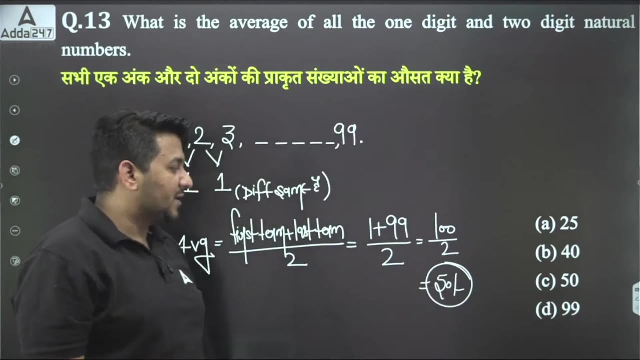 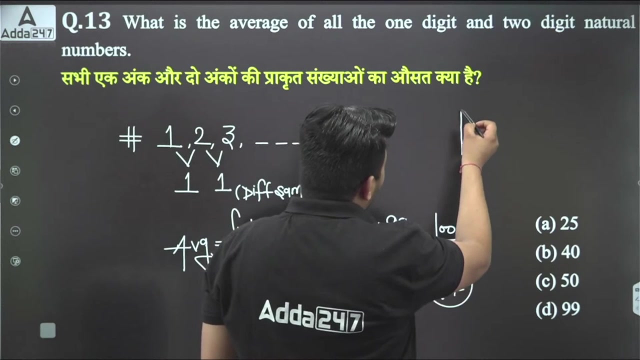 divided by two. first term plus last term divided by two, how much is the first term? one, how much is the last term? 99 divided by two, that means 100. divided by two, that means how much will it be? it will be 50,. it will be 50, it will be 50,. you know why my feelings are connected to GD. when I started studying, I used to study from my home, so the first three children used to come to me in the form of home tuition. I used to teach them math. 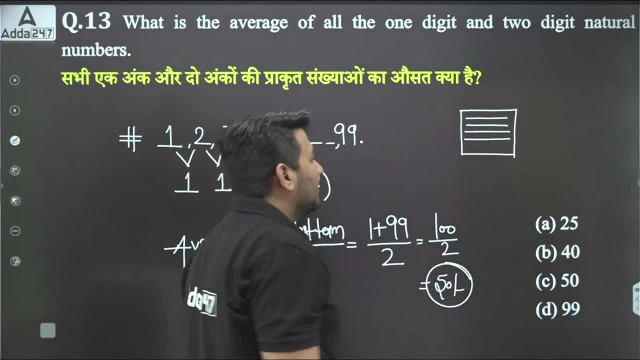 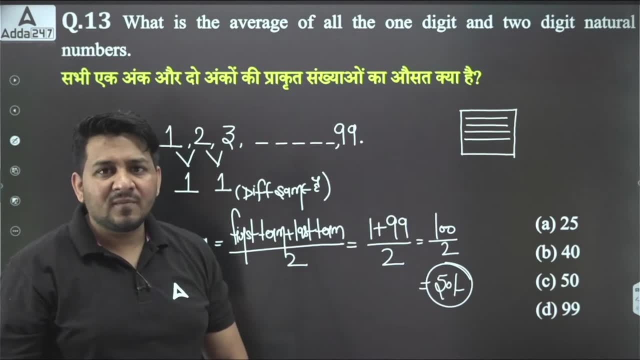 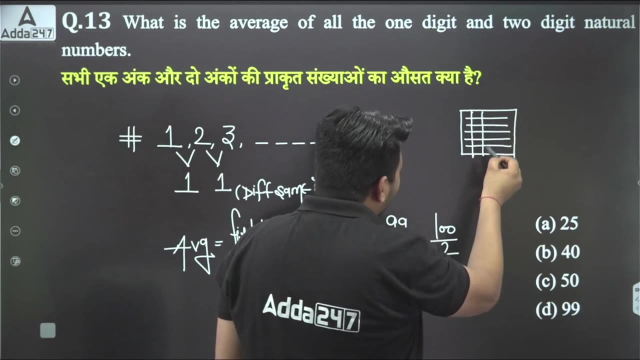 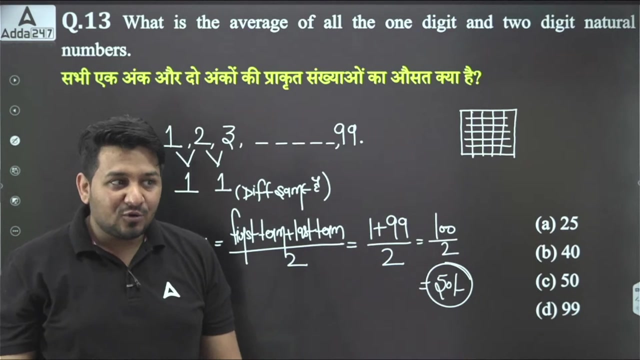 reasoning. I used to teach them all the subjects and among those three, even today, some are connected to Facebook. two children are on Facebook and you will see. you will also find their photo wearing the uniform. those three were my first students who were selected in GD and even today they are in my touch and I taught them math and reasoning. then I taught something. 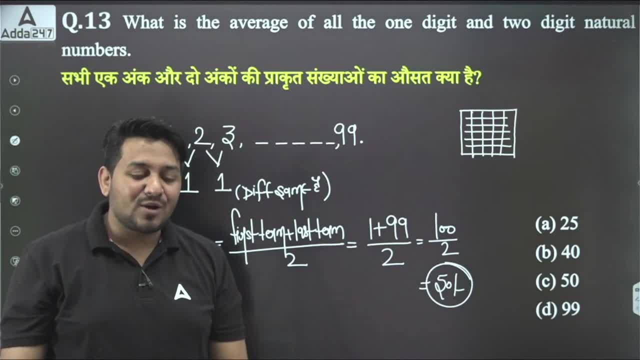 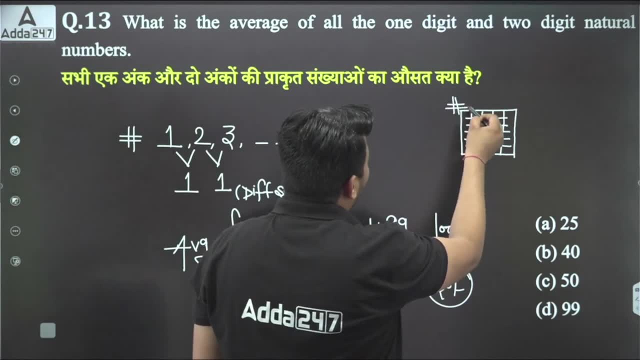 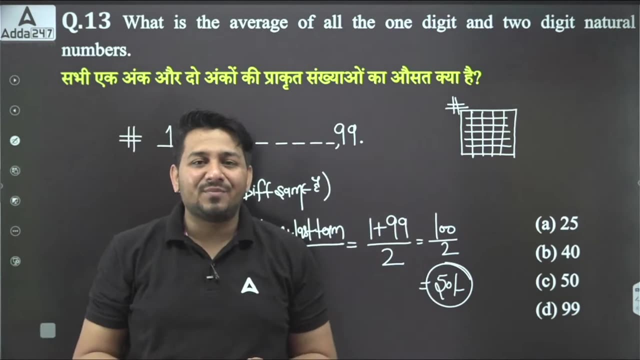 so GD is a very old relationship of mine, GD, and after that Astosh sir came. okay, our whole team kept on becoming, and gradually, in an excellent way. I got your support, I got your love. the last playlist I have, son, it has millions of views, millions of views. it means my heart gets happy to see your love. 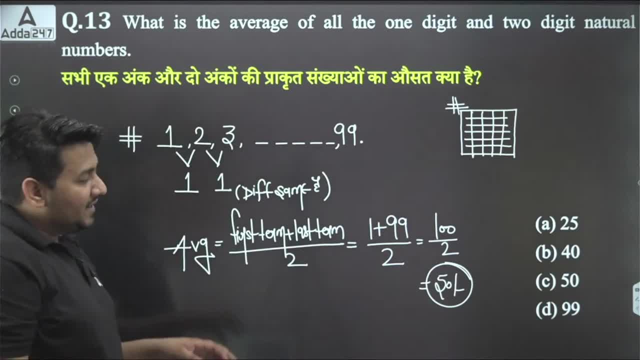 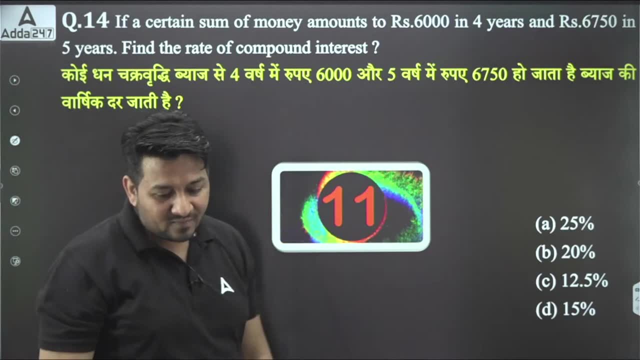 let's move forward, let's move forward, let's move forward. next question: tell me, I did it yesterday and this same question, son, has come to your exam. yesterday I did this type of question in the class of compound interest and the same question, children, has come to your exam. tell me, tell me, what will be the answer to this question, quickly, quickly, quickly. 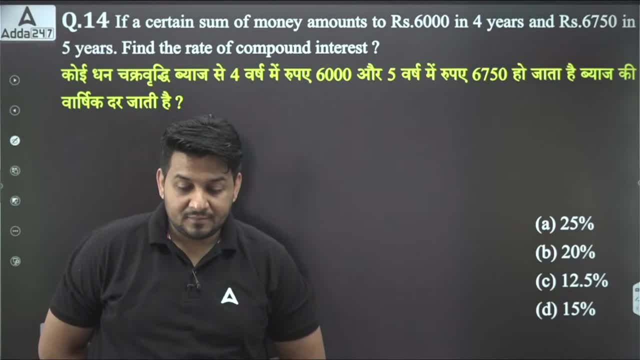 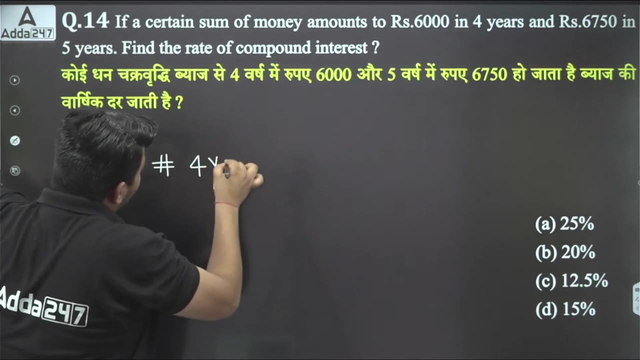 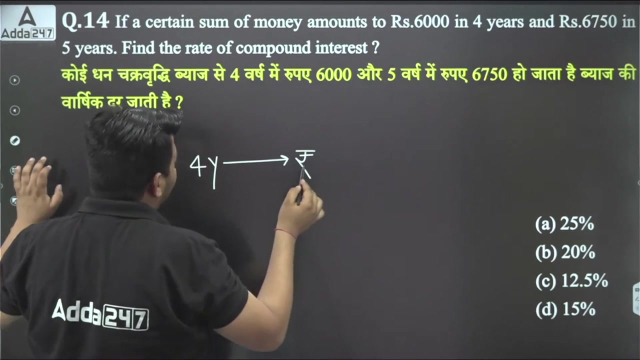 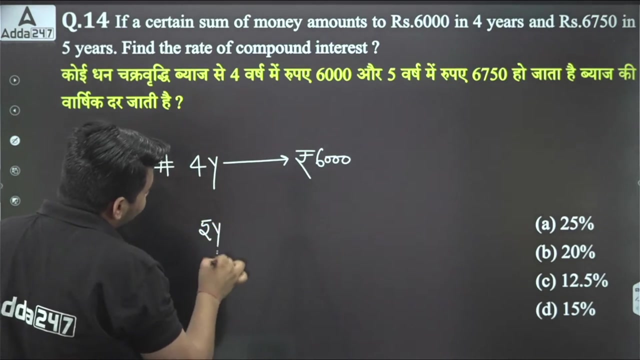 how will the prime factor of 80 be 10,? son, let me tell you right now how will you get the prime factor of 80, see what the question is saying. on any financial interest in four years, doesn't matter any money. on World Index interest in four years: six thousand rupees in four years, my son, six thousand rupees. six thousand rupees in four years and five years, five years, six thousand seven hundred fifty rupees. 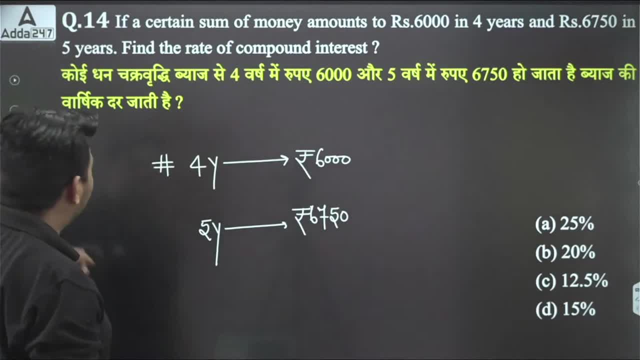 Six thousand seven hundred fifty rupees becomes mention the annual interest rate. look, it is 6000 in four years And in 5 years there is 6750. Remember the annual interest rate of the interest: See 6000 in 4 years. 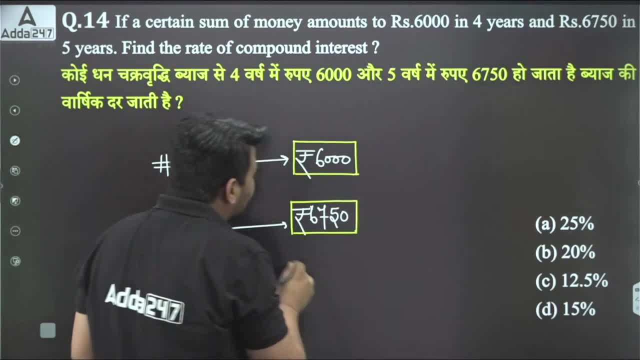 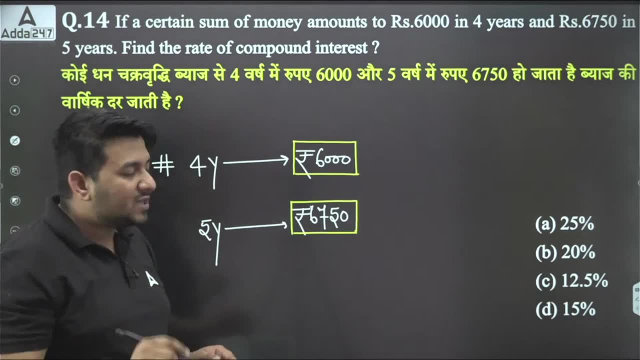 And what is 6750 in 5 years? Consecutive years have been given. See, It is the annual interest rate. It is the annual interest rate children. If it is the annual interest rate, Then 6000 rupees in one year Convert to 6750 rupees. 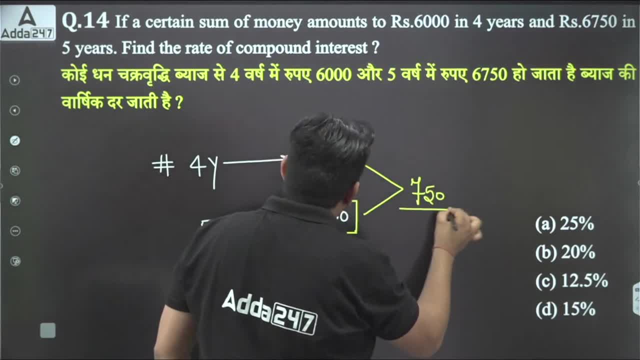 That means 750 rupees. is your interest How much on 6000 Convert to 100? This went from this. This went from this. Okay, Cancel from 3 times 25 times. Cancel from 3 times 2 times 25 divided by 2 means. 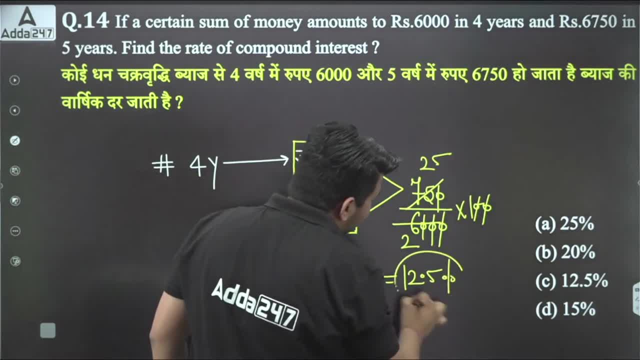 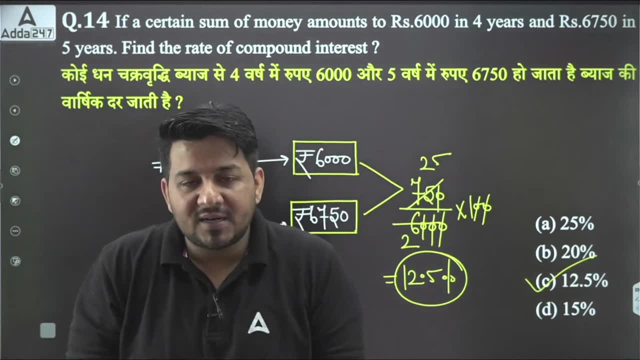 12.5%. 12.5% children is your rate. 12.5% children is the rate of interest. Is it clear or not? All children share. once 1200 people live, All children share. Come on, Share quickly. Next question, Next in front of you. 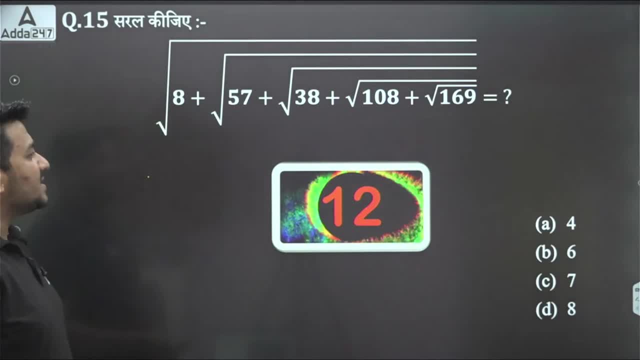 Tell me. See, Many students will try to answer this number by just looking at this number. I will say to you: Don't make such a mistake, Because sometimes There is a square root in the middle. If there is a cube root, Then the chances of questions Making a mistake in different ways. 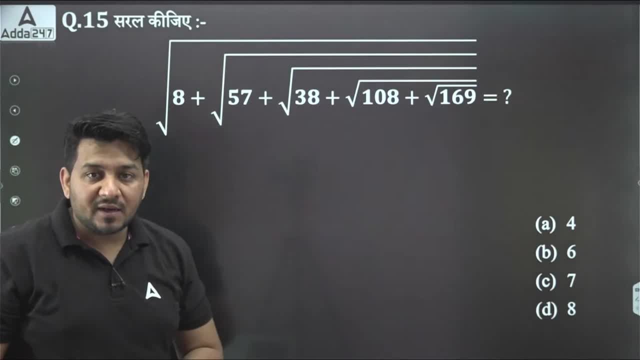 You have increased. Always remember, Whenever this question comes, Only one trick, Only remember one concept: Always make the question from here. If you make the question from this side, Then from this side. Just remember: Make the question from this side. Remember: If you make the question from this side, the chances of making a mistake are 0%. 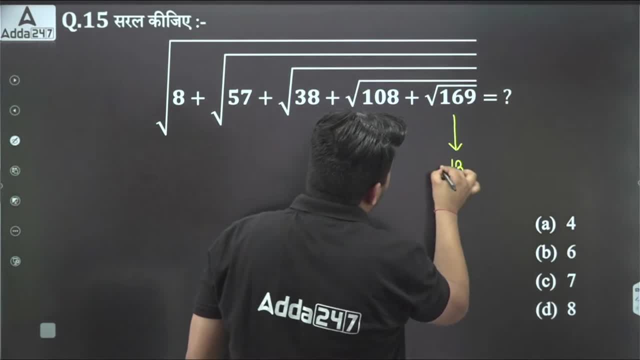 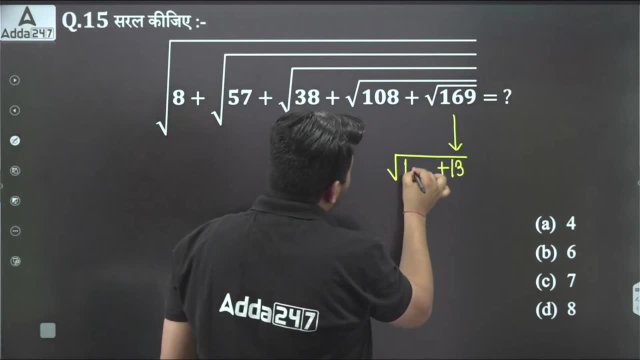 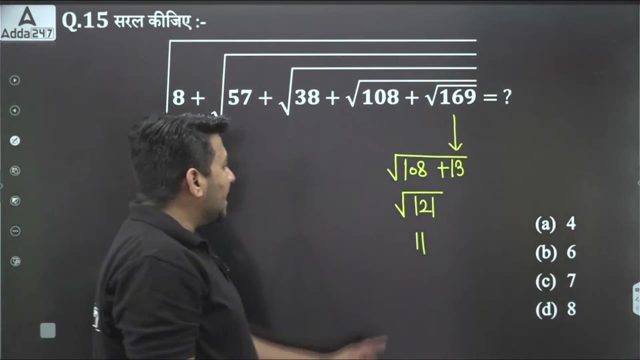 Under root, 169 will give you 13.. And this 13 will be connected to 108.. Under root, 121 will give you 11.. 11 will be connected to 38.. When 11 will be connected to 38, it will be 49.. 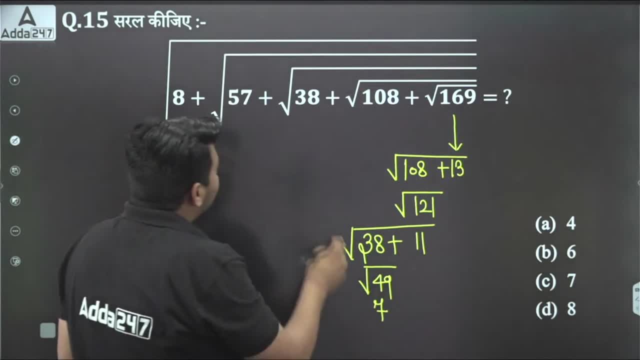 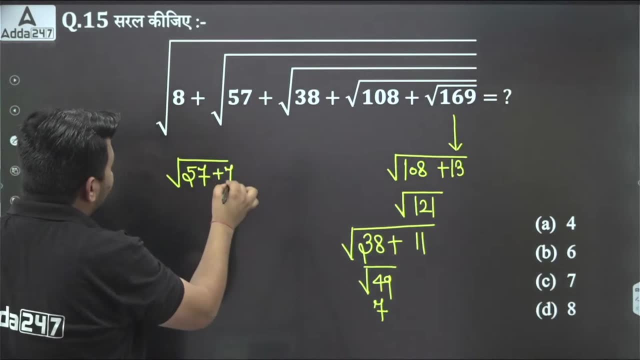 And 49 will give you 7.. This 7 will be connected to 57.. This 7 will be connected to 57.. 7 plus 57 will be under root 64.. Under root 8 will be connected to 16.. 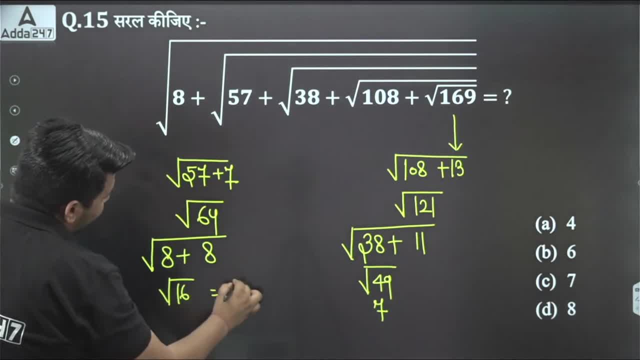 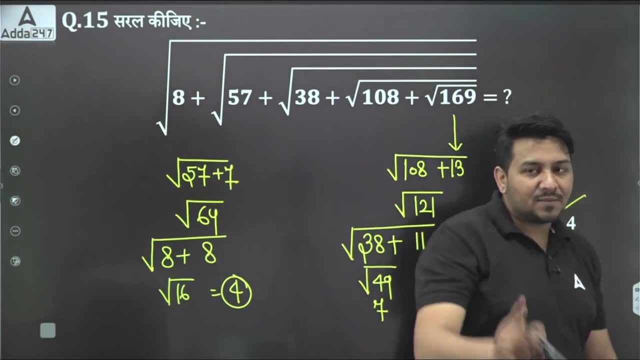 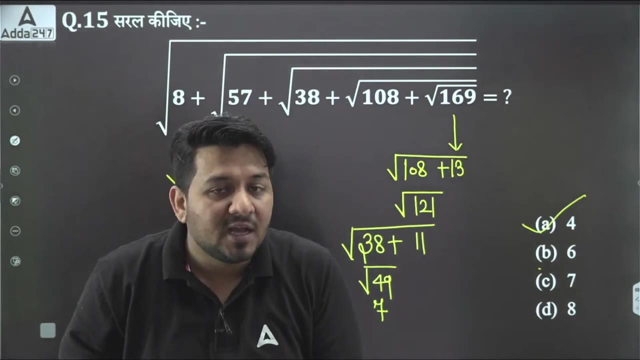 Under root 16 will give you 4. And some people will give 8.. You can see clearly: If 3 was also available in the option, children would have answered 3 most often. If there were 3 in the option, then they would have answered more, because people who answer based on it, they have the biggest problem. 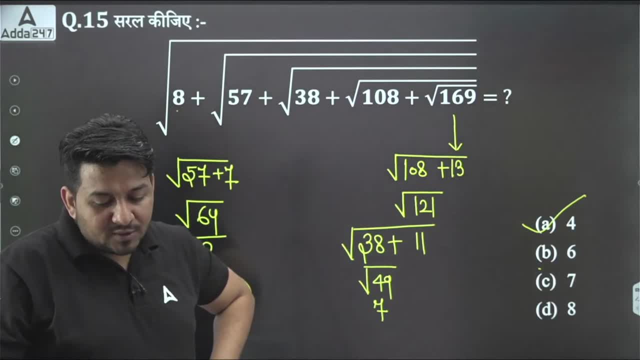 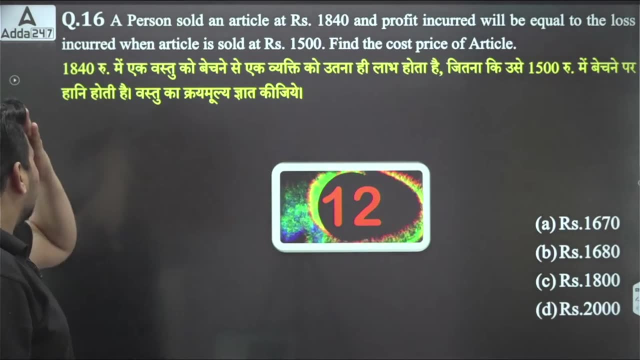 Tell me, does it happen? I can understand very quickly. Yes, sir clear. All children say yes, sir, clear. Next question is in front of you children, Very important. What is the question saying 8. If you sell it for Rs.1840,, one person will get the same profit as if you sell it for Rs.1500,. the loss 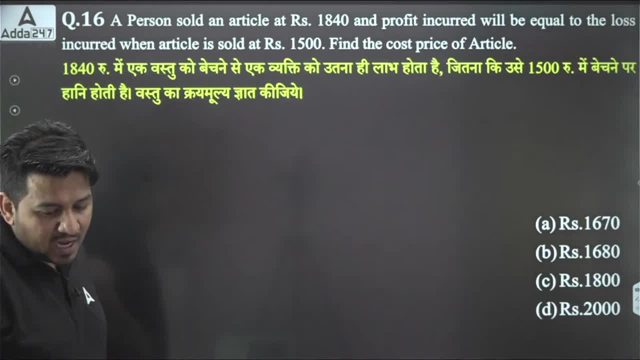 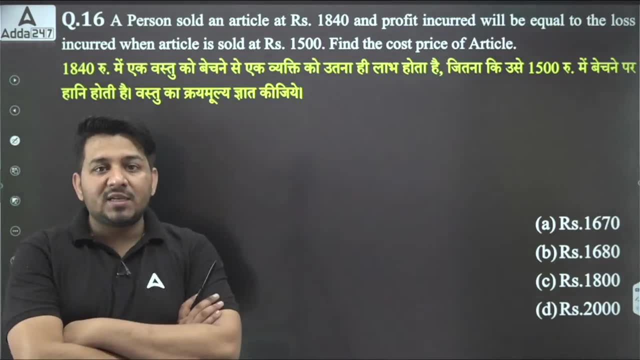 Find out the price of the item. find out the price of the item. tell me quickly. The question is: what is the profit of selling it for Rs.1840, as compared to the loss of Rs.1500?? So tell me what is the cost of selling it for Rs.1500?? 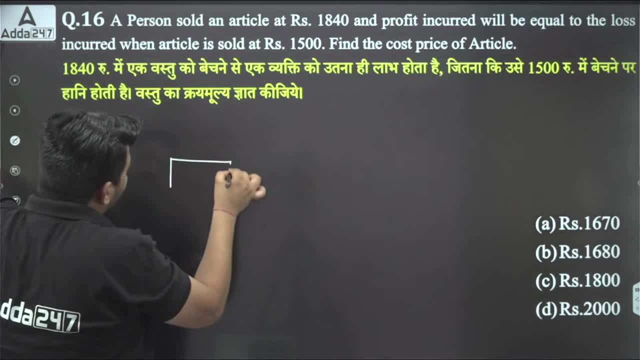 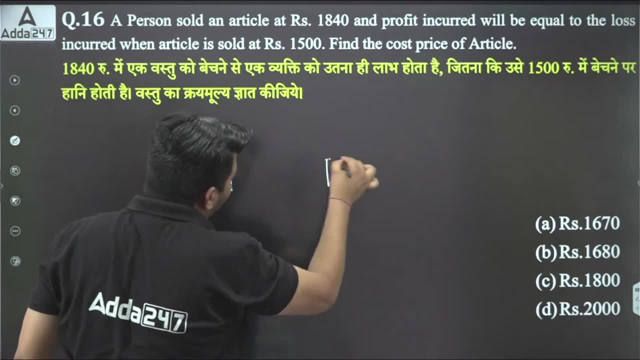 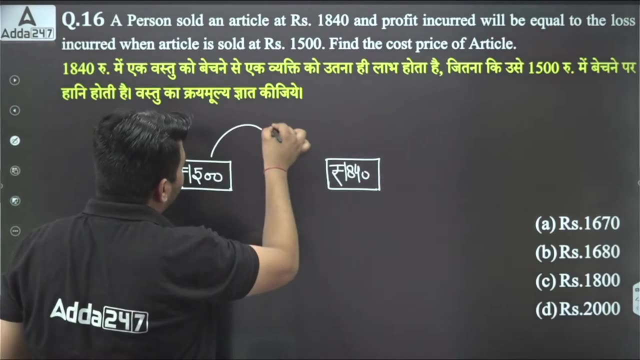 What is the loss of selling it for Rs.1500?? What is the loss of selling it for Rs.1840?? What is the profit of selling it for Rs.1840?? The cost has been asked. The cost is here in the middle. 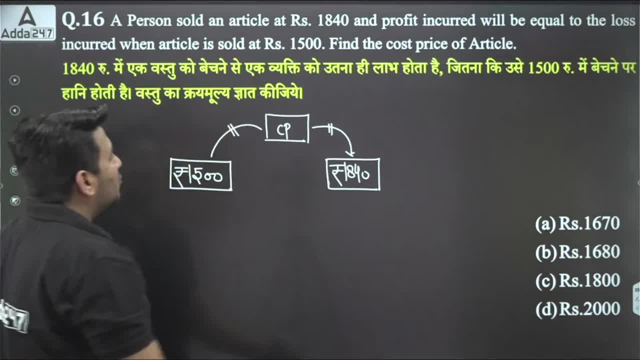 And what is the loss and profit? They are equal. How will you find out the cost? How will you find out the cost? Remember, I will explain the trick of this to you. Whenever such a question comes in front of you, you should be asked the cost. 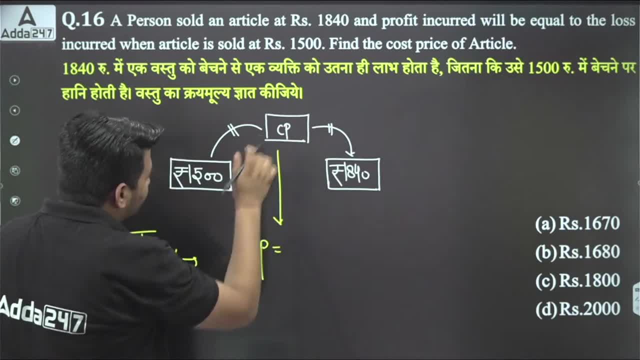 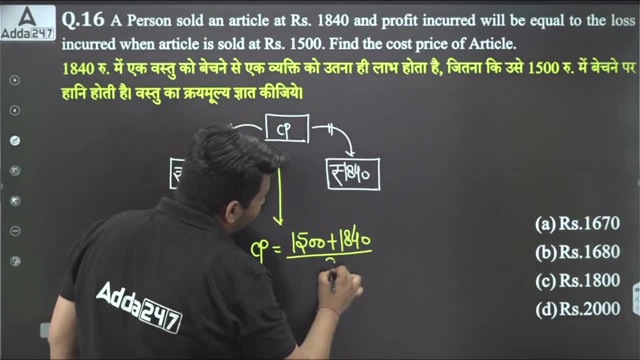 The cost is always the value between these two. That is, the value between these two. How do you find out the value between these two? Rs.1500 plus Rs.1840 divided by 2. How much is it Zero? 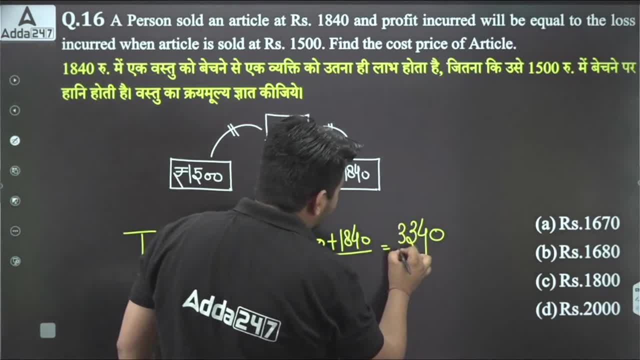 This will be 4.. 8 plus 5 is 13.. Carry 1.. Rs.3340 divided by 2.. 2 is exactly 2.. 13 is 12.. 14 is 274.. 1670.. 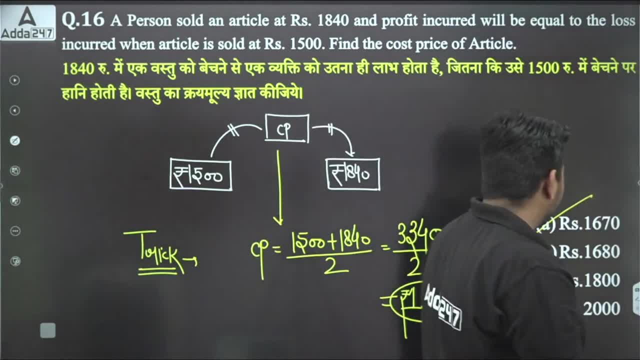 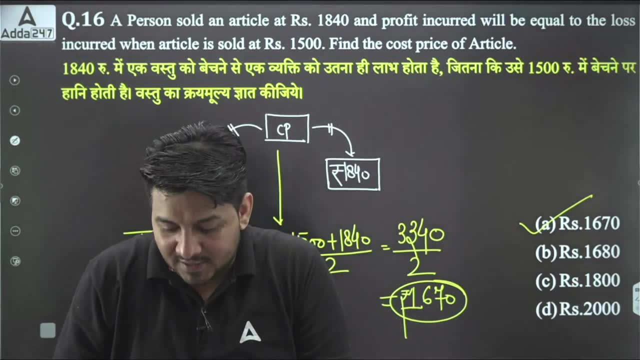 1670.. How much will it be Rs.1670.. Rs.1670.. Tell me, is it clear or not clear? Rs.1670.. How much will it be Rs.1670.. What is the correct answer? 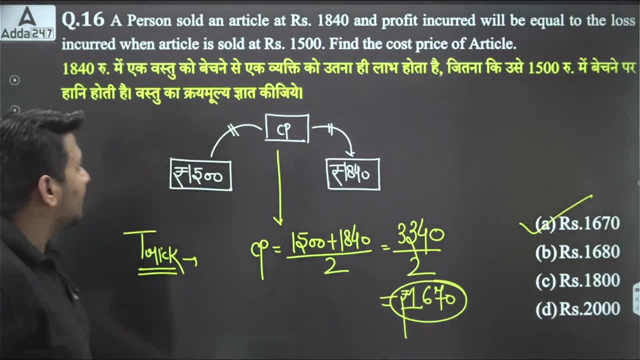 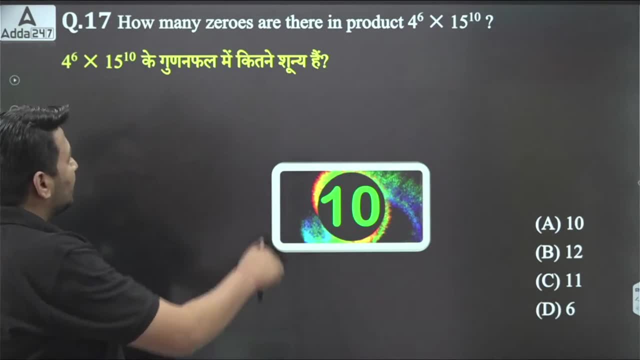 Tell me, is it clear or not clear? All children tell me: is it clear? Next question is in front of you. It says: what is the number of zeros in the quality of 4 power 6 and 5 power 10?? 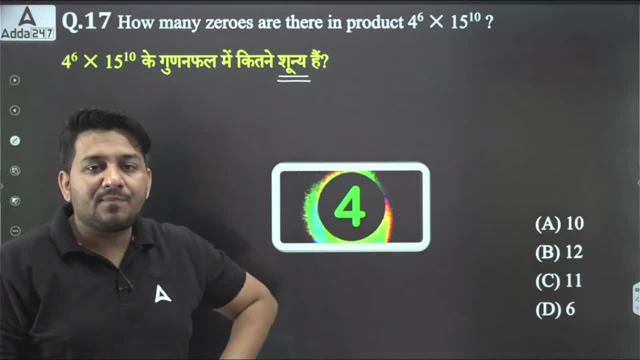 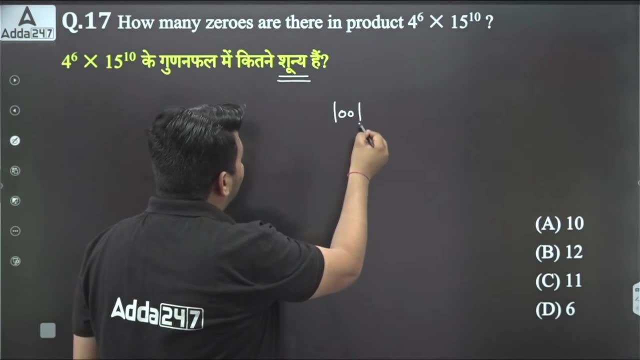 What is the number of zeros? You must have read this question. You will always see the question like this: Tell me, tell me how many zeros are written in 100 factorial. Or suppose it will give 500 in this way? 400, 599.. 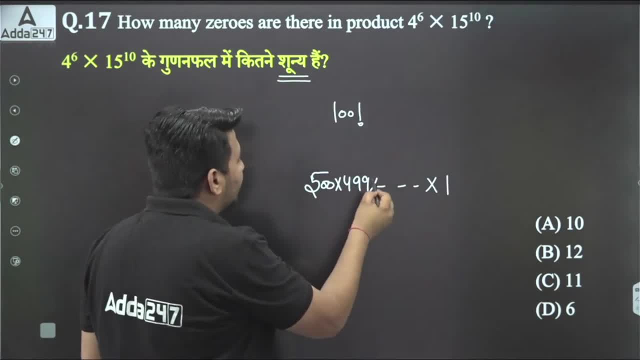 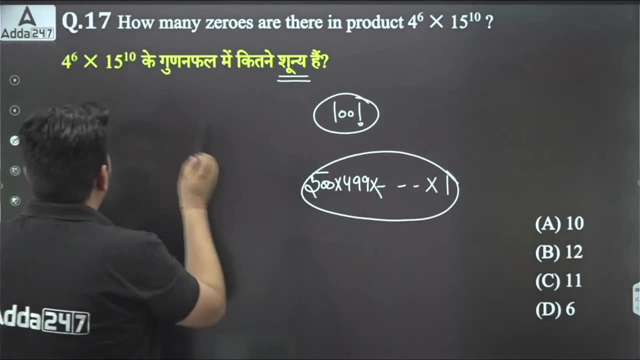 It will give up to 1 in this way. Tell me what is the number of zeros. But children, now the question asks in this way. It will ask this way. But now the new pattern is that the question has started asking questions in this way. 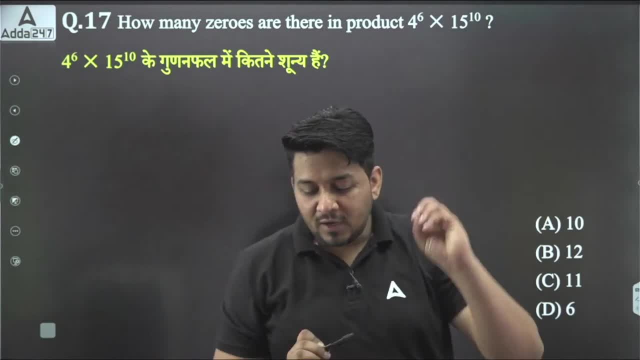 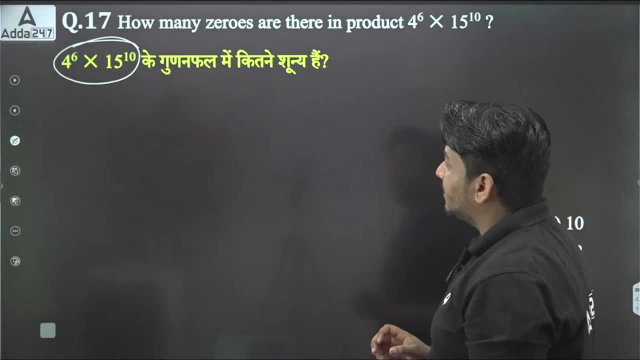 Tell me how will you find it? This is a totally new way of question. The question is asking questions in this way. on the new pattern, Tell me what is the number of zeros? If I multiply these, Then what is the number of zero? 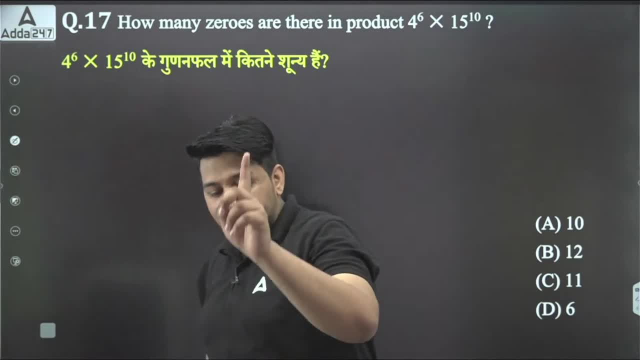 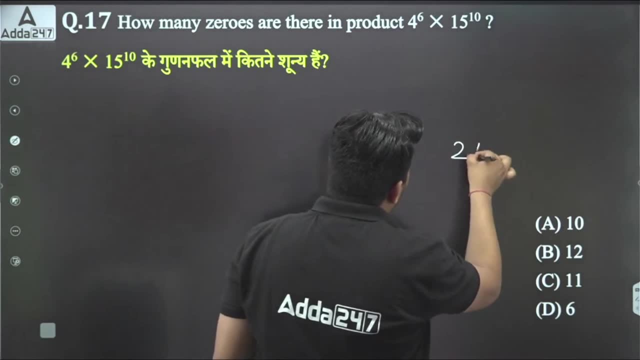 So don't move from the concept, The concept I have taught you. If you know the concept, then you can't do anything wrong in your life. See, When does zero become? Whenever we multiply 2 by 5, Then zero becomes. Zero becomes from 2 and 5. 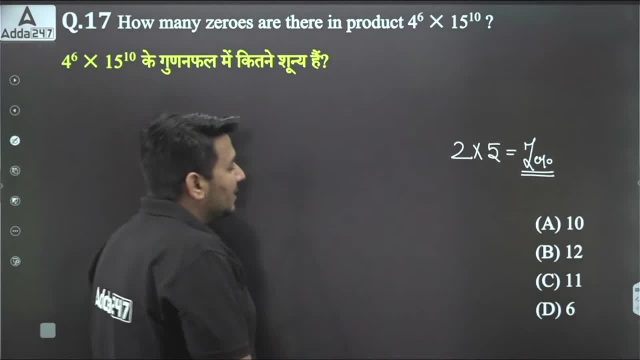 Tell me, is it or not? Did I teach you Zero becomes from 2 and 5? Tell me yes or no, The number of pairs of 2 and 5. That's how zero becomes. Tell me yes or no. Now look very carefully What will you write? 4?. 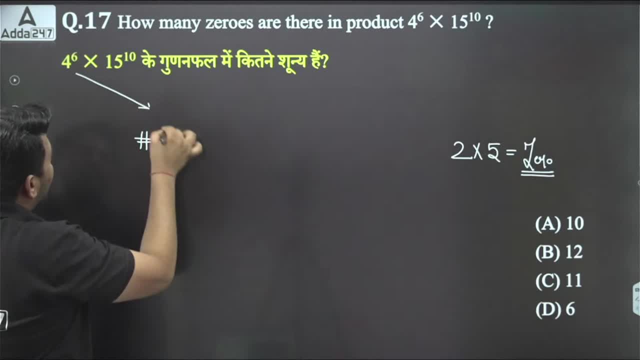 Guruji, What did we write? 4? I wrote 2 to the power of 2 And 6 to the power of 15. What did I write 15? I wrote 15 as 3 times 5. How much is the power of 10?? 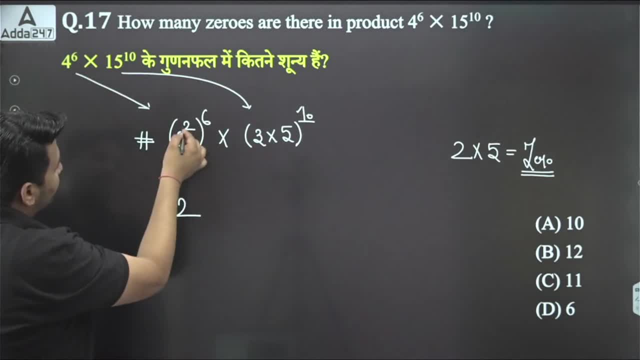 I wrote this. Now see How much power does 2 have. 6 times 12. Okay, This 10 power, This power, This will come on this too. This 10 power will come on this too. So this will become 3 to the power of 10. 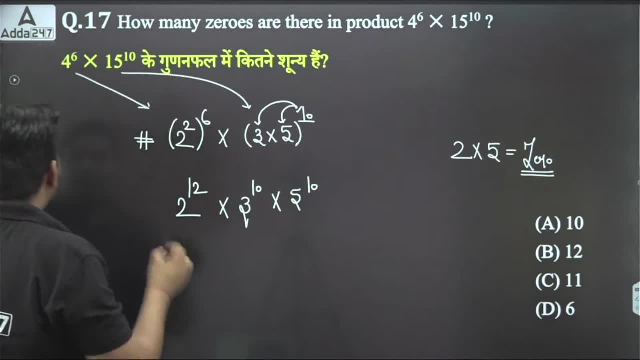 And 5 to the power of 10. Tell me, is it or not? Now tell me, How much is 2?? See, This has no relation to zero. Okay, Okay, Here look. 2 to the power of 10 And 5, 2 to the power of 12. 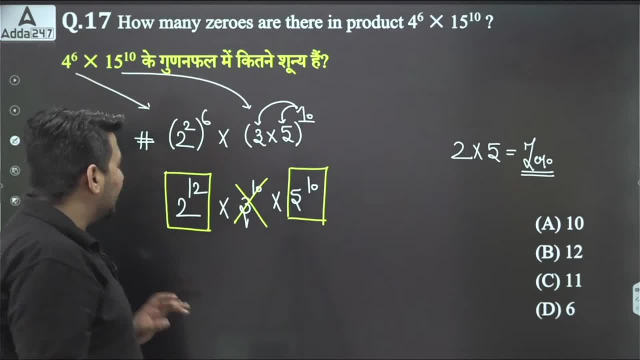 5 to the power of 10. This does not come in zero. Leave it, It doesn't mean anything. How many times is 2? 12 times? How many times is 5? 10 times? So how many pairs will become 12 boys, 10 girls? 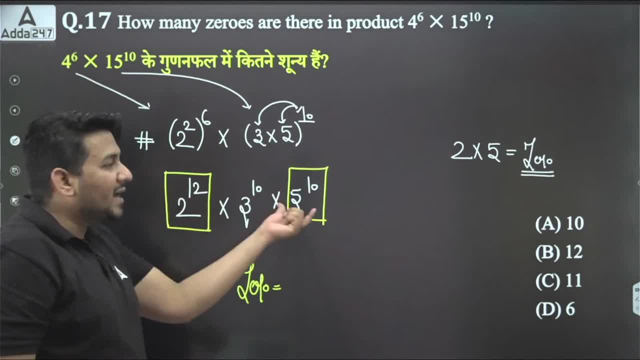 How many weddings Use your money to make pairs? How many pairs will become? Because, sir, 12 boys, 10 girls, How many pairs will become? 10 pairs will become And all pairs will become Same number of zeros. So how many zeros will become? 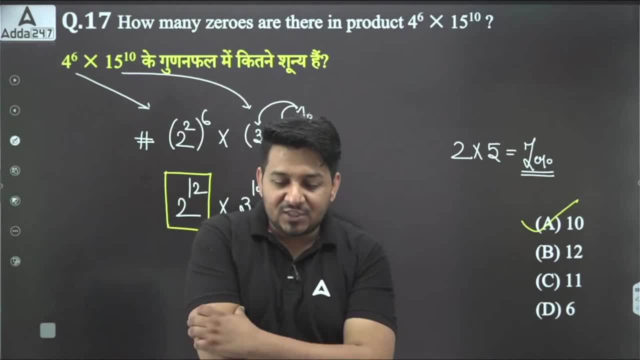 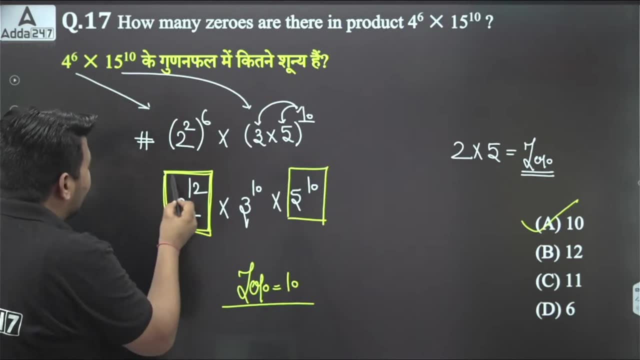 10 zeros will become. How many zeros will become? 10 zeros will become. There is no confusion, No confusion. Look: How many times is 2? 12 times. Assume there are 12 boys And here the power of 5 is 10. How many boys are there? 10 boys? 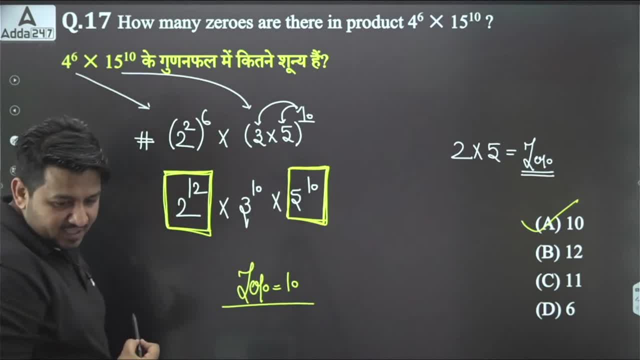 So how many girls can there be? How many pairs will there be? Only 10 pairs will be made, And the number of pairs that will be made? The number of pairs that will be made Will be zero. The number of pairs that will be made of 2 and 5. 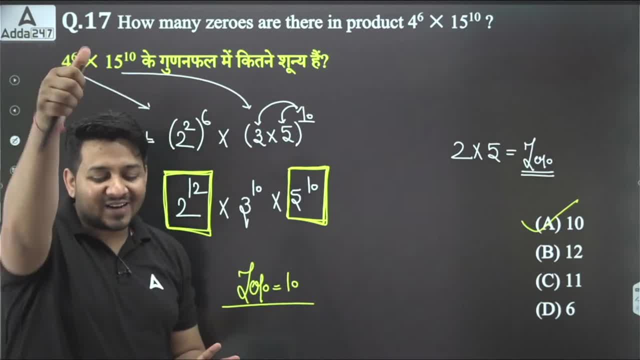 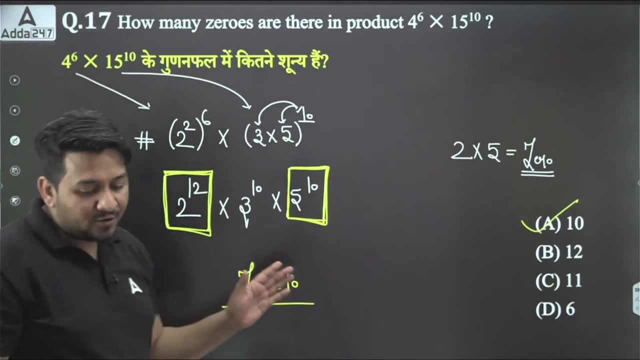 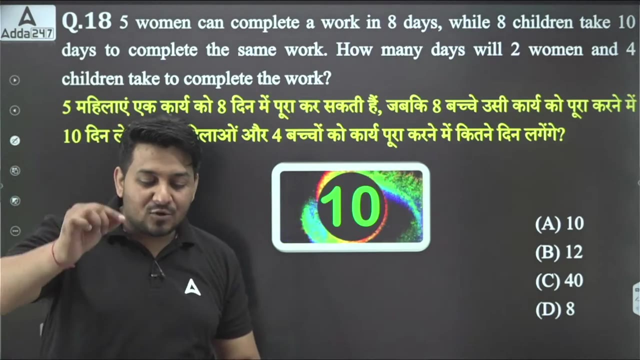 Will be zero. Say clear. All the kids once like and share and say yes, sir, clear, Proper clear, Proper clear. Quickly say yes, sir, clear, Very good. next, Next question: I will tell you: Man, woman based One question will remain. 100% will remain in your exam: Man, woman based one question. 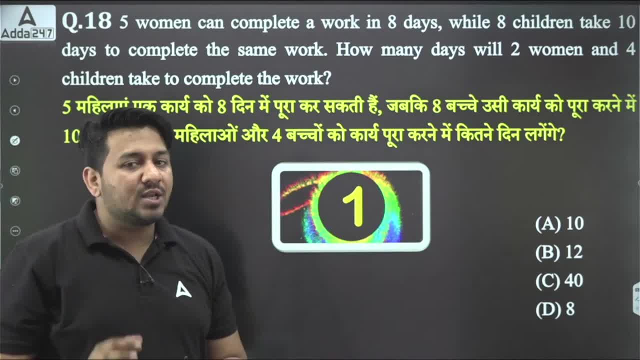 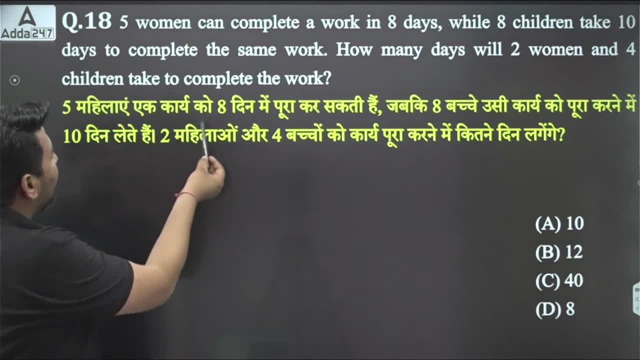 Man and woman's son. One question will remain in your exam. Read the question carefully, Do it. What is the question saying 5 women can do one work in 8 days, 8 children. Take 10 days to complete the work. 2 days: 2 women and 4 children. 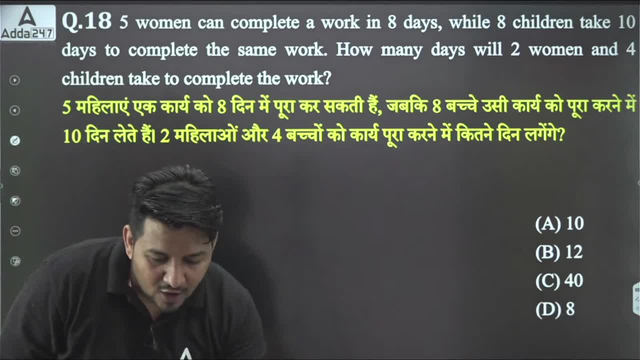 How many days will they do this work? All the children, tell me what will be the answer to this question. See how they will do. See. You know that if I put 5 women at work, Then the work is done in 8 days. Look ahead, If I put 8 children at work. 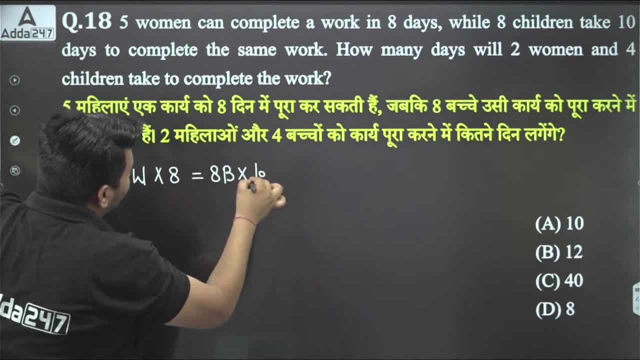 Then the work is done in 10 days. Tell me if it happens or not. Cancel. These 8 are canceled by this. 5 equals 5 5 times 10. That means 1 woman is equal to 2 boys. That means How much is the efficiency ratio of a woman and a boy? 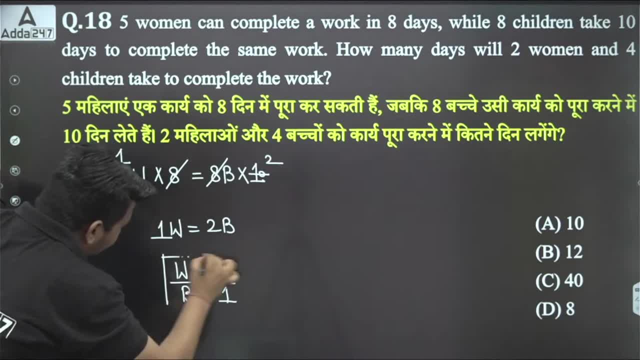 2 is equal to 1. That means Woman will do 2 work in a day. Boy will do 1 work in a day. Woman will do 2 work in a day. Boy will do 1 work in a day. Tell me clearly: How will you find the time? 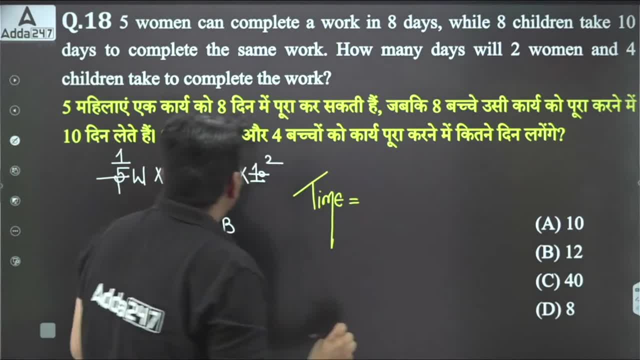 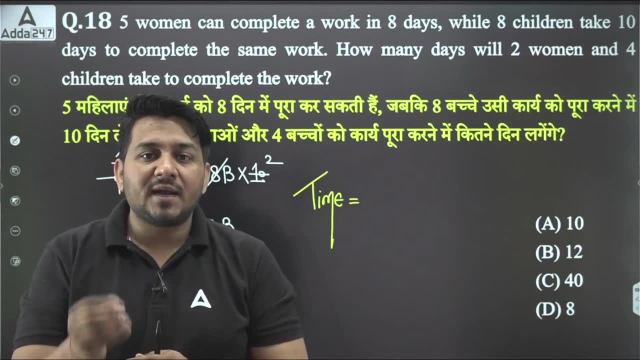 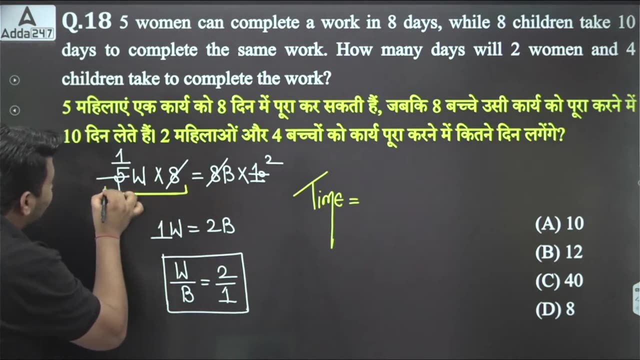 How will you find the time? See, We will find the time. First, tell me how much is the total work. If you find the total work, Time will come out immediately. See So to find the total work. If you want, you can pick this. You know that 5 women are doing the work in 8 days. 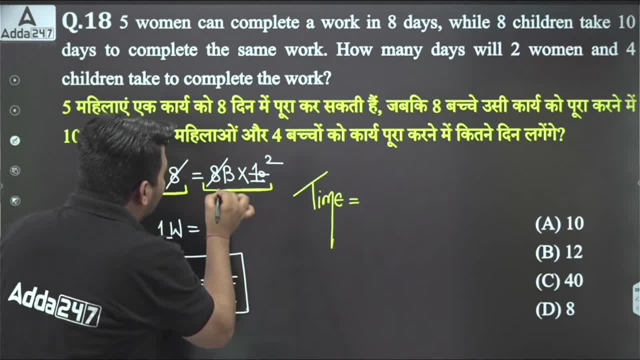 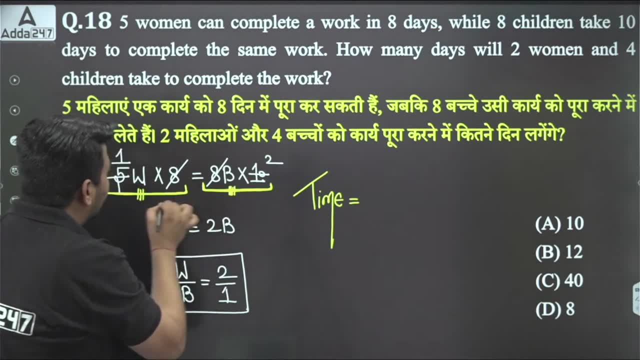 And if you want to find the total work, You can pick this: 8 boys are doing the work in 10 days. So if you want, you can find the total work from here. If you want, you can find the total work from here, From where you feel appropriate. 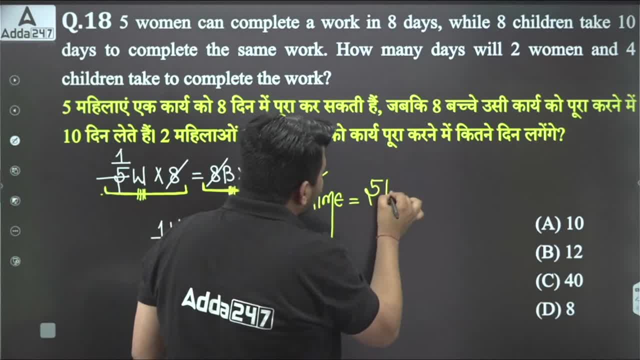 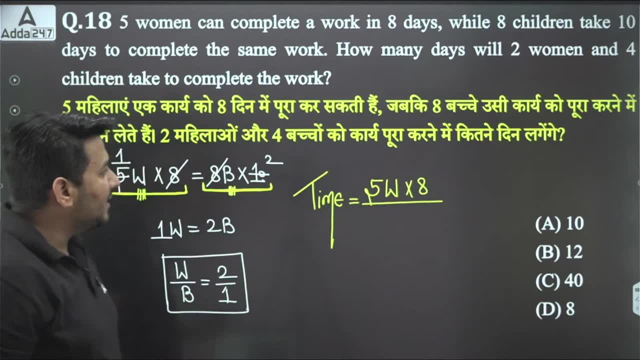 You know, 8 women Do the work in 10 days, Do the work in 8 days. See: 5 women are doing the work in 8 days. How many people have been asked? 2 women and 4 children. That means 2 women and 4 boys. 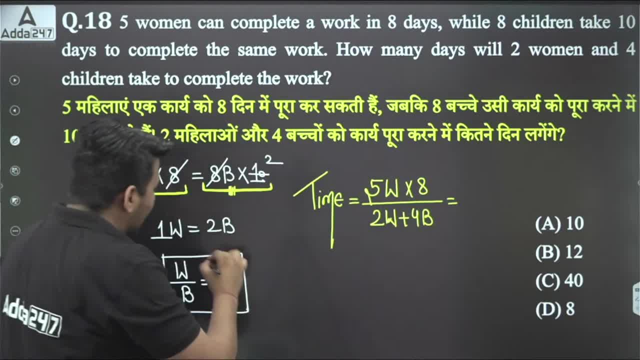 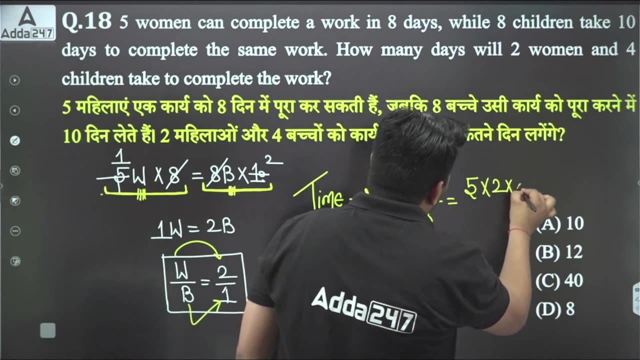 How long will they work Now? where there is W, There are 2 And where there is B, Put 1 there. Where there is W, There are 2. Where there is B, Put 1 there Quickly. Do it quickly 5 times, 2 times 8. 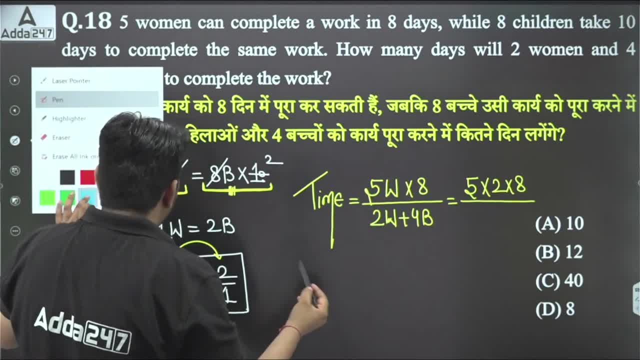 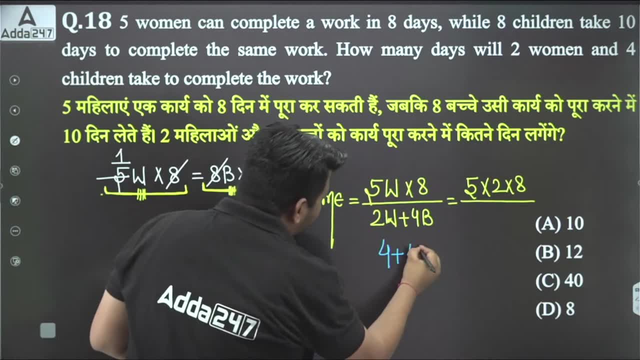 This is done. Now put it here Quickly. See here: 2. Keep W equal to 2, 2 times 2, 4. Keep B equal to 1. 4 is less 4, 4 and 4 together, How much is it 8? 8 is done. 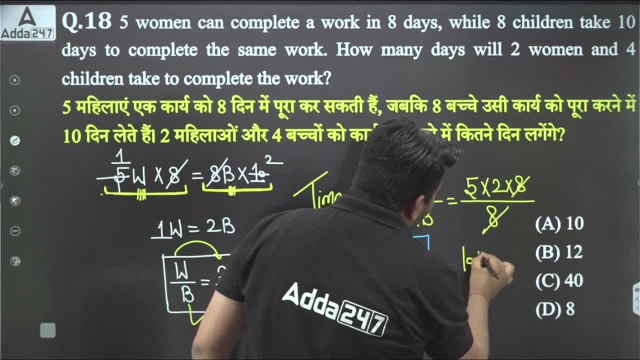 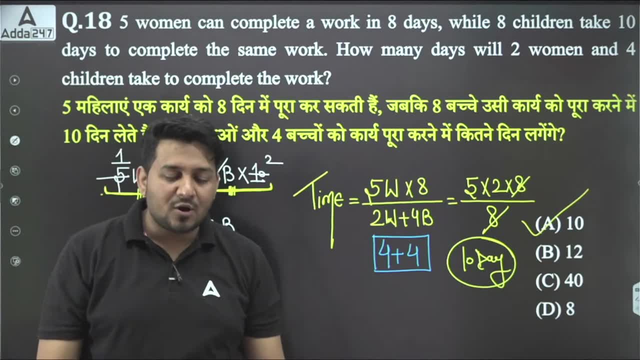 Cancel this here. How long will it take? 10 days, 10 days. What is 10 days? Correct? answer Option number A: What is 10 days, 10 days? What is 10 days? Correct? answer Option number A: Thank you, friends. Tell me quickly. 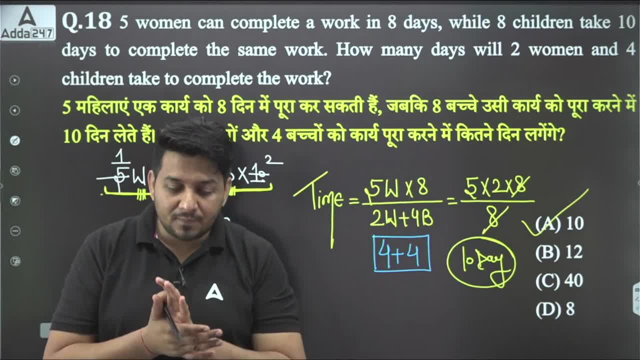 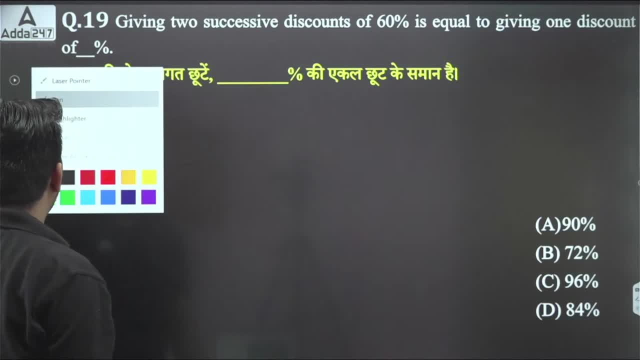 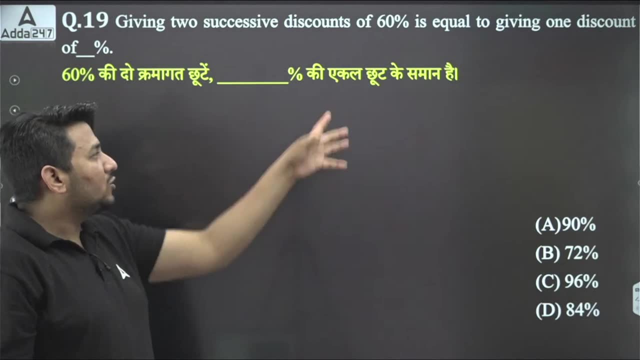 Yes, sir, clear, You are doing very well. You are doing very, very well. Next question. Next question: 60%, 2 times less than 1. You all know This question will come in your exam: 60%, 2 times less than 1. See how to do. 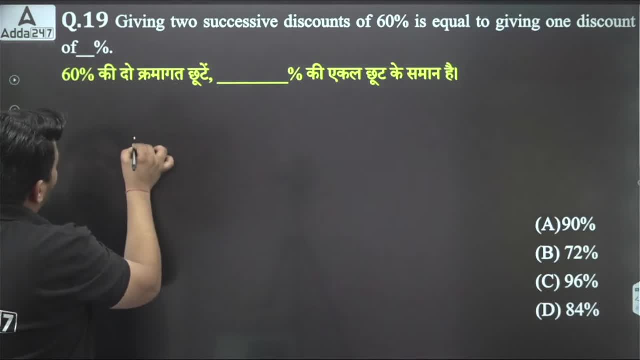 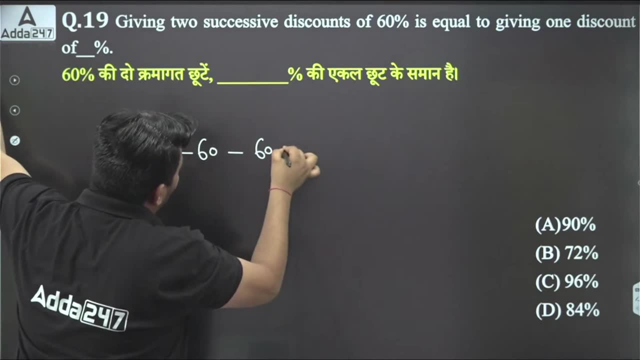 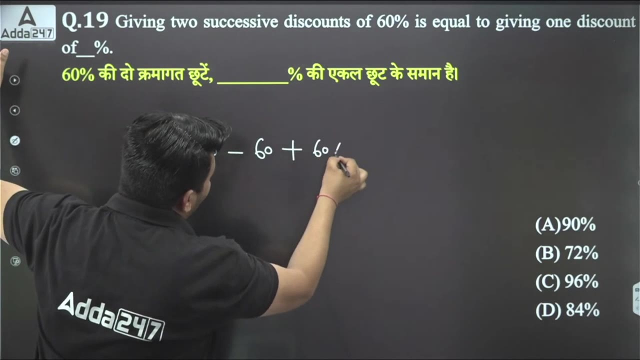 The easiest way I am telling you: See, First 60% discount was given to you, Then 60% discount was given, Then both multiply. You know, When you multiply minus and minus Plus 60 times 60 Divided by 200, A plus B, AB upon 100. concept. 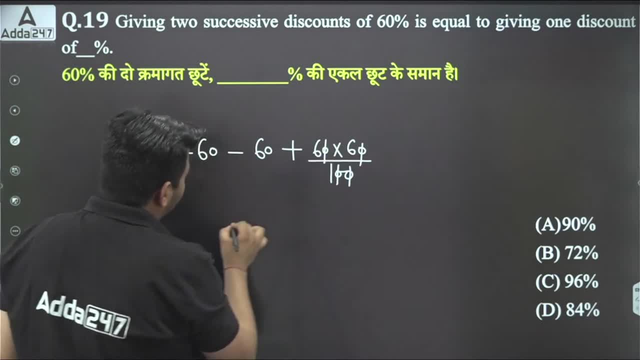 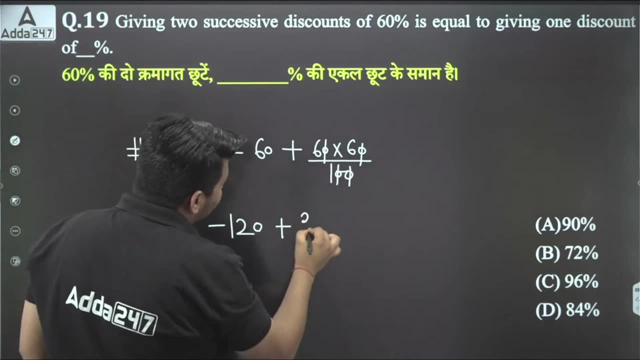 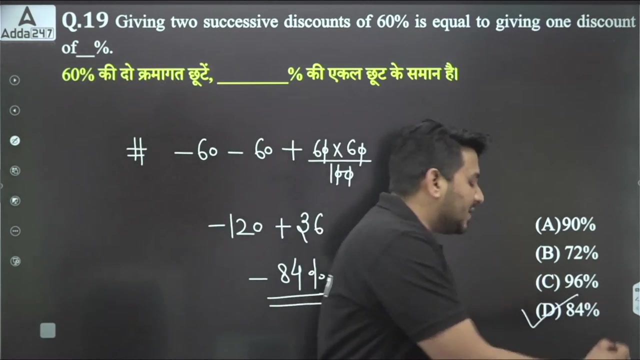 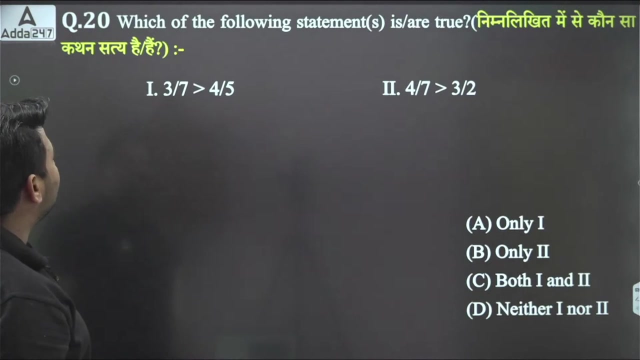 Simple. This is canceled by this. This is canceled by this: Minus 120 Minus 60, Minus 60. Minus 120, Minus 630 Minus 60. How will you find out which is the truth and which is the lie? Which is the truth and which is the lie. 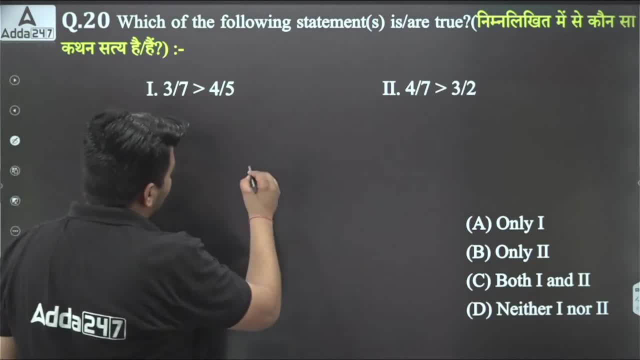 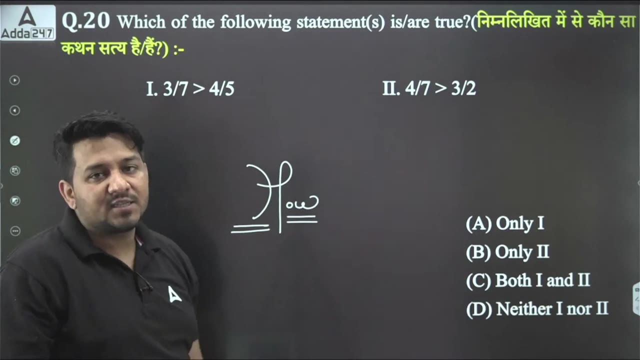 You have to find out. Let's do one thing. I am giving this question in the homework. You all do it. I am giving this question. Do it in the homework, Don't leave it. Don't leave it. Everyone's answer is required in the comment box. I will discuss it tomorrow. 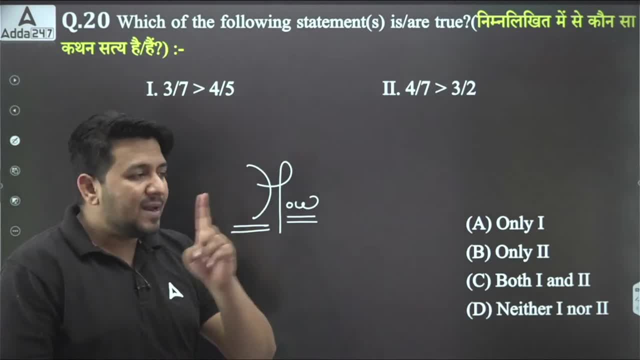 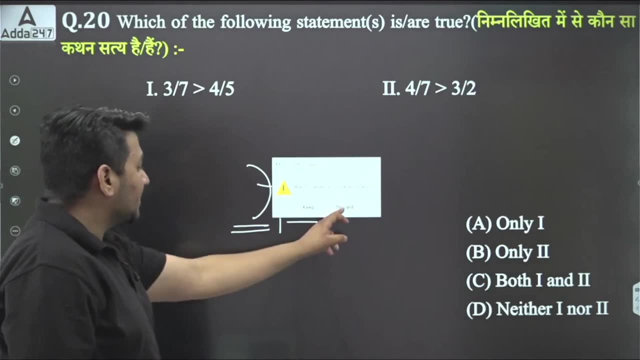 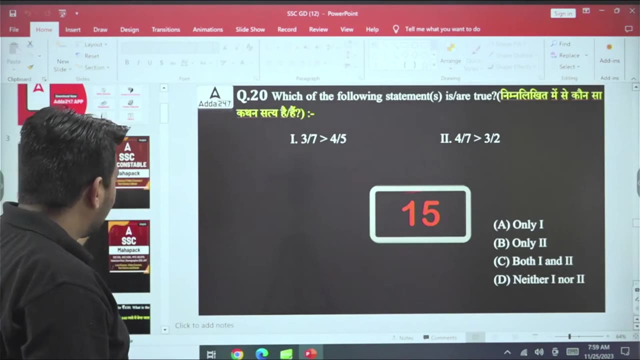 Before going. The number of vacancies has come. Don't worry, The number of vacancies will increase. The number of vacancies will increase. Now look very carefully. All the people who are preparing- I am giving you all a chance To fulfill your dreams- All the people who are preparing, All the children, do one thing: 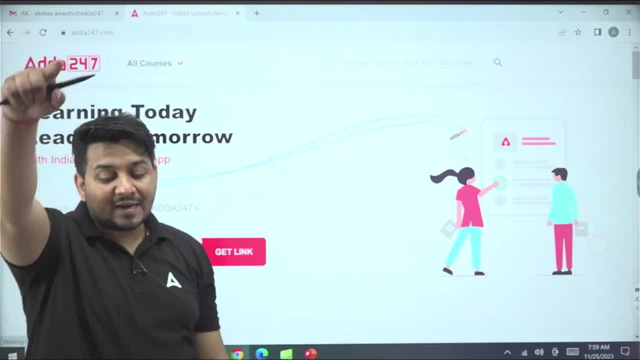 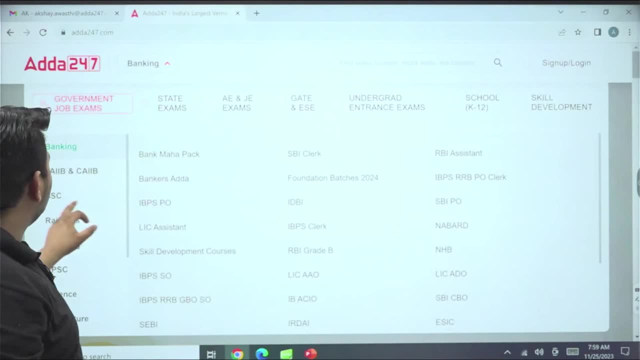 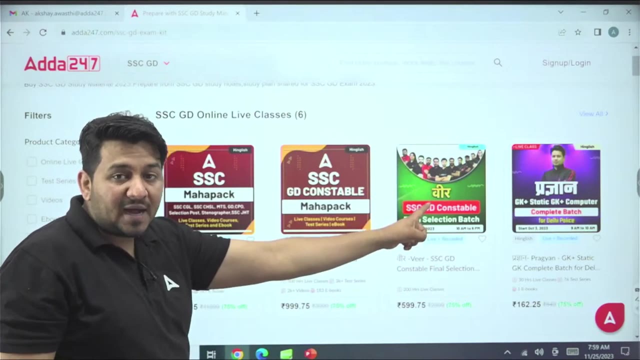 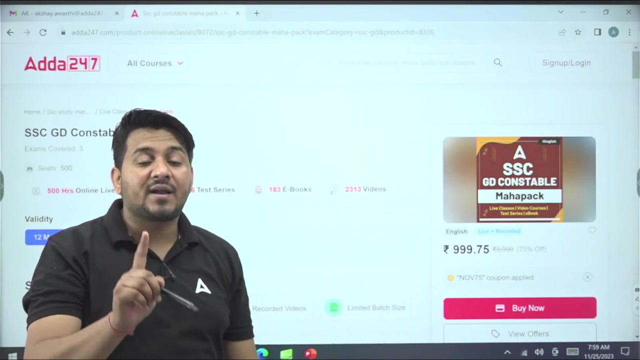 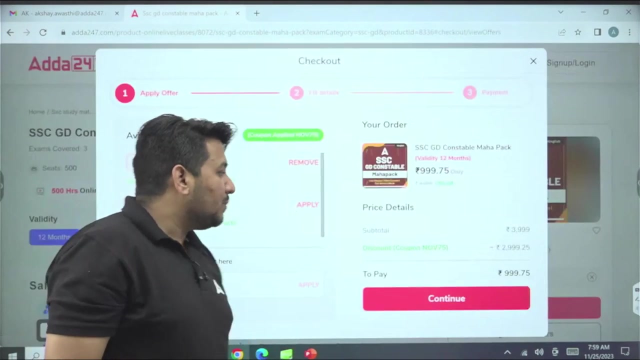 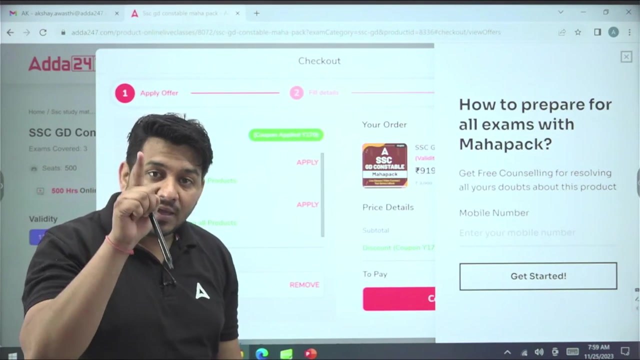 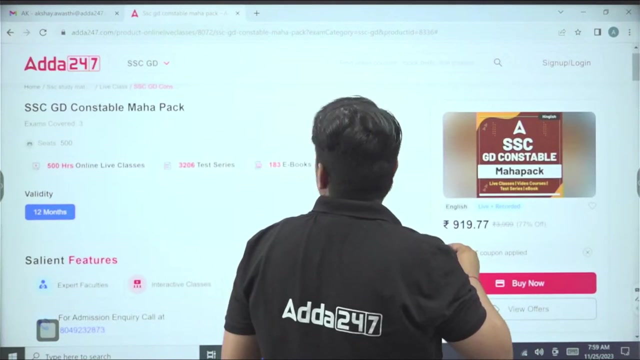 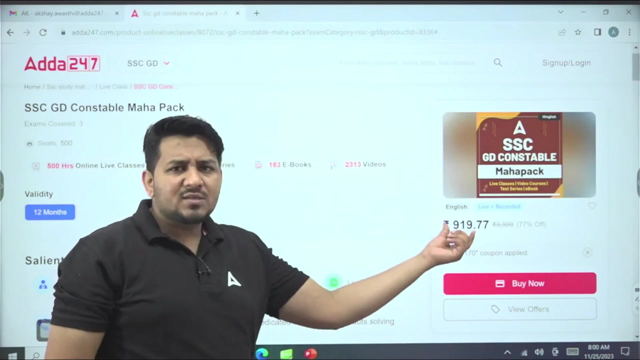 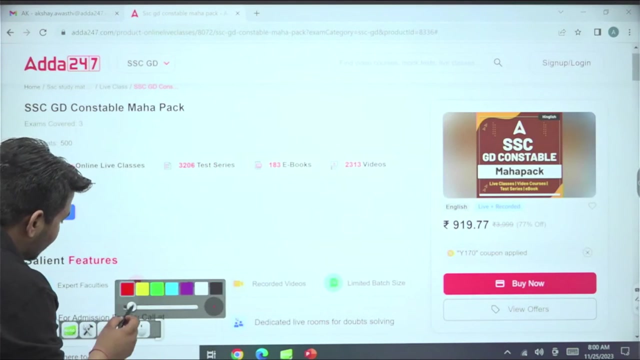 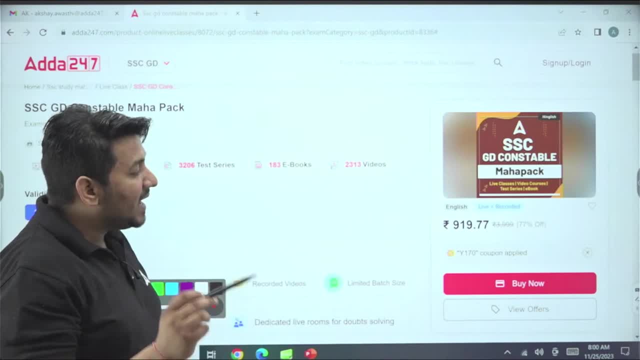 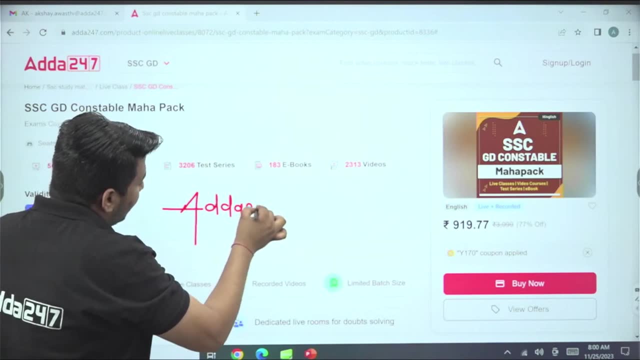 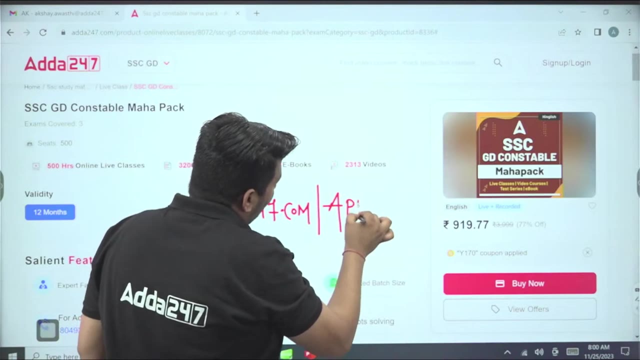 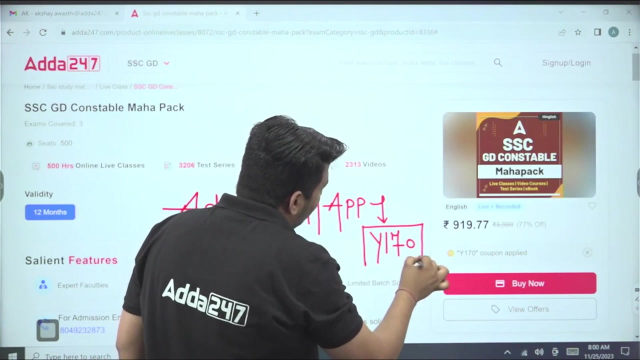 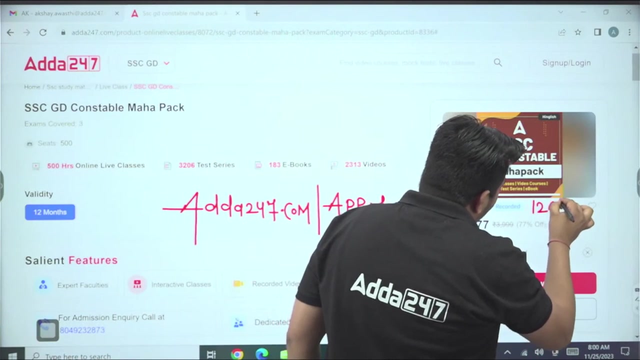 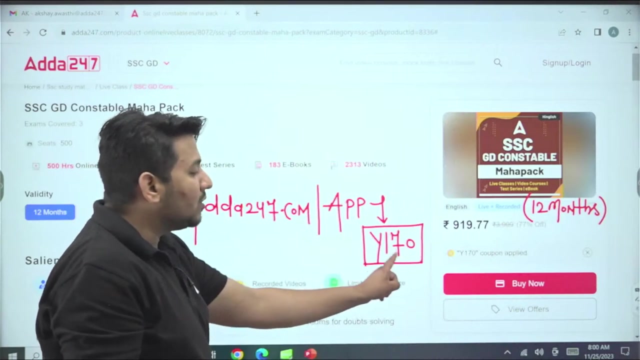 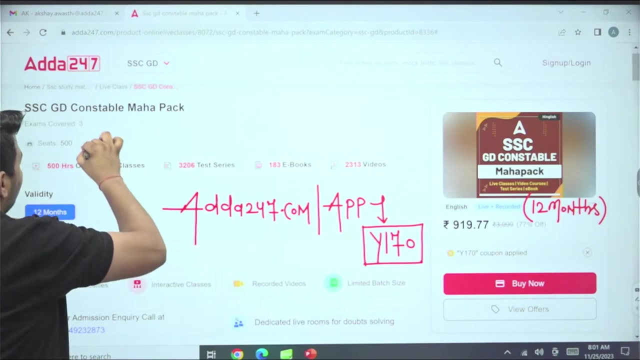 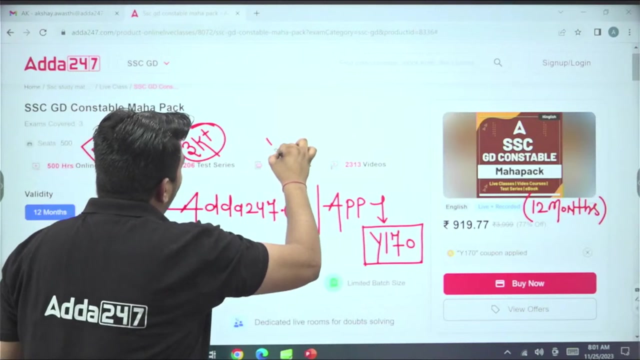 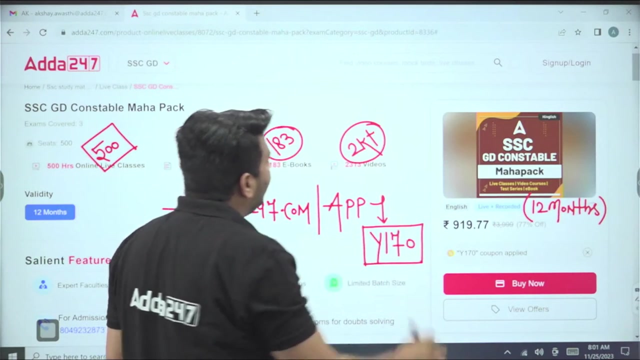 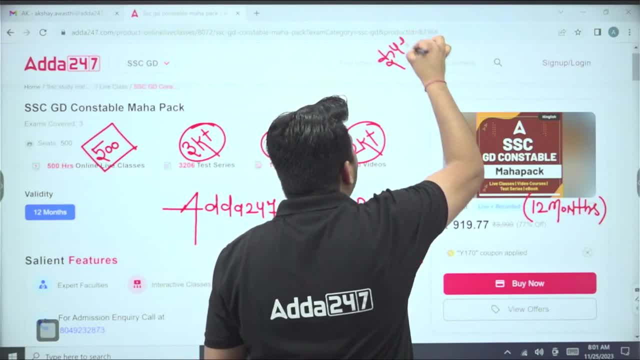 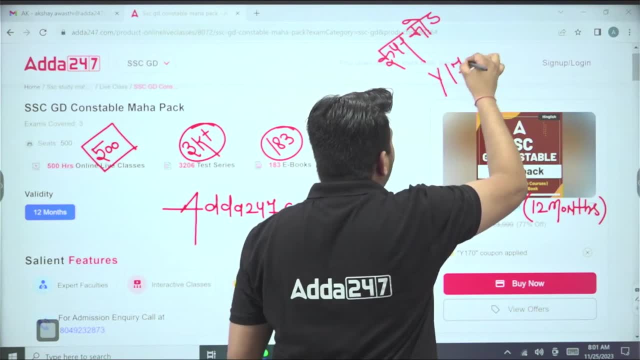 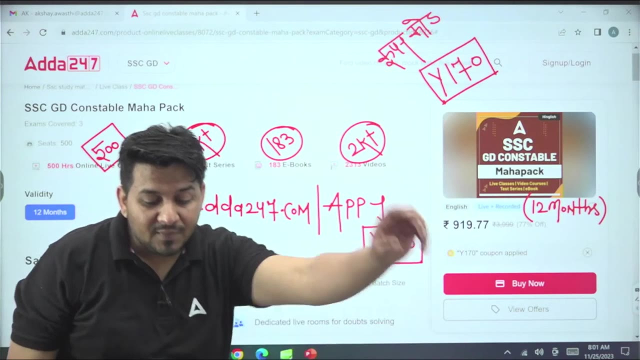 But remember, don't use the wrong coupon code. What will be your coupon code? Your coupon code will be Y170.. For discount, you have to use the coupon code Y170.. Don't use the wrong coupon code, Otherwise you will be worried later that. 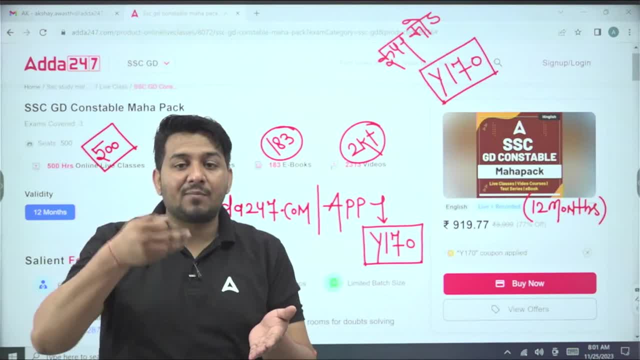 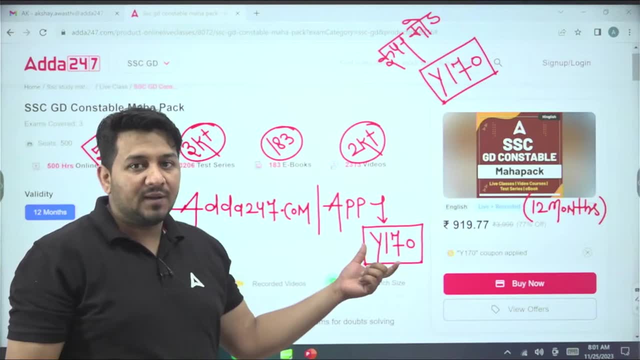 Sir, we got this thing and we didn't get this thing, Then I may not be able to help you at that time. So quickly, use the Y170 code and join. It is my full responsibility of maths. Okay, Let's go. 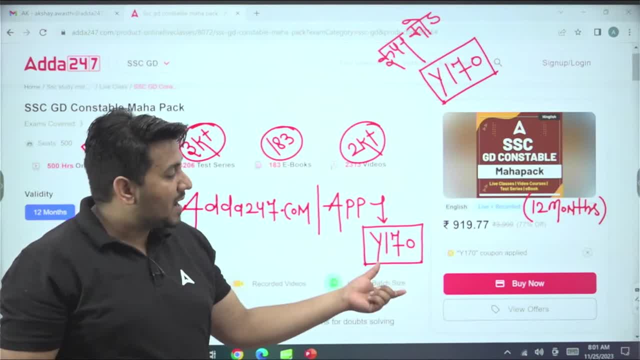 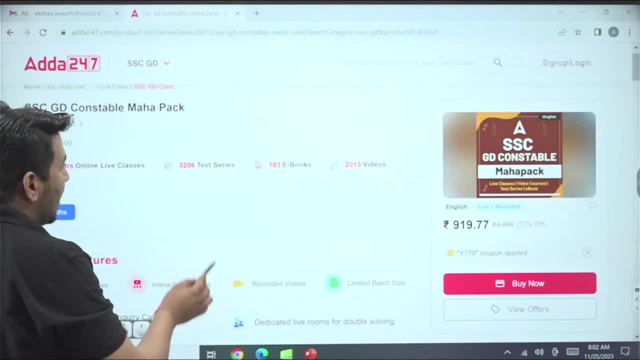 Write in the comment. write to the people who want to join this Mahapack in the comment. Quickly, Okay And friends, a small information. If you are preparing for GD, then you can join GD Mahapack, But along with that, kids. 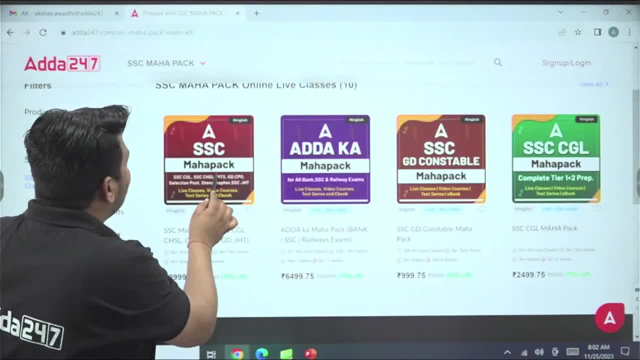 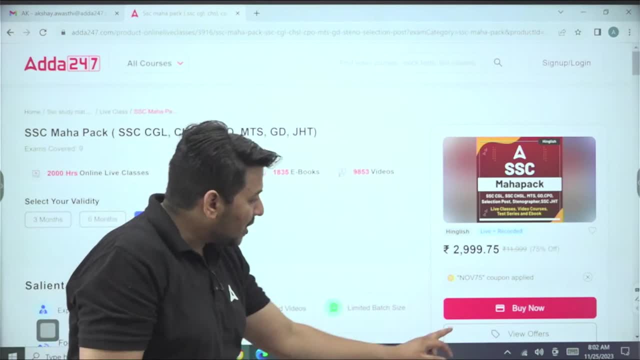 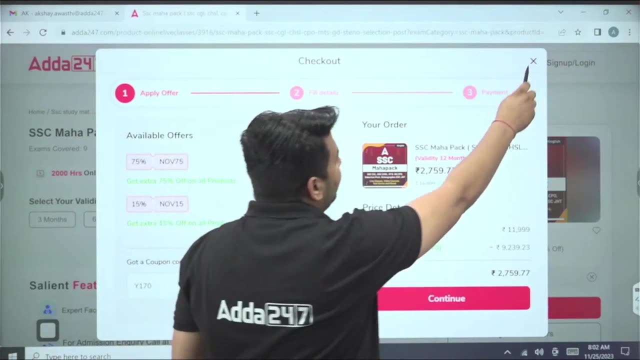 If you are, If you want to cover all the SSC exams together, In which your GD, CGL, CHSL, MTS are all covered, Then you go to our SSC Mahapack. It has the code Y170.. It will be yours in Rs 2759. 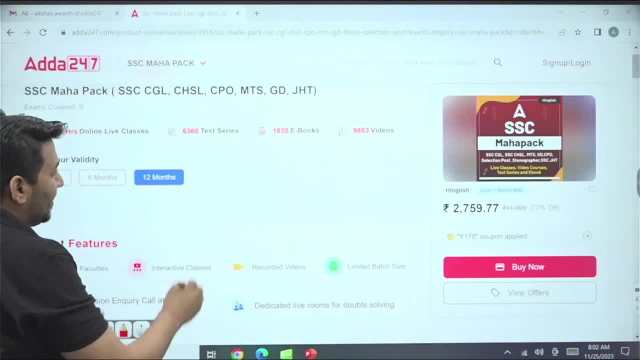 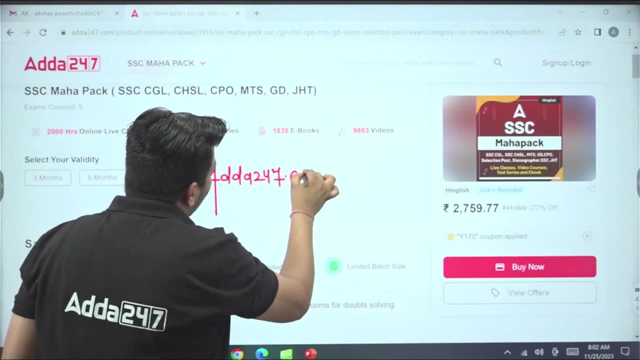 All the SSC exams are covered in it. No SSC exam is left. What is the process of joining Kids? it is the same. You can visit adda24x7.com or the Adda app. Visit adda24x7.com or the Adda app and go to the code Y170 and get enrolled in it. 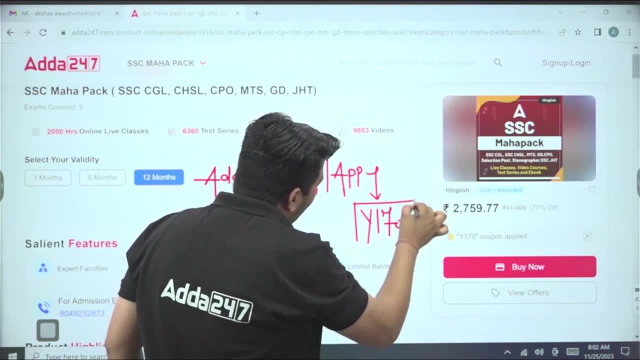 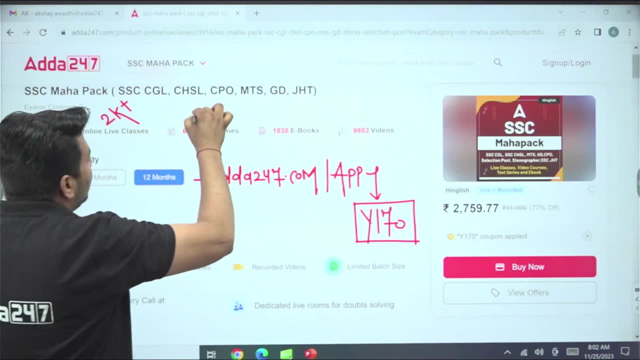 Okay, In Y170.. Okay, This coupon code is covered in all the SSC exams. Here kids have 2000 plus hours of live classes, 6000 plus test series with detailed solution, 1800 plus kids have e-book. 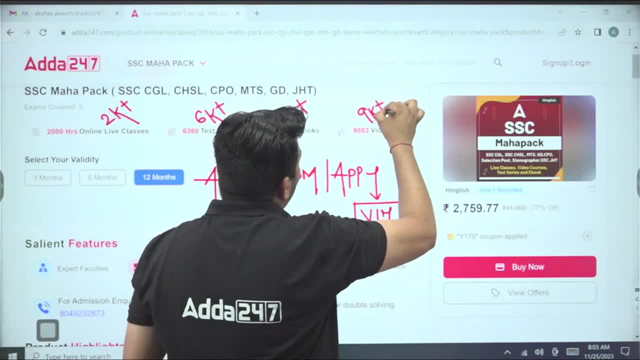 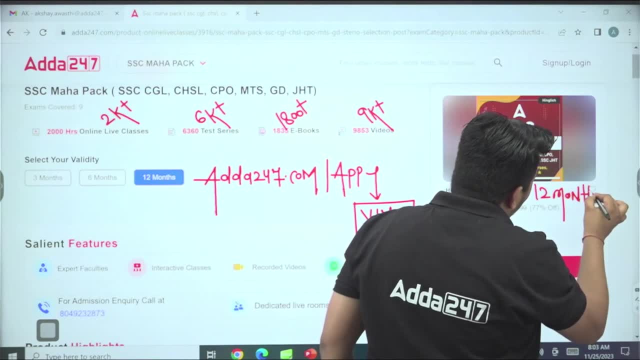 And 9000 plus kids. What is this? Video courses. This much content is there. Validity is of 12 months. Tier 1, Tier 2 is fully covered. Okay, All the things. we will guide you here, But remember you have to enter the coupon code Y1702.. 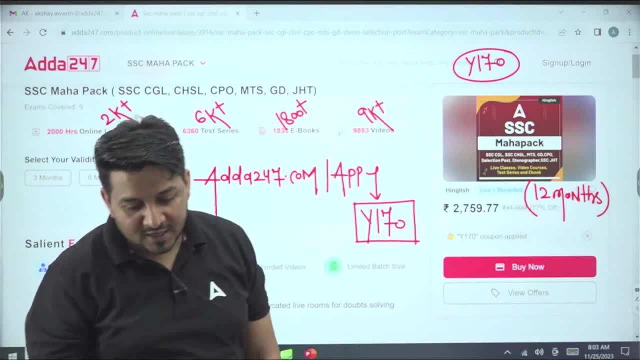 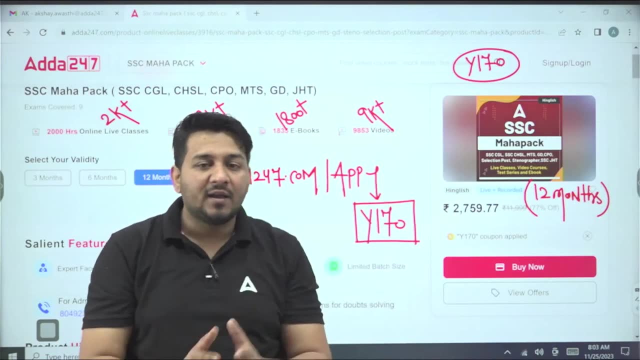 Take the benefit of this. Connect with us And confirm your selection. Okay, kids, So all the people who have not joined: Look, if you are preparing for GD, then you can take GD Mahapack, But if you want to cover all SSC exams with GD, 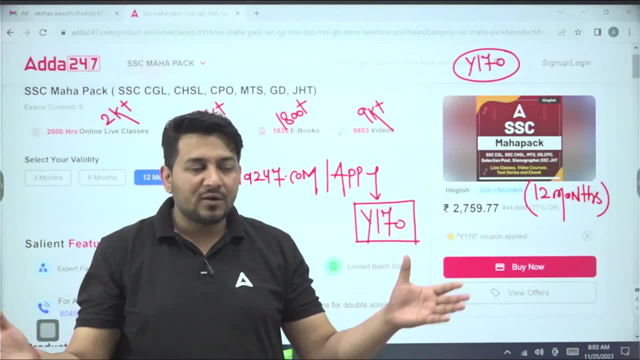 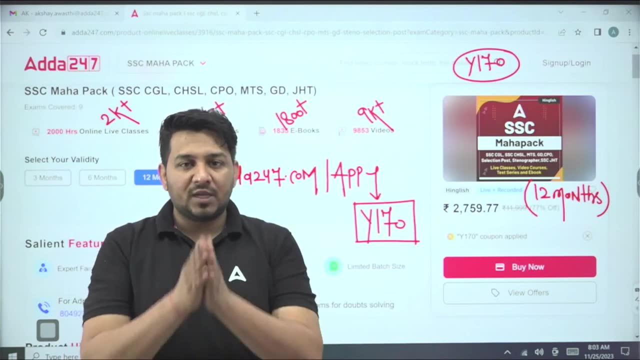 Then you can go to SSC exam In GD Mahapack. Use coupon code Y1702.. Connect with us And confirm your selection. So, friends, Till here for today. Till then, good bye, Jai Hind, Keep studying. 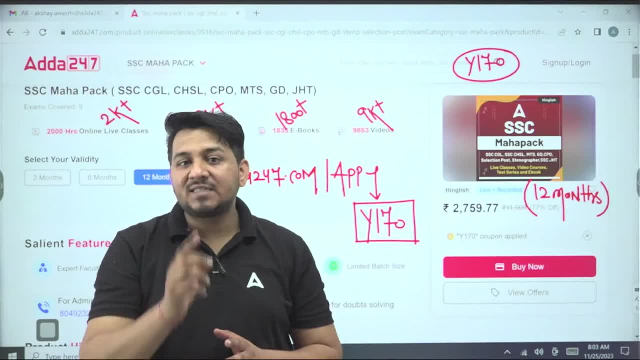 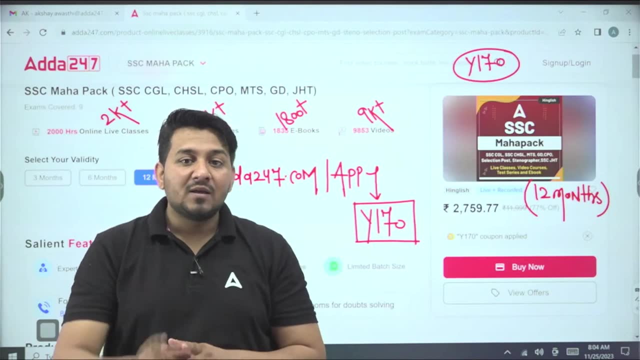 Stay safe. And one thing, Before all the kids go, write in the comments: How was the class Plus? You have to connect with me daily at 7 am Morning, at 7 am. You have to connect with me in this special class of daily math.